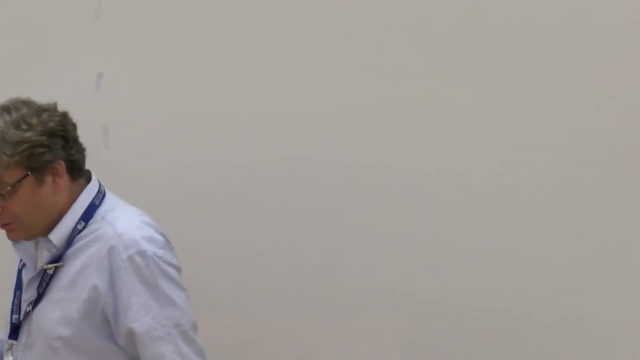 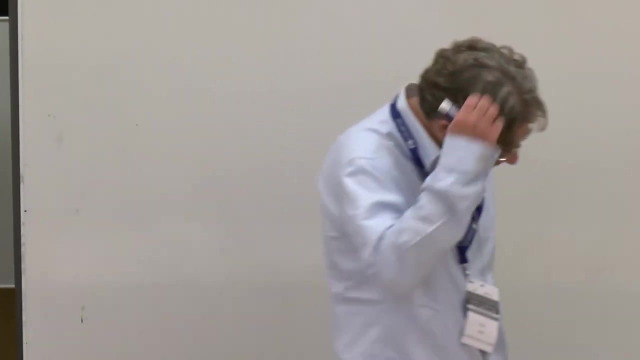 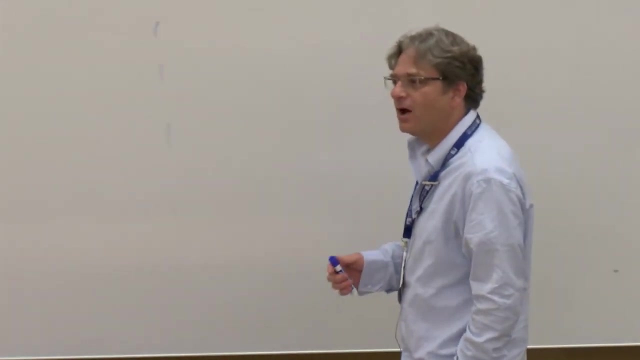 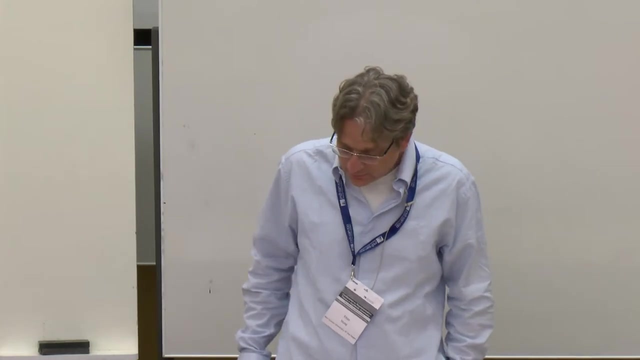 and I will try to illustrate the ideas and somehow the motivation for us to study the problem. The basic thing is motivated by classical problems of counting lattice points in various compact sets in homogeneous spaces, and this is a very classical subject. Maybe I will formulate: 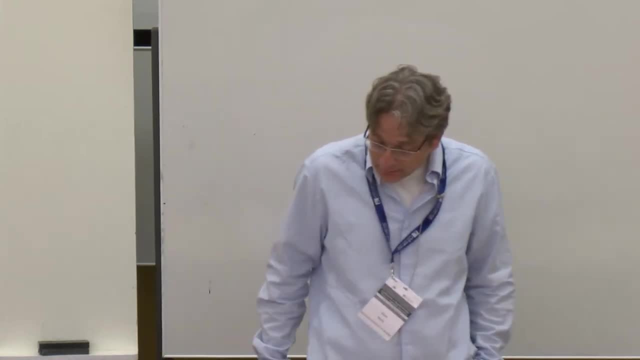 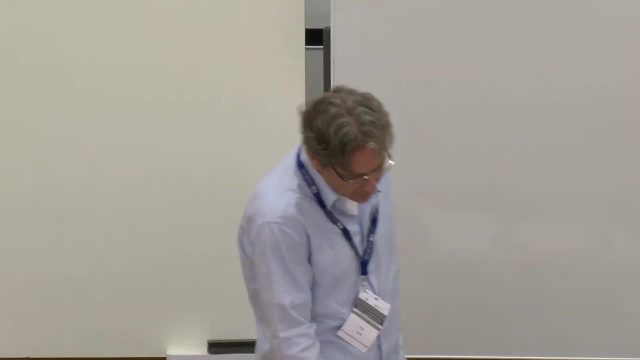 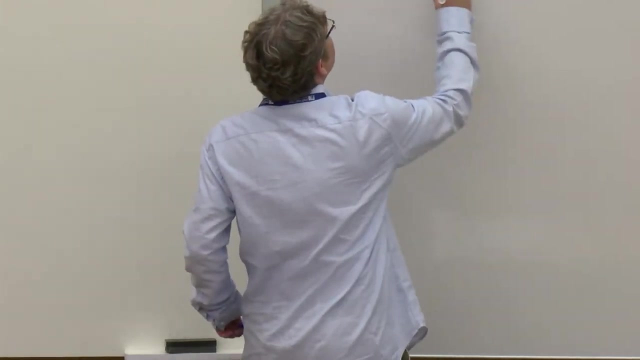 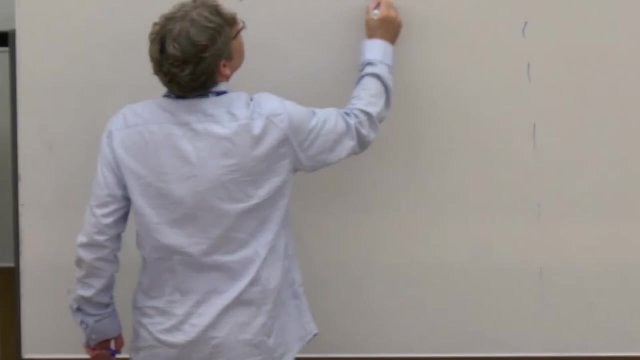 the setup and then introduce some of the ideas which played a role in our study. This is a report on a joint work with Bernard Krutz and Henrik Schlittgur, who was giving a course here. Bernard is going to come next week. 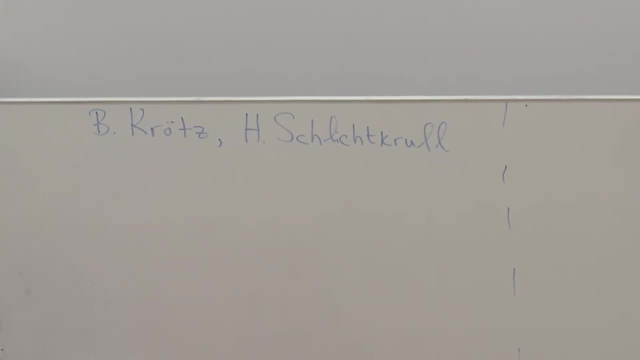 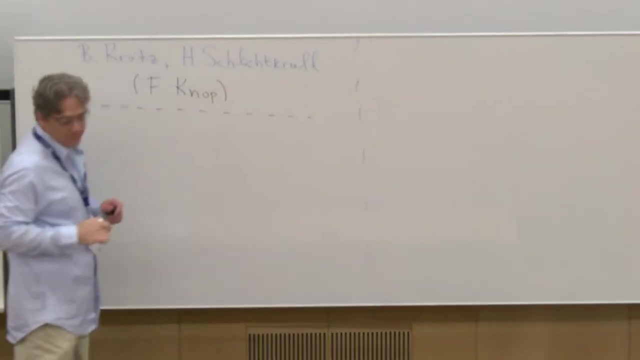 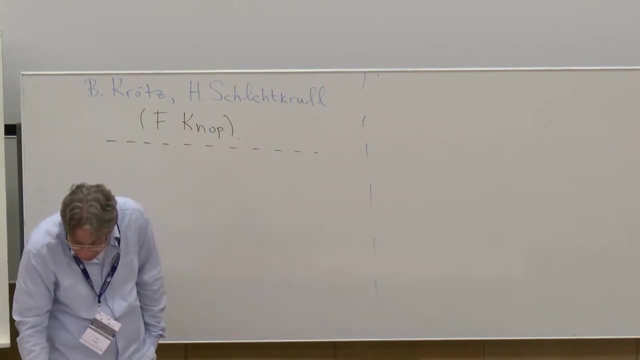 Is this visible? Okay, And parts of this project were also joined with Friedrich Noll, The paper itself I'm going to report on. Friedrich is not the co-author, but it was a series of works. So what is the setup? Let me start with. 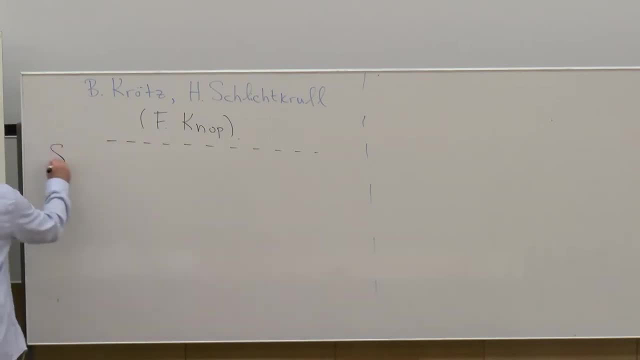 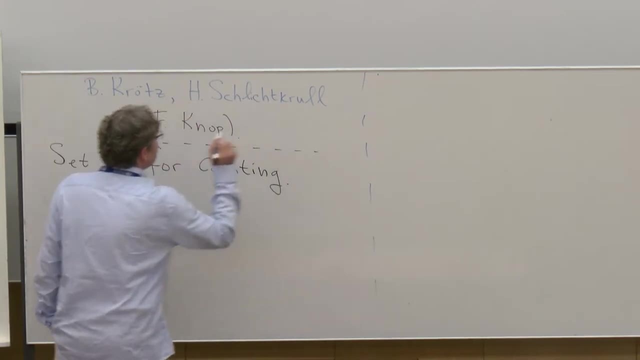 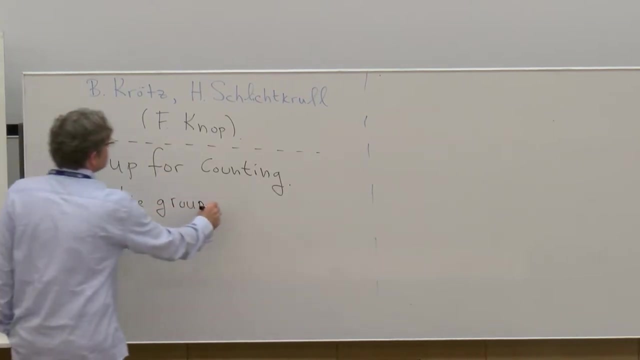 a set up for counting. What do we want to count? So in principle we think about G, which is some kind of a Lie group and a space where G acts, And for simplicity we assume that the action is transitive. So usually smart people work with a group acting on. 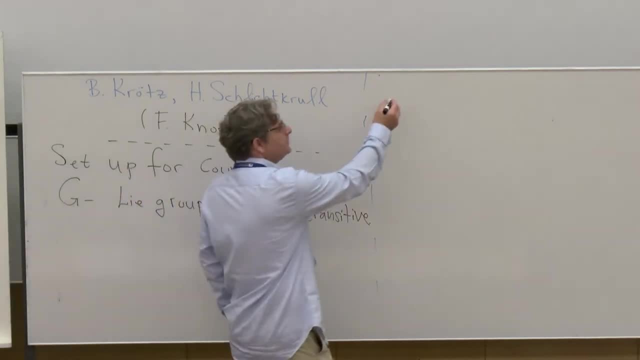 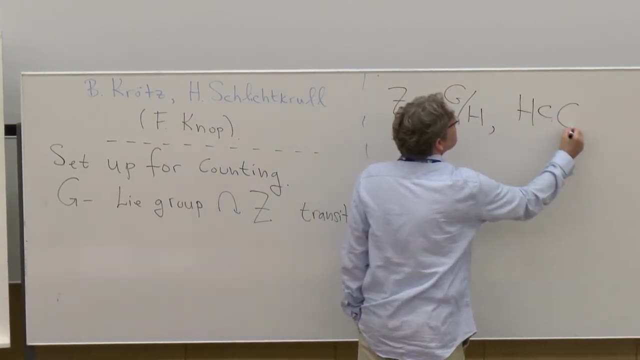 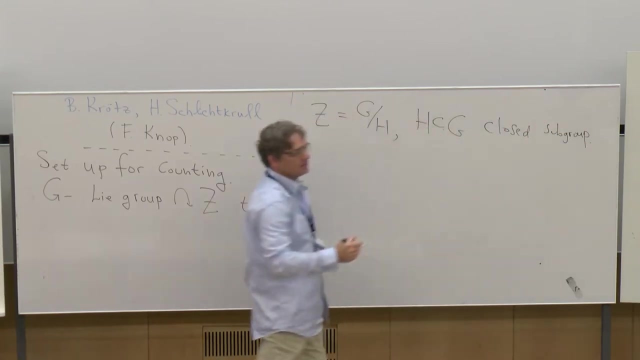 a space More pedestrian people would, in a transitive case, would write: Z is a G more H, where H is some closed subgroup. But this is the general setup and our aim is to count points in Z. So what does it mean to count points in Z? We will have a balance. 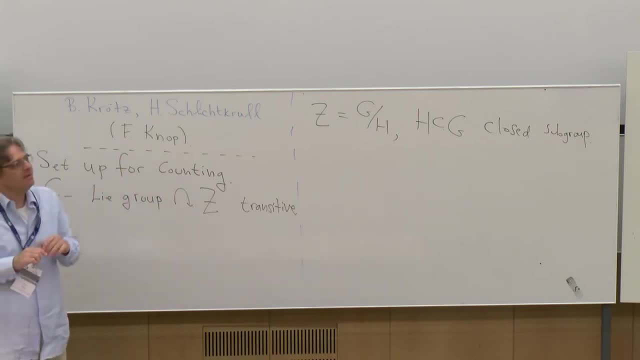 between a countable object which is manifested by a lattice in G, So D in Z is going to be a countable diamonds, Okay, so if you want some kind of things you want to collect, So a typical setup for that would be. 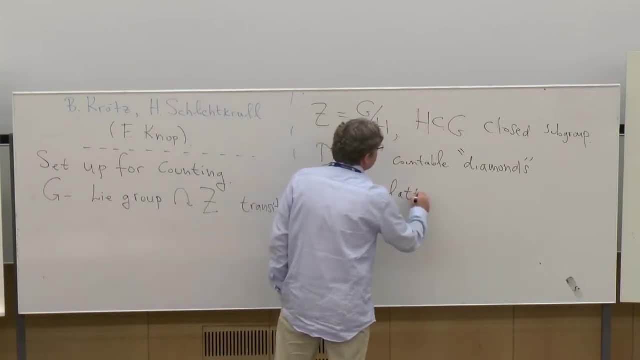 gamma in G is a lattice, a discrete subgroup, and D is going to be a countable diamond. Okay, so if you want some kind of things you want to collect, so a typical setup for that would be: gamma in G is a lattice, a discrete subgroup, and D. 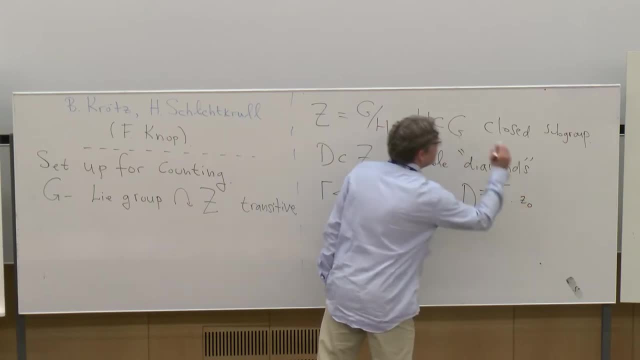 is going to be a countable diamond. Okay, so if you want some kind of things you want to collect, so a typical setup for that would be: you say, the orbit of one point in Z. Z, nought for me represents the class of H or the identity element in G. Find G gives me a particular base point in Z. 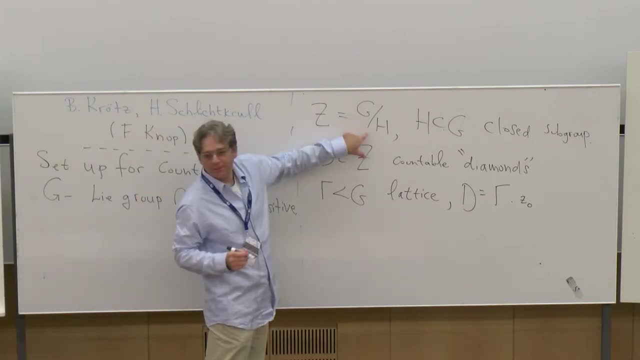 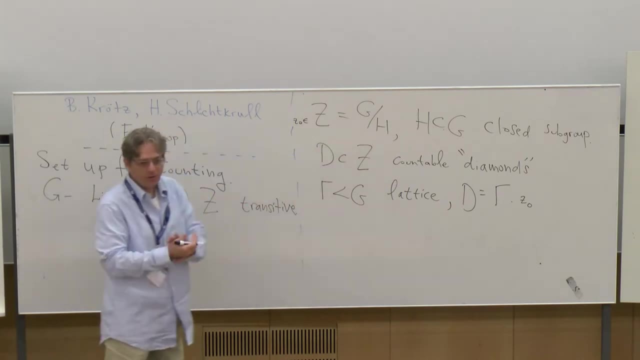 Is that okay? So this is the diamond I want to collect, but then of course, there are infinite, So I need some compact sets in which these diamonds are organized. So I need aIse. don't know if it's visible here. 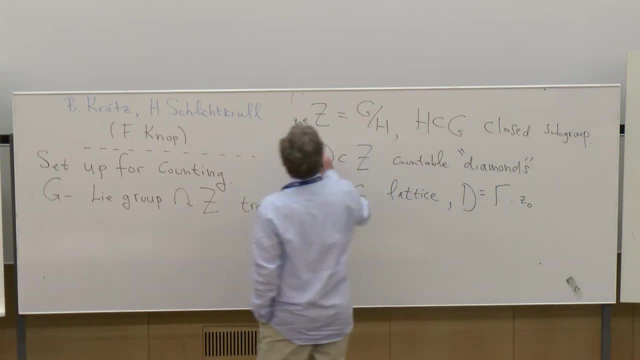 I'll try it here. It's visible, So in this setup it's visible to you. Eris doesn't pay attention anyway, but let's see. So we have this countable set, and the third item in this scenario is a collection which I parameterize by some real positive number. 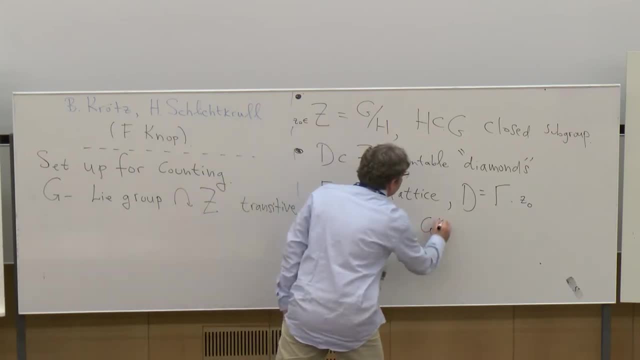 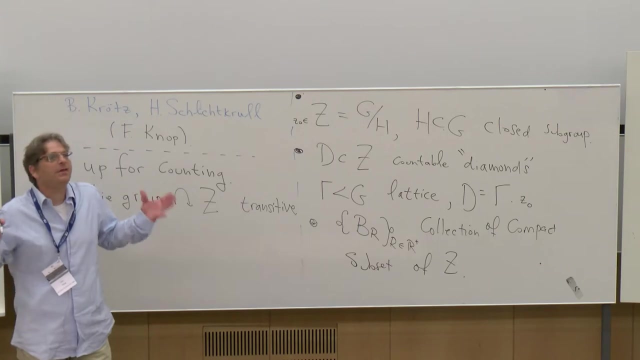 So we have a collection of compact subsets of Z. Okay, So for convenience, I mean, you can think about the Euclidean space, and PR would be a ball of radius R centered at the origin, and gamma would be so okay, 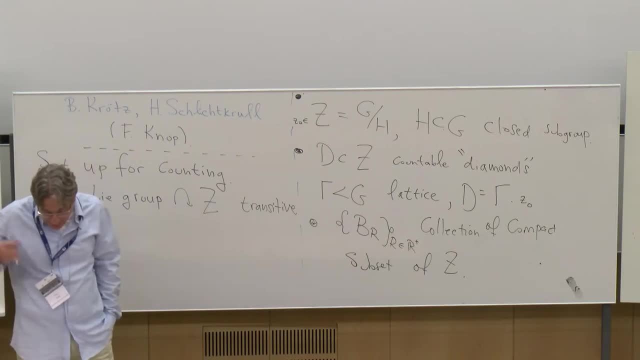 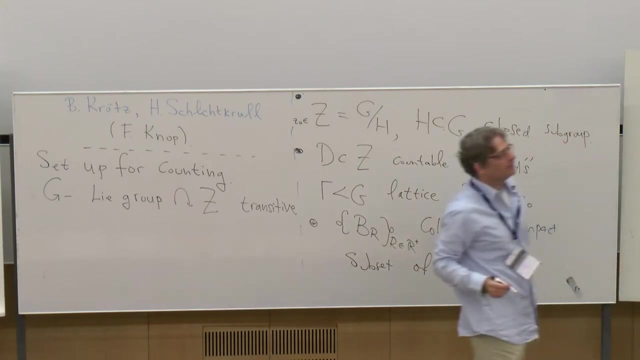 In such a setup, the set we are interested in. so we want to count the size of the intersection of V with this BR or gamma acting on Z, naught intersection of VR. So these are the numbers, Okay, So these are the numbers we are interested in. 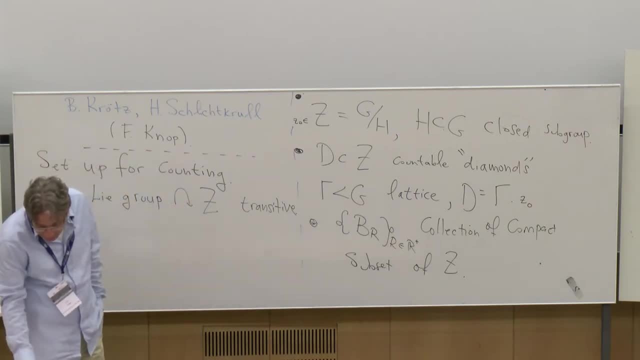 Okay, I don't know if this is visible, So maybe I will. So you're assuming it's a discrete set? Let me, Yeah, the D is discrete set. yes, So I don't really know whether this is which parts are visible and whether I'm writing too big. 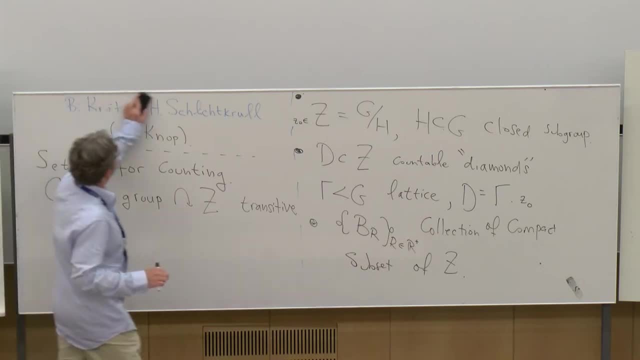 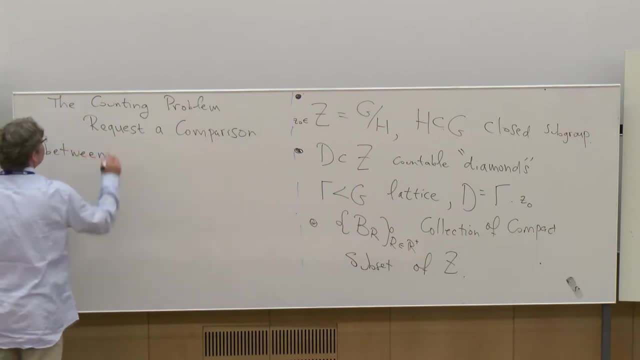 Let's call it arithmetic quantity, which I will denote N sub R. So this N sub R is formally the size of the set of elements gamma in R. Okay, So it's going to, and one more time. Okay, So one of the way I was due to visiting my parents to see this. That's a much smaller number. You have to measure it earlier this week. 질문 gamma H. I'm going to prove it Studying. Okay, You have started at Mach- overheating Students are cute, So we are going to write number 11 and that is or or. we are going to take into account. 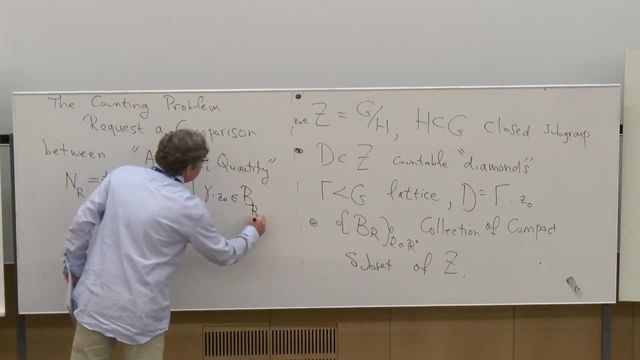 sum over there. So you have given be that the cell N is equal to, And so you have given that gamma. And now, So this is So. that's the plus information here, right? The second septal ogram here. Now what we are going to do is we have two numbers. 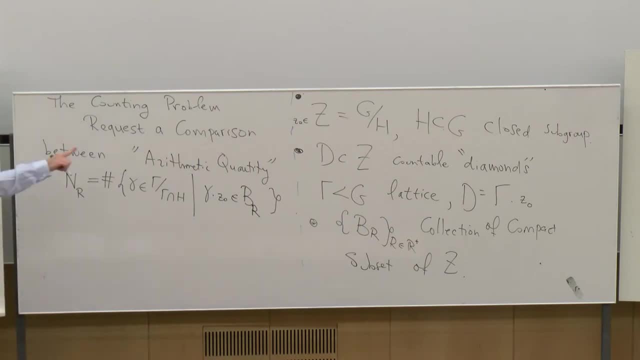 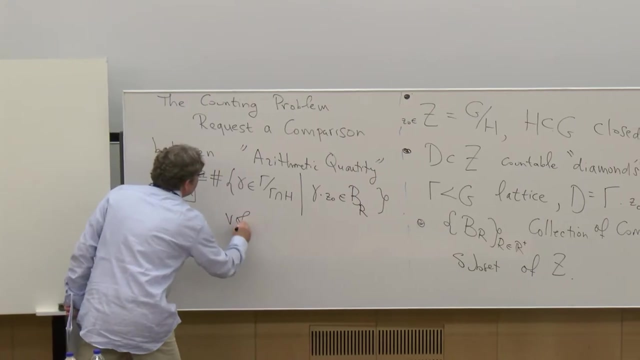 One is eight. Do you see the Rector? So it's a simple exercise to see that the number I was mentioning over there is given by this formula. Okay, So this is the number of diamonds, Okay, And the volume of the ball. 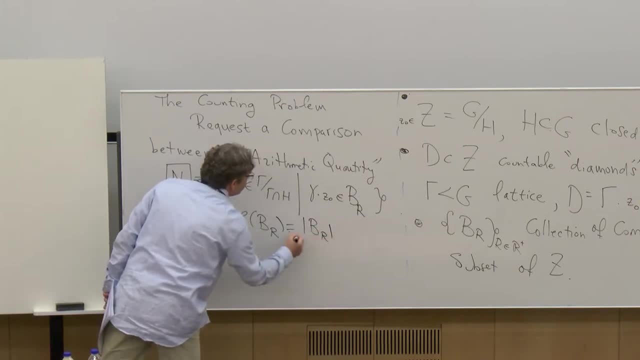 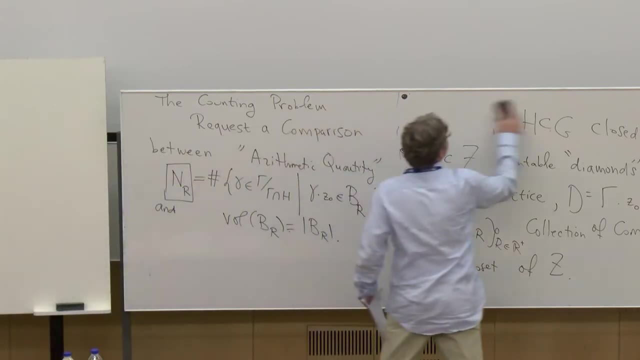 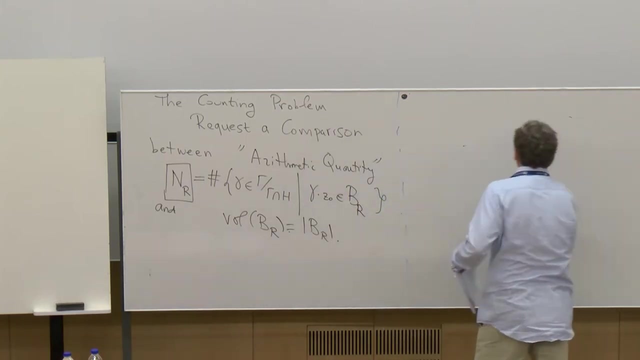 which I will denote by Br further on. Okay Now, these balls are not necessarily balls and they're just compact sets at the moment, And the comment which was made ensures that these sets, these compact sets, intersect, these discrete sets. find out the many elements. 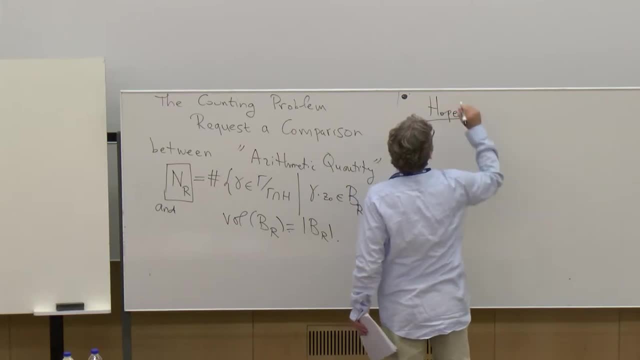 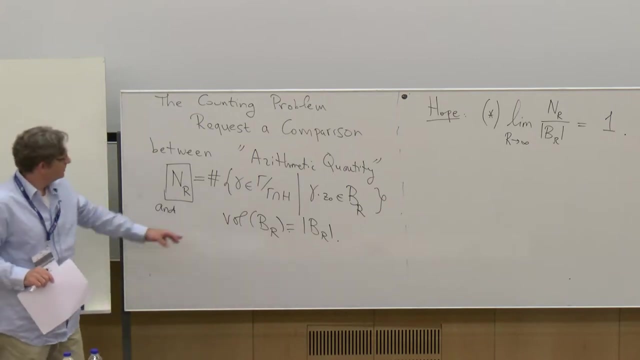 So the whole is that the limit of nR divided by Br, where R goes to infinity, exists and is equal to 1.. Okay, Nobody jumped volume with respect to what. Okay, we will put all these small iotas later, but it's kind of clear what's going on. 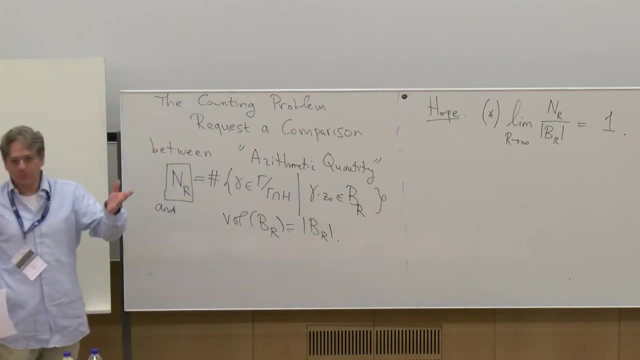 We have this group G and H, which were erased from the blackboard. We will assume that say they are reductive or semi-simple. So we have measures and the quotient space is unimodular. So we have a unique invariant measure and properly normalized. 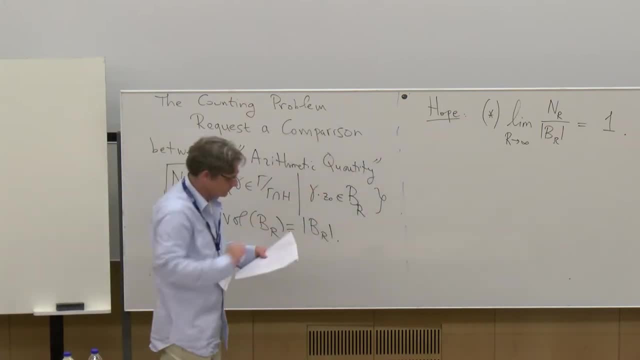 We want to get this, So we have this equal to 1.. Okay, So I'll put all the small things later. I just want to. So this is called: If this holds, we say counting holds. Okay, So we are very happy. 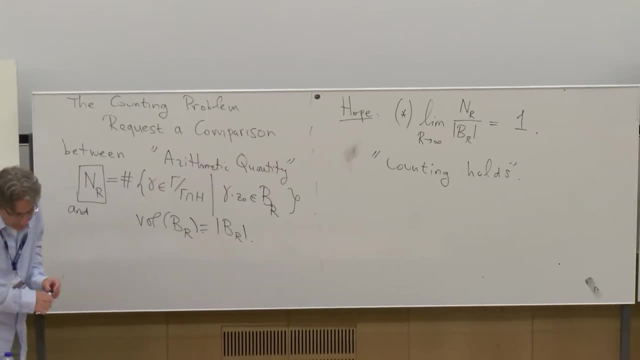 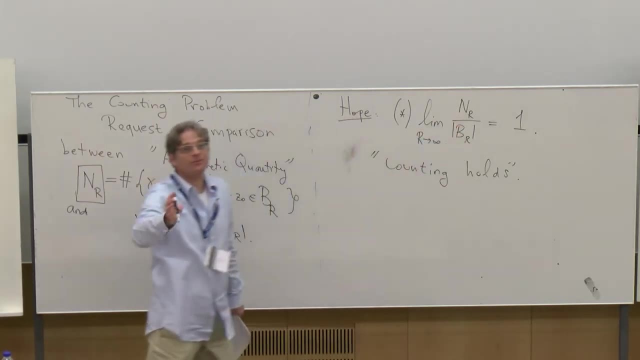 And we can ask for the further things. So this is called sometimes main term counting. So this means that the number of diamonds is approximately the volume of the set where you're looking at. And now you can, of course, ask Next. 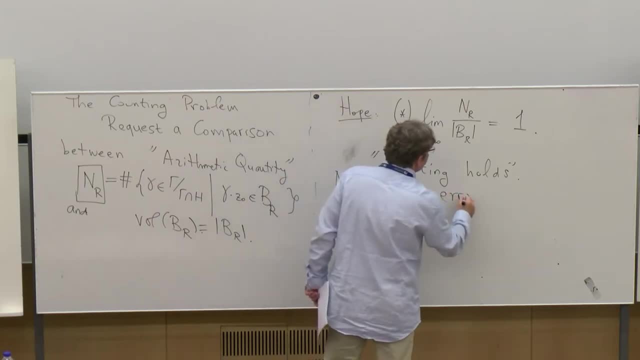 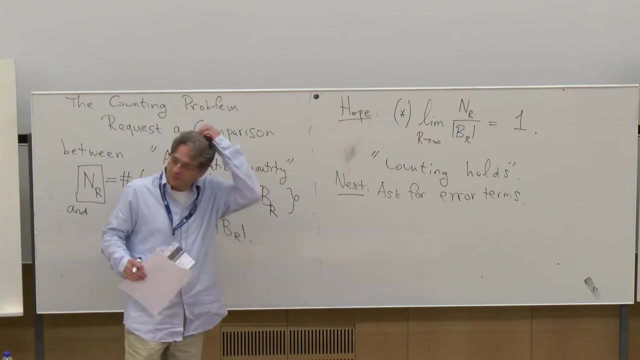 Ask for error terms. I will formulate the theorem. I will formulate the theorem saying that the hope is validated in this case. Okay, Just because you are impatient, if you take G to B, S-O-N-1 to the power 3,. 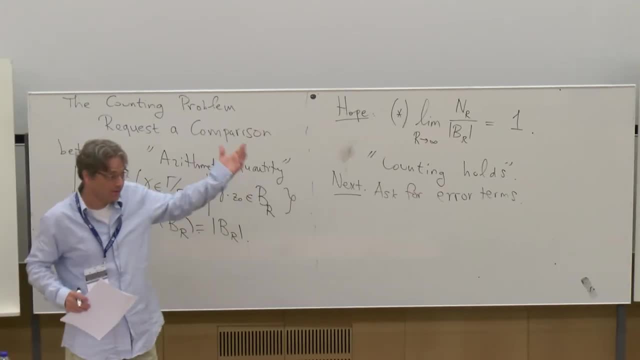 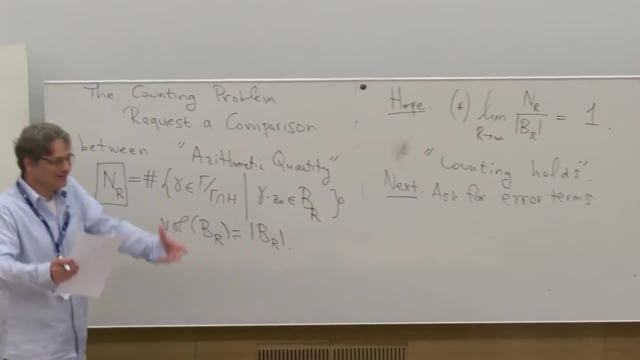 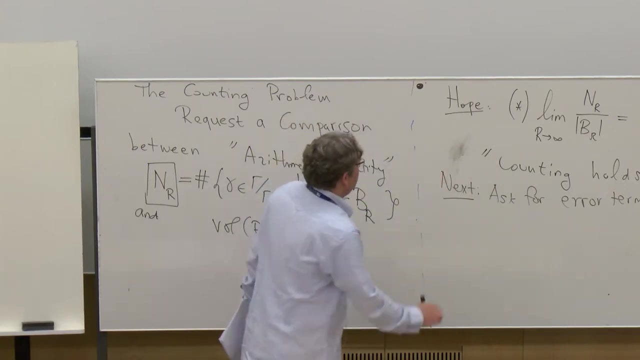 and H to be the diagonally embedded subgroup. then in this space, this kind of triple product space, this property will hold, for certain class of discrete subgroups, gamma. Okay, So we'll sort out the parameters later. Okay, so the natural thing to do is to look at the difference. 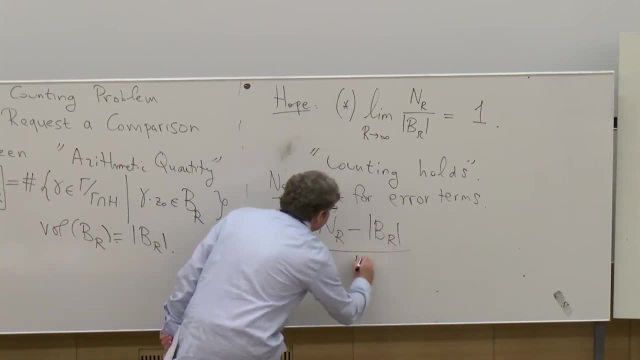 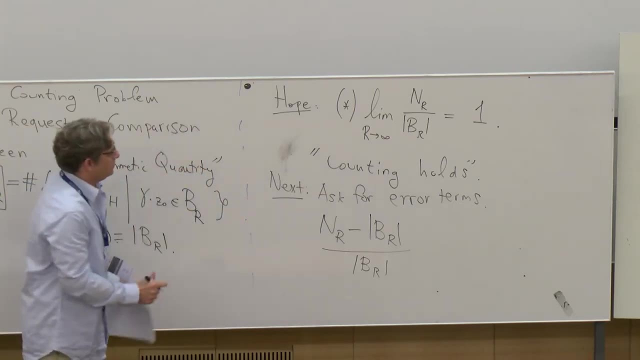 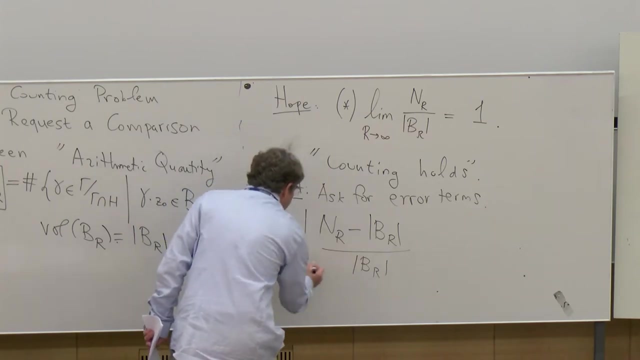 and properly normalized, would be probably to divide it by the volume. So what we are asking is to estimate this difference. So the next hope, which might be simplistic, is to get this number less than or equal to some constant times the volume to the power minus S. 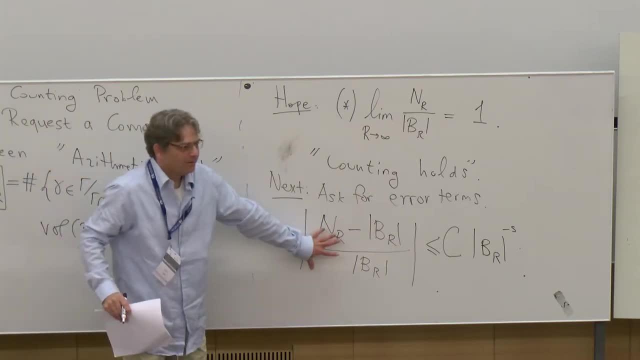 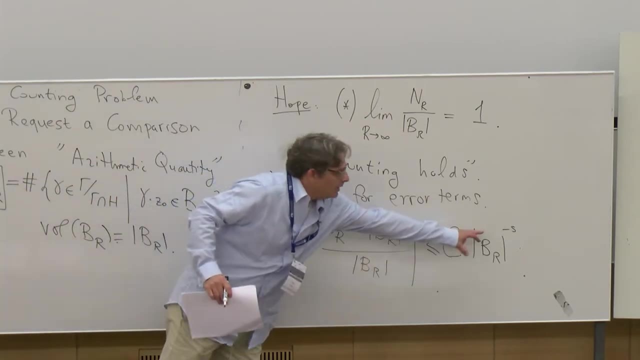 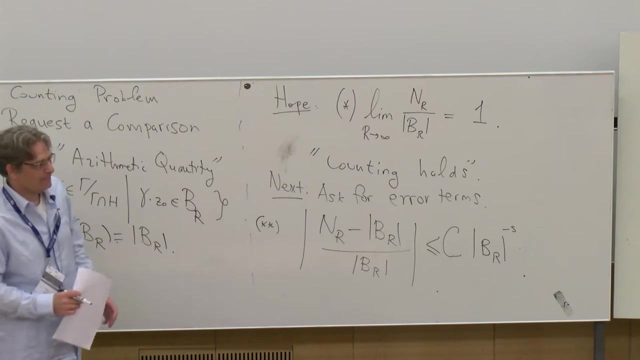 So there are so many letters here, The error decays to zero and the quantifier goes like that: There exists a positive constant C and a positive constant S, so that this inequality holds for every R. Okay, So there exists positive C and S. 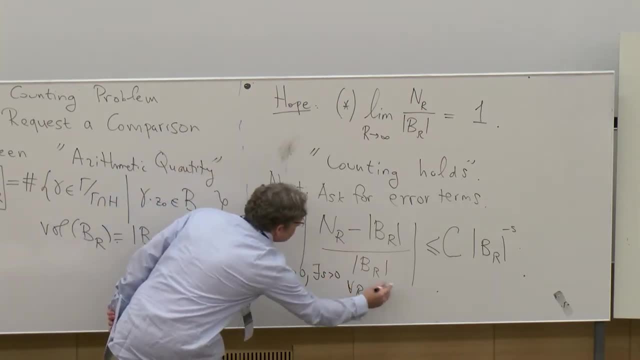 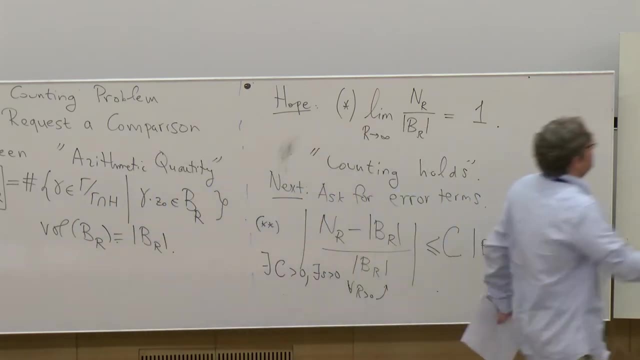 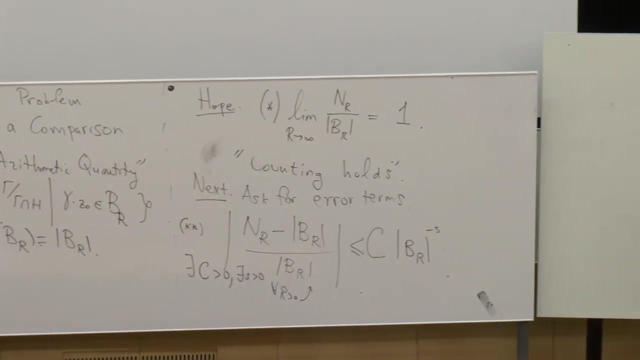 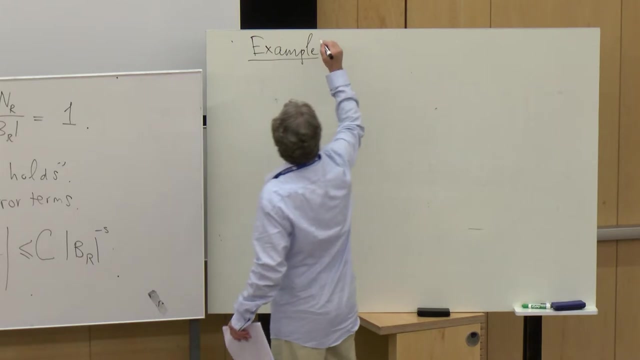 so that this holds for every R? Okay, So these are the kind of two questions one may ask. This is really a classical subject and it really goes back to Gauss. So the mother of this example- I mean I trust that 101% of my audience is familiar with this example- 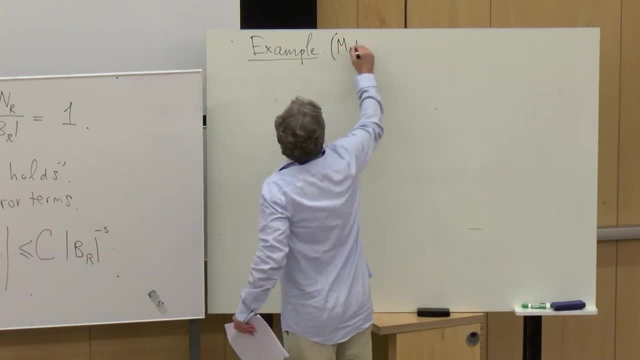 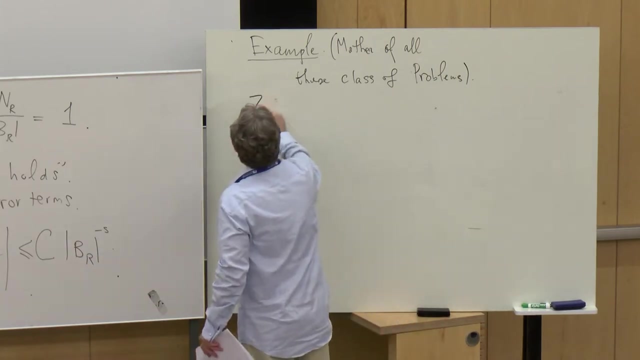 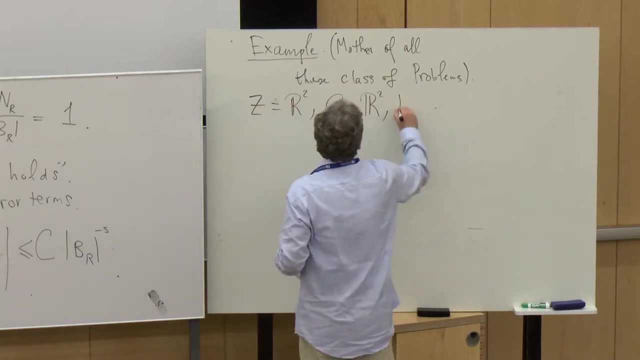 but nevertheless so. this is the mother of all these problems, this class of problems, and this goes back to Gauss. So in that case, Z is equal to R2.. G is equal to R2.. H is just zero. Okay. 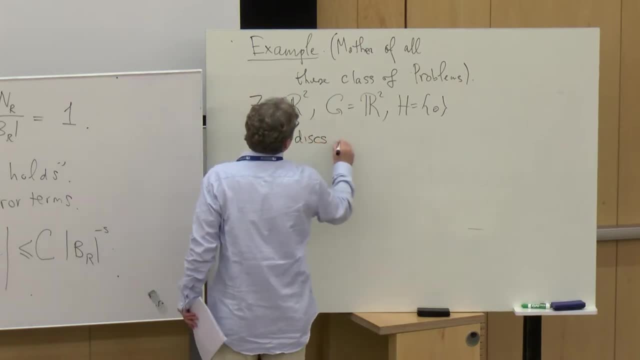 And the class of balls that we take are disks of radius R around origin. Okay, So in this case, maybe this should have been a better answer to Rami's question In this case. so Gauss said there is a hope, so it's validated. 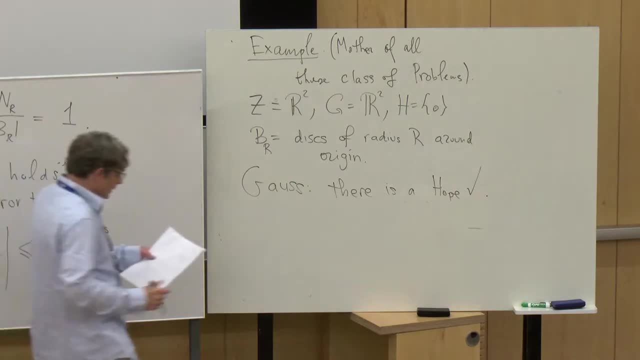 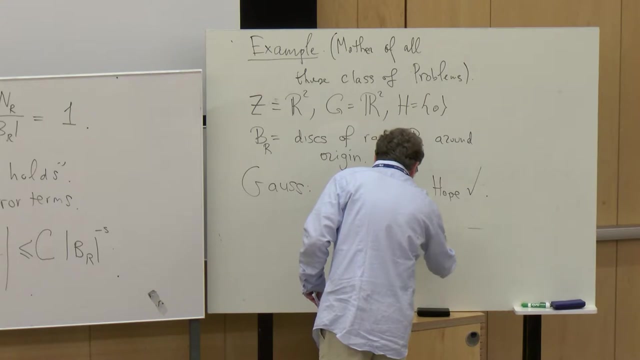 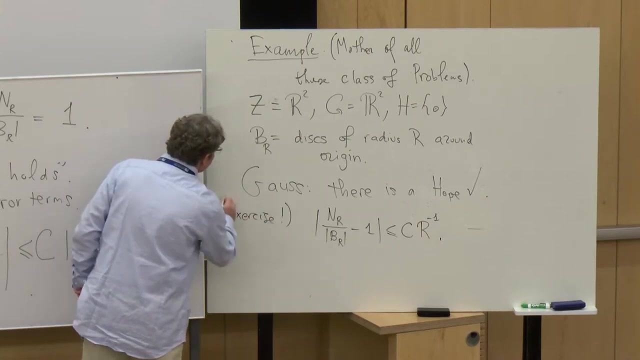 Actually Gauss proved more. He proved that nR divided by Br- now I normalize this- minus one- is less than or equal than a constant times the inverse of R. Okay, and I leave this as an exercise to the interested audience. 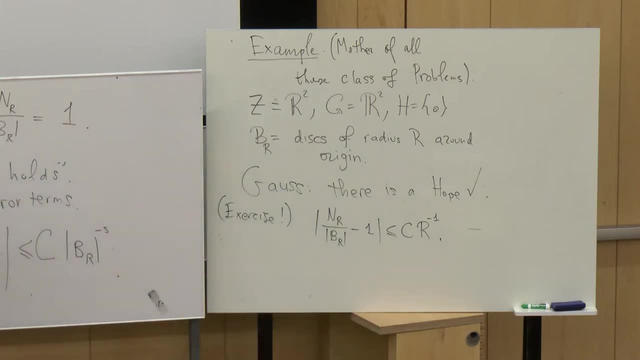 Okay, So people, usually there is an issue of normalization. People remember half, one quarter, never remember what we are talking about. The idea is that the circumference is the only enemy in this case. only near the circumference we might have rational points. 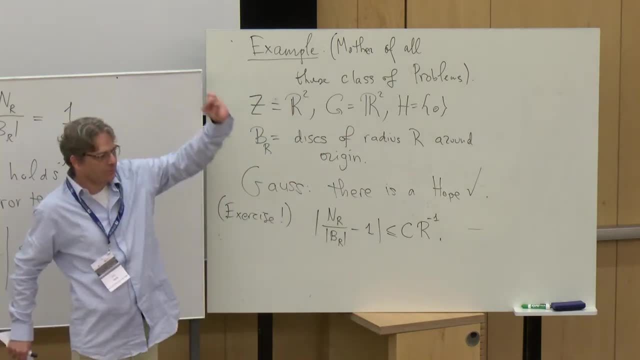 So the mistake is of the order of the length of the circumference. So the number of points in a ball of radius R is really R squared, or well, there is a pi somewhere, Yeah, And the mistake would be approximately constant times R. 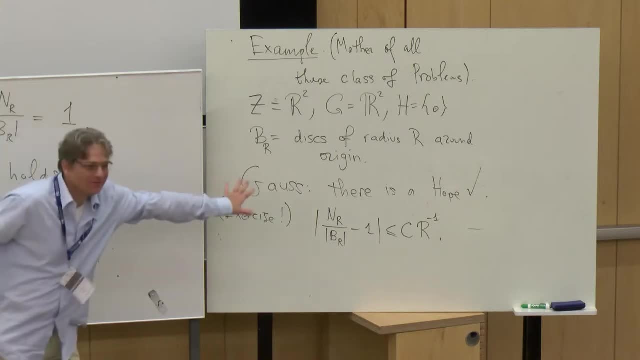 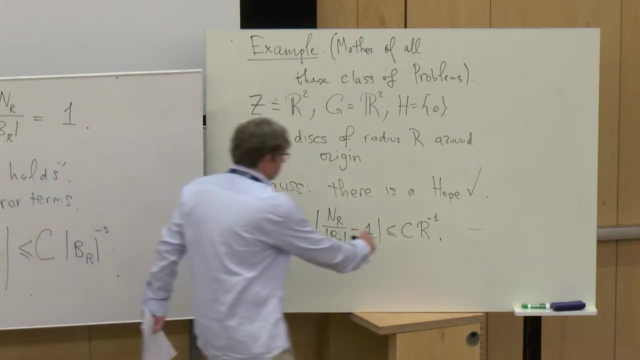 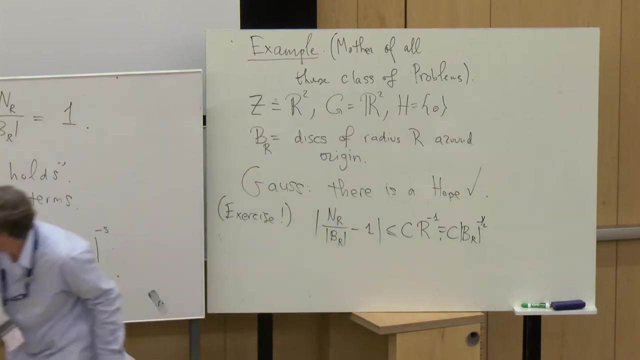 But with these notations it gets a bit ugly. but okay, So in that language H is one half. yes, Yes, Yes, Yes, you are right. Thanks a lot. This is what I should have written. I just wrote from the memory. 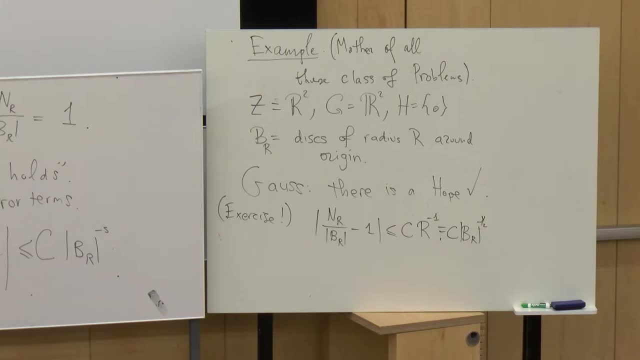 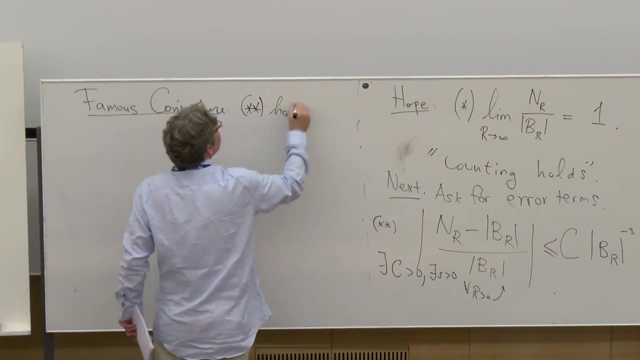 Yeah, Okay, That was good because you explained it Well. okay, With every mistake comes a redemption. The point is that there is a famous conjecture for those who are searching for double stars: Double star holds in this case with, and now I cannot remember. 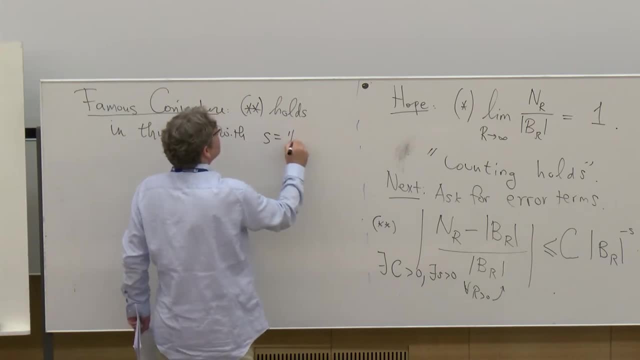 it's just going to be half of what I wrote. so one quarter, Is that correct? No, Three quarters. Three quarters, All right, Yeah, so it does, and it falls with three quarters. Okay, So I wrote a minus S, you see. 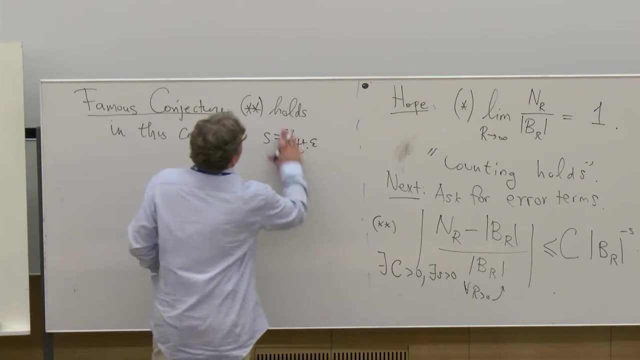 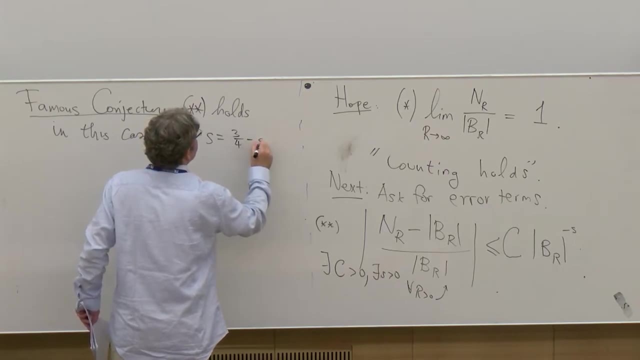 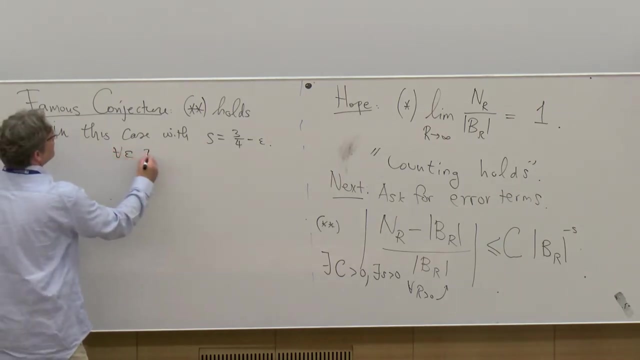 Minus S, So one. So what is the quarter? Three quarters is larger than one half. One quarter, no, No, Larger is more interesting. Right, Okay, This is correct, I'm sorry. Okay, For every epsilon. 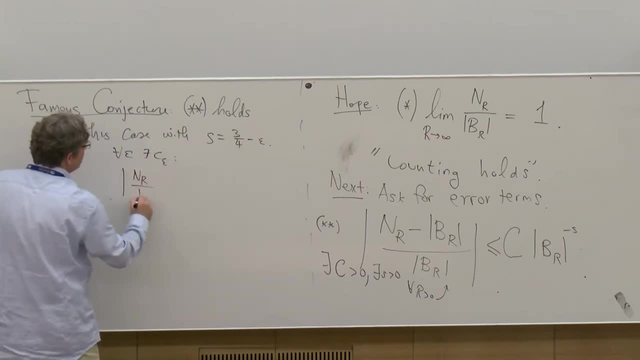 There is a C epsilon, such that the number of points in the ball, when you probably know what. Is there any other conjecture which is related to this? I don't know. Yeah, So I exactly wanted to say that I think this is what we want to say. 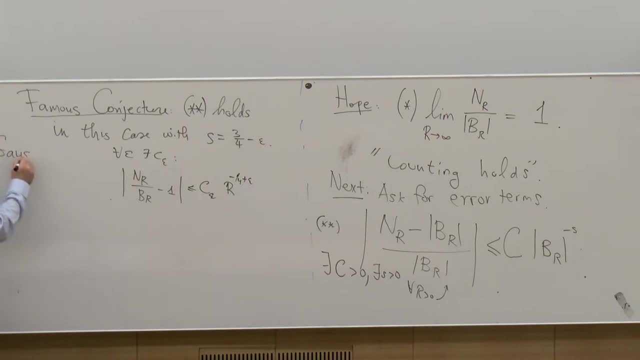 Yes, So this is due to Gauss. I'm not going to say anything about it. It's not related to, as far as I understand, it's not related to any standard conjecture in automorphic forms or in number theory. It is just then. 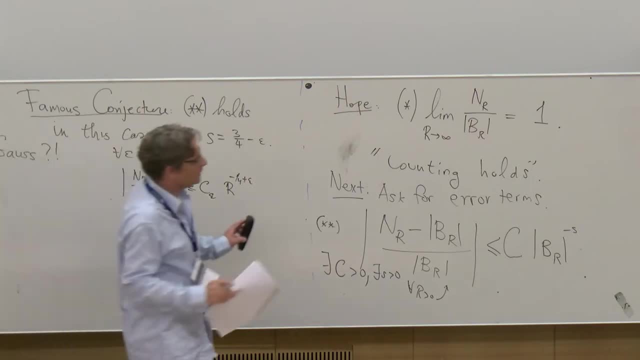 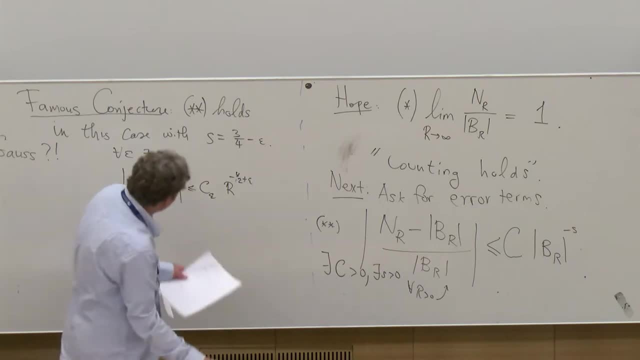 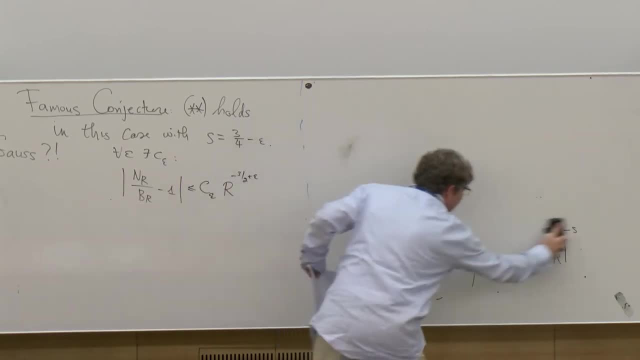 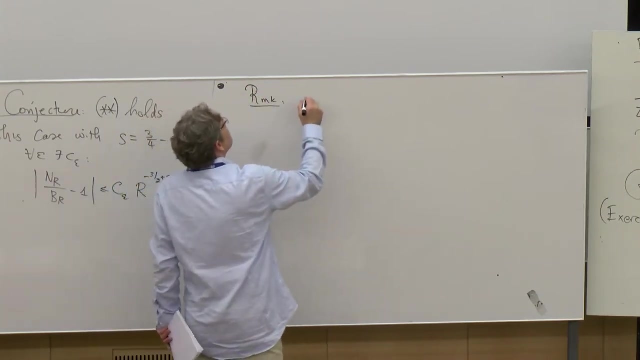 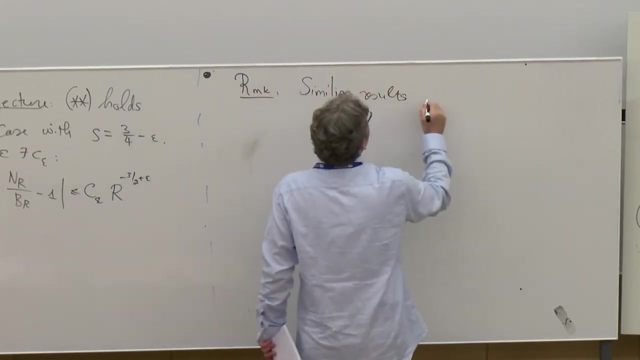 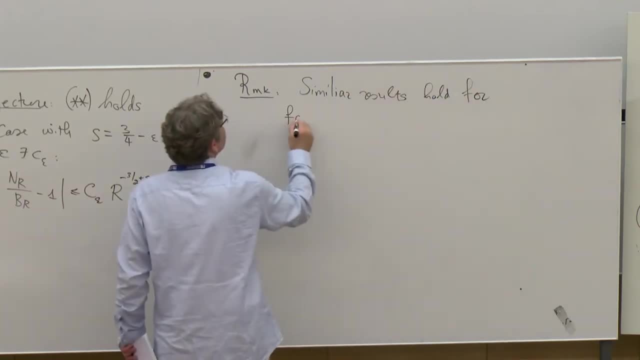 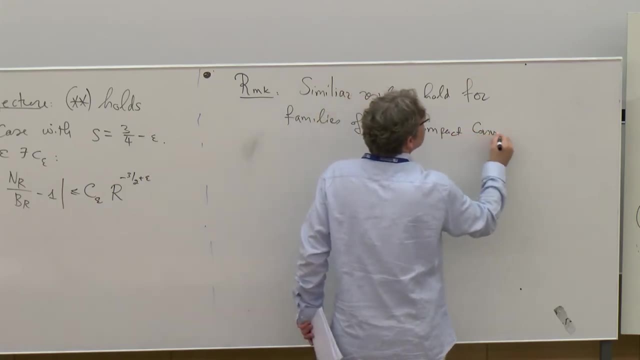 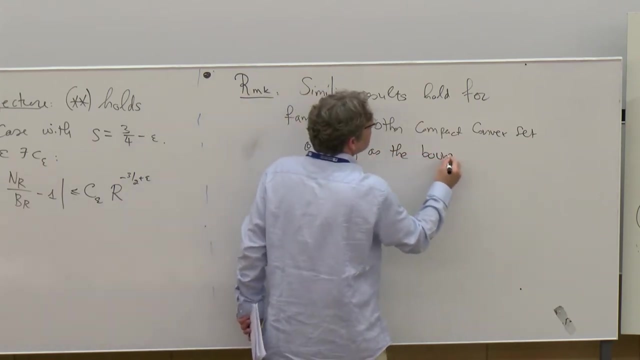 Okay are families of convex sets, of other compact convex sets, as long as the boundary is nice, say C2 or something like that. So on the other hand, you can't improve on Gauss, you can't improve on what I've written here. 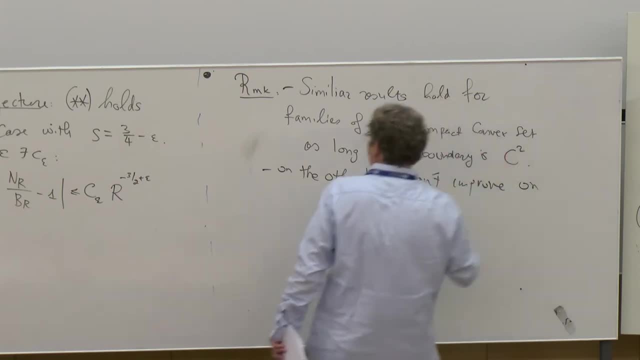 where is that? On this half on Gauss, if you work with bricks, with squares, So if you work with bricks, So if you work with bricks, So if you work with bricks you're counting in in sets which are kind of not so nice, then this is the 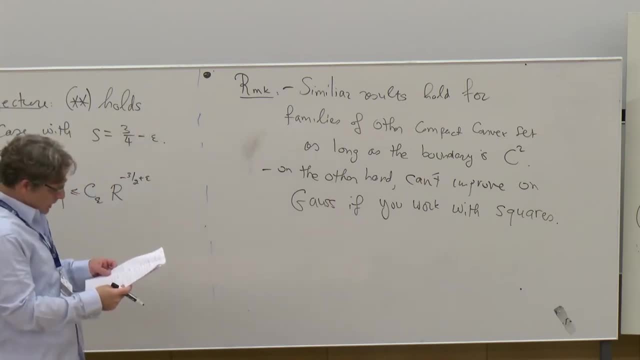 error that you anticipate. you just check that. so we see that in this whole problem there is an issue of deciding which sets to counting. so this is one of the things I want to to discuss. before before doing that, let me mention another famous example. okay, just just to be sure I will not say anything new about Gauss. 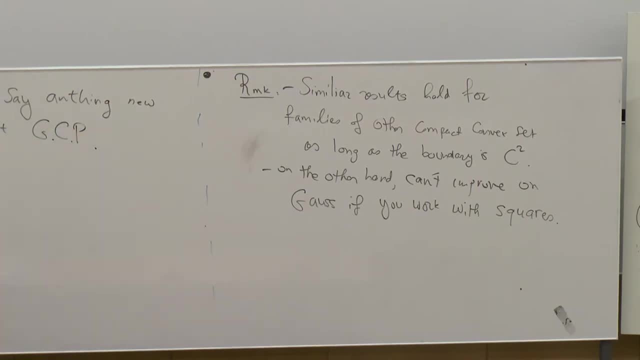 circle problem. okay, this is Gauss circle problem. okay, but somehow I hope that now the target is clear. it's very elementary. we just want to count how many points there are approximately and then to say something about there. and, as I said, this is a very well rehearsed subject and many, many people 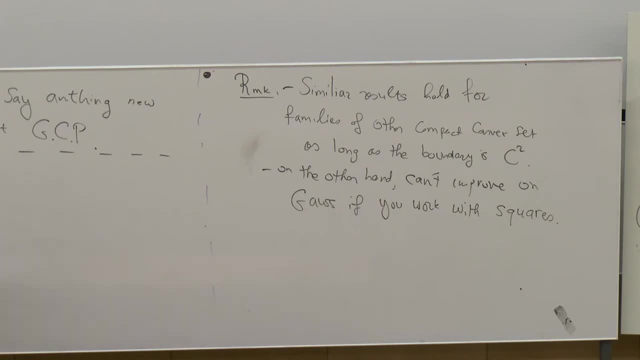 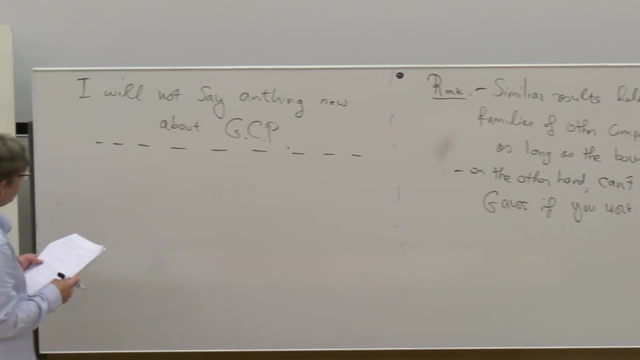 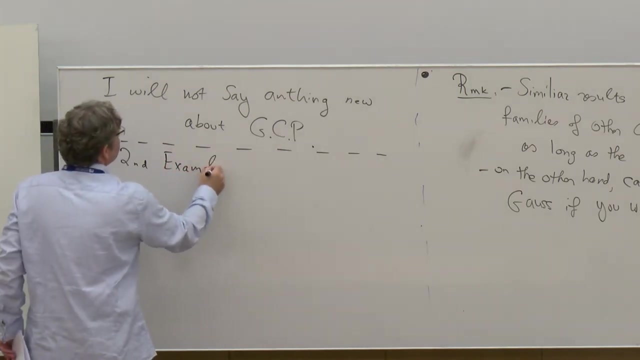 have contributed and I will not be able to mention all the names, but some names do stand up and I will just mention them as part of my introduction. so maybe the second example, which is a. usually I thought it's attributed to sell bird, so this is due to. 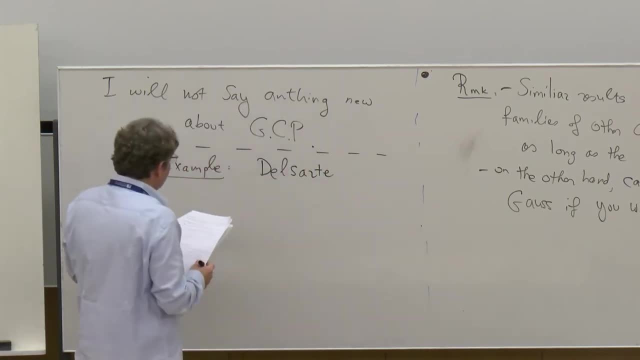 the start. so he, he initiated the study. his thinking was over. a kiss to me people who tell me the history. he initiated the study or he studied, initiated study, the case of the hyperbolic plane, the upper half-plane of Z being the upper half-plane. 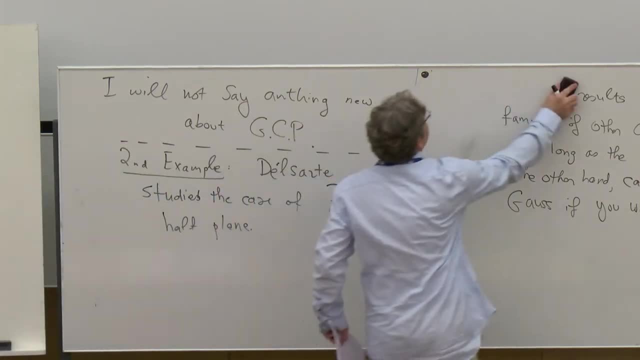 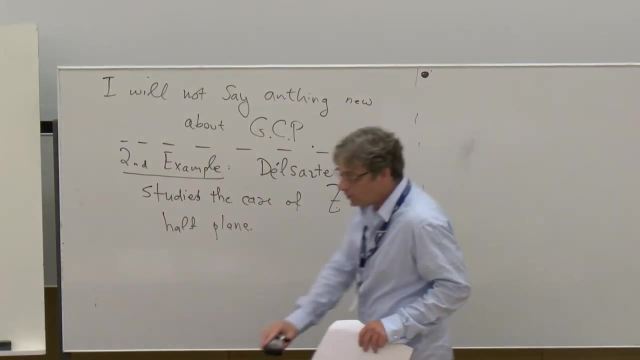 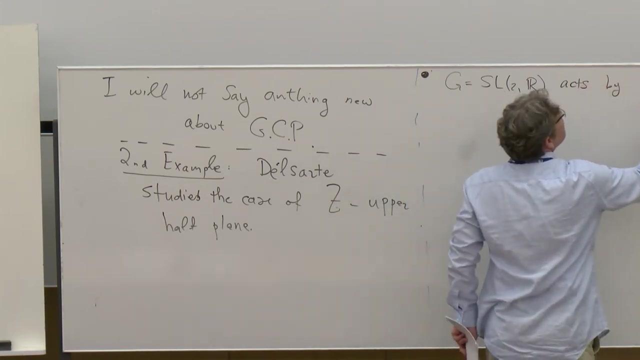 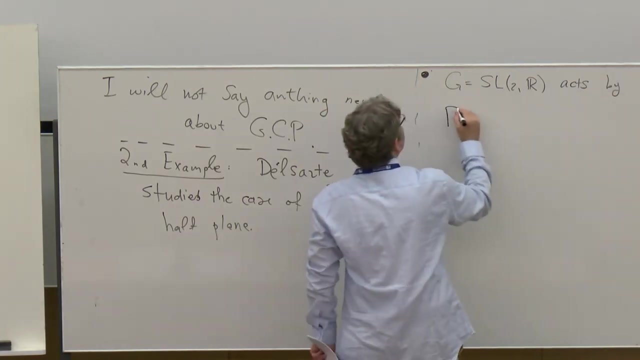 So in this case the groups which play a role are familiar to us. so G is SL2R. could be also PSL2, just for simplicity. So this acts by fractional linear transformations on Z and gamma. I will take it to be SL2Z. 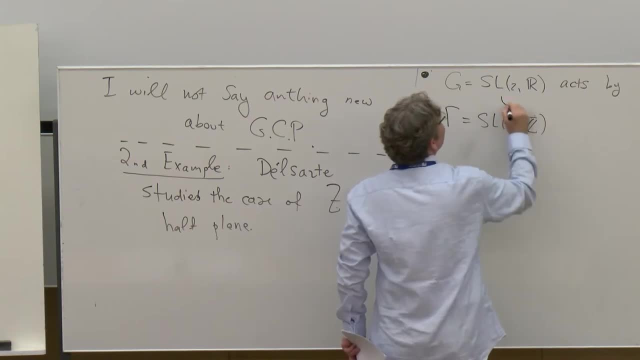 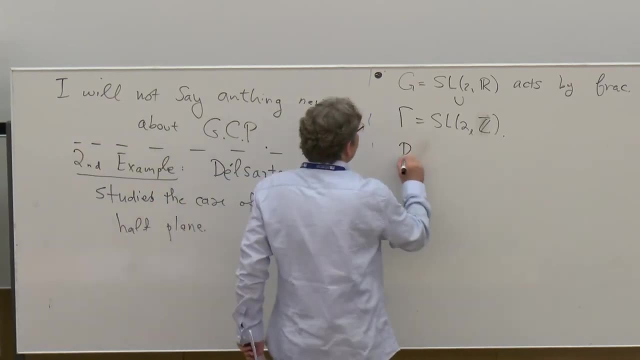 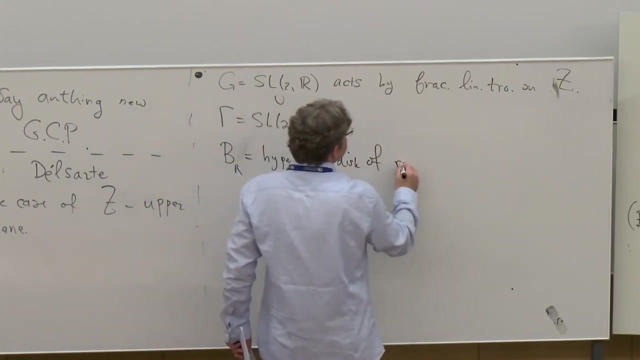 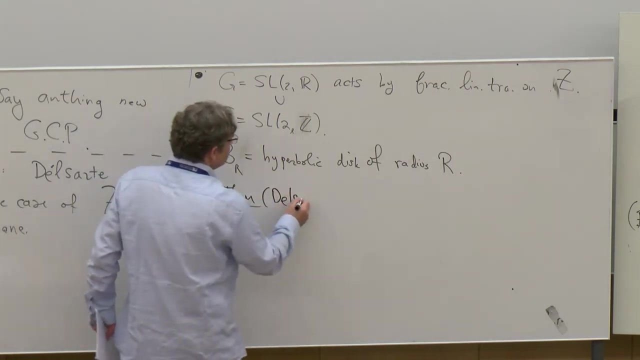 it's a different Z, sorry. okay, so these are the kind of gammas we like, And BR is going to be a hyperbolic disc of radius r eminating from the point i. okay, So, uh, the theorem of Tilsart is yes for star. 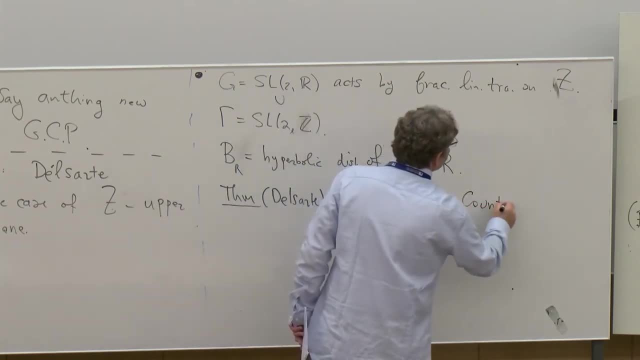 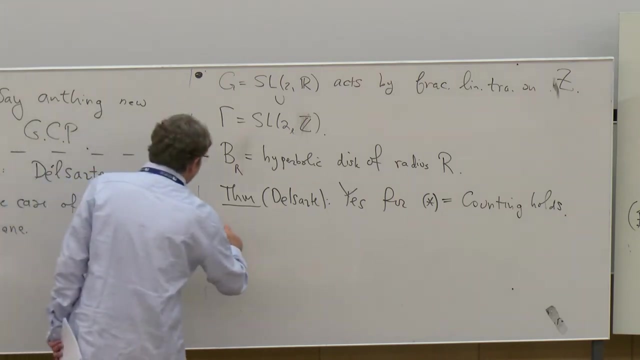 Or is, In other words, counting holes? The number of points is indeed proportional to the volume of the ball. I should remark that there was a foundational work by Selberg later. Selberg who studied this problem. I don't know the history, but in relation to his trace formula, 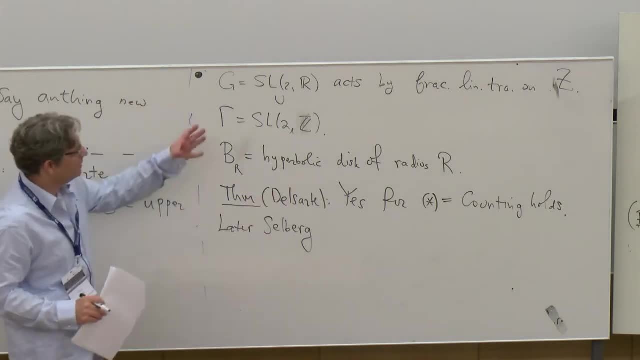 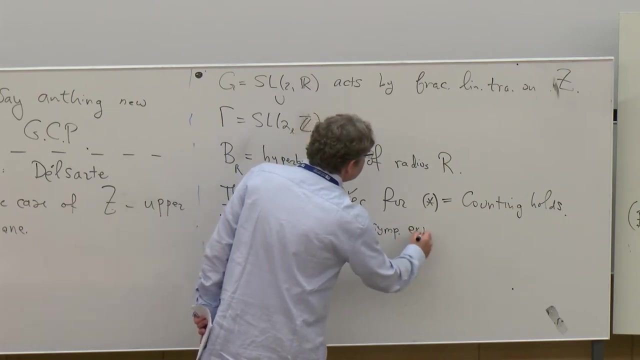 and he achieved fantastic results regarding this number. nr So Selberg produced a certain asymptotic expansion. I'm not going to write it: Asymptotic extension plus an error term, and the error term he got in my normalization is br to the minus one-third. 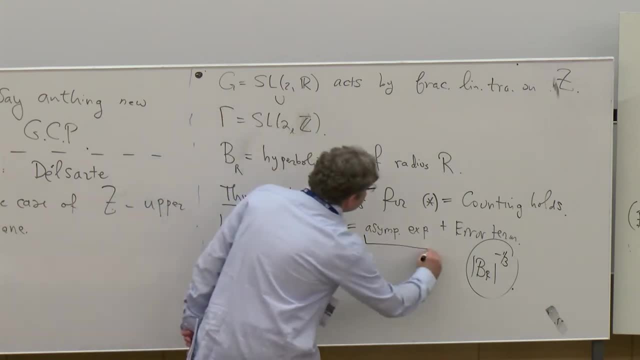 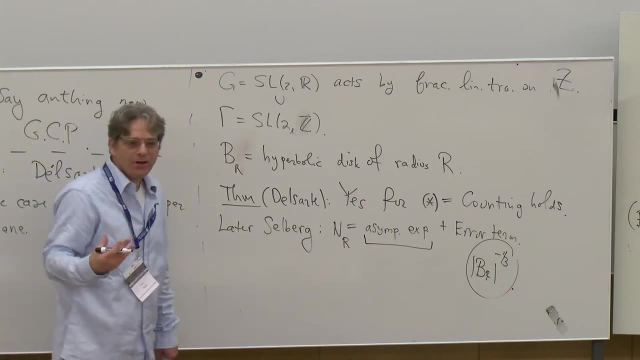 and the asymptotic expansion depends on. so the quantities here are objects occurring in the theory of automorphic forms. So he used- maybe I'll just write the formula. I will not explain the notion in the formula, I'll just write it and you will feel what it is. 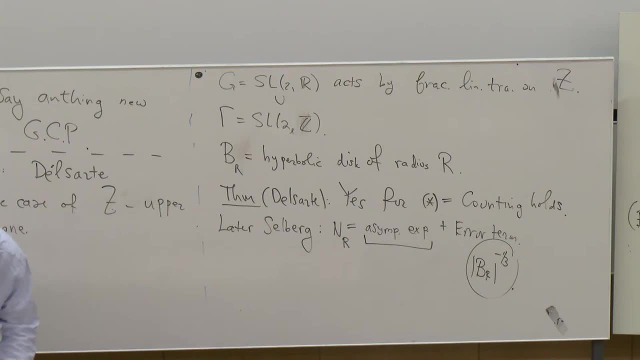 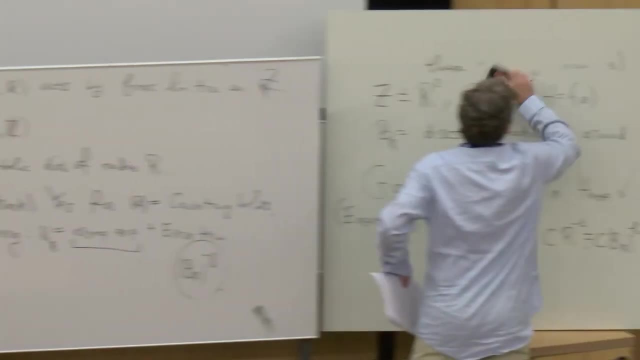 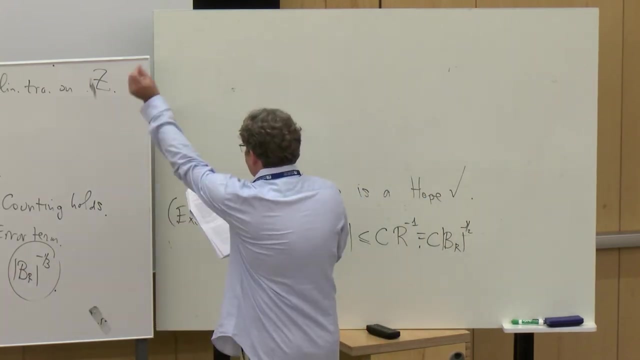 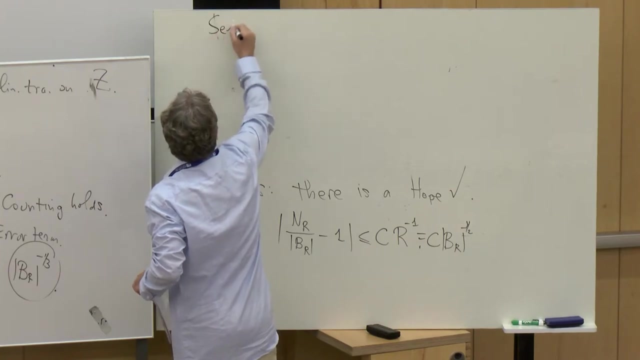 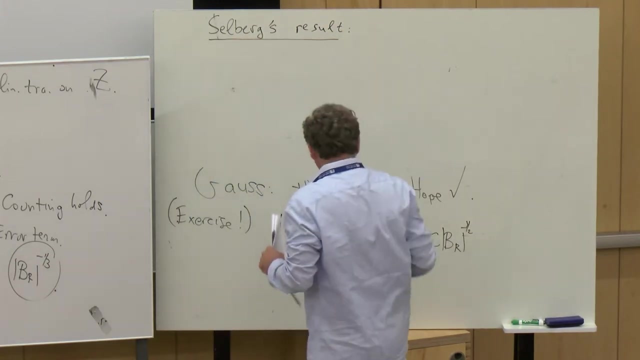 Just I'll copy it, because I don't remember it by heart. I'm too old already, So I'm going to write the formula for this. So more or less just Selberg's result, and I'm pretty sure that you will have many questions after that. 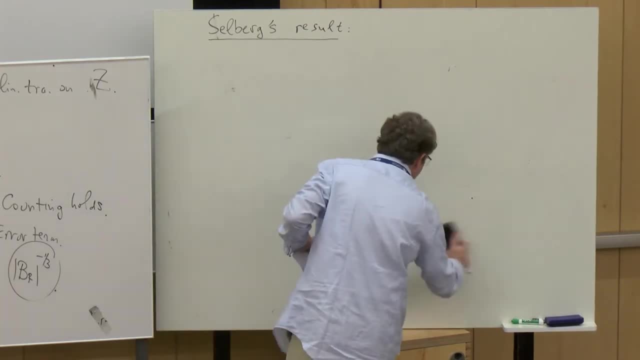 I will try to avoid answering because I don't want to, because I don't want to, because I don't want to and I don't want to take too much time of the lecture for that. but it's a beautiful result. 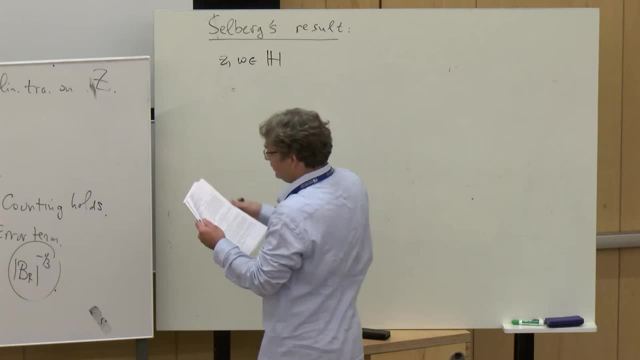 So, to formulate it, I will not use the notions I have introduced, but rather a different one which is equivalent but nevertheless. So I fixed two points in the upper half plane and hyperbolic plane, and defined a number, nr. 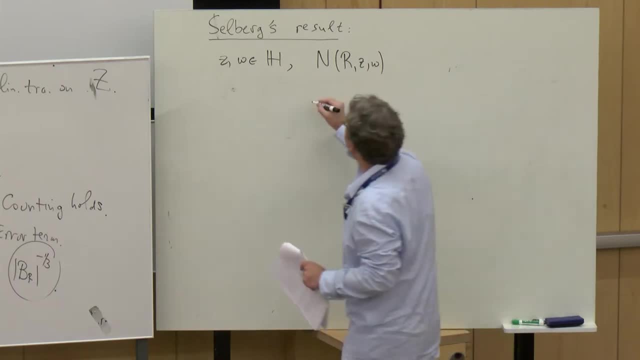 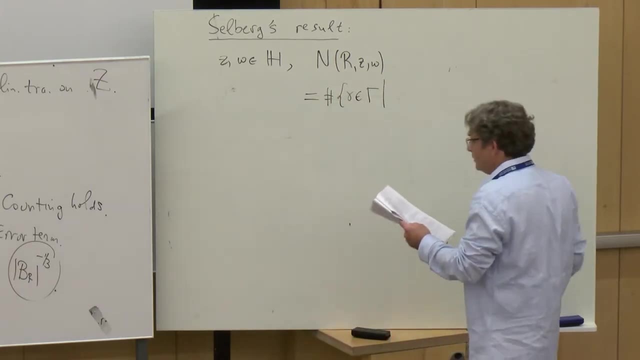 but now with two parameters, z and w, And this number is going to be the numbers of gamma, the numbers of gamma in gamma, gamma being SL2z, which satisfies some strange inequality: twice the hyperbolic cosine of the distance between gamma z and w. 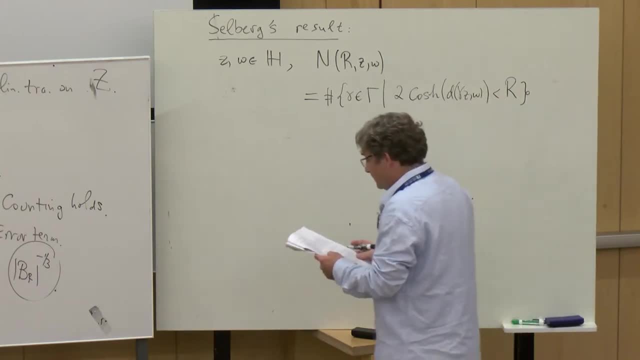 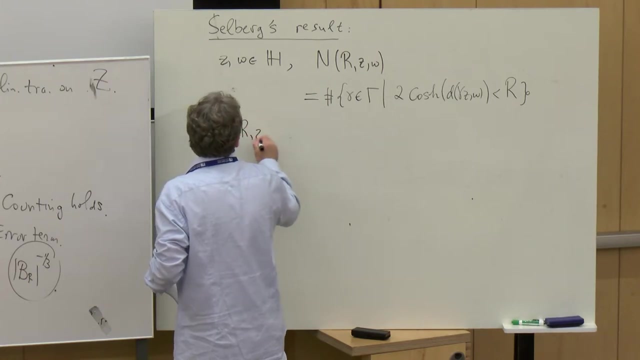 less than r. Okay, So just to fix ideas, the formula that Selberg produced for this nr z w- I'm not writing the connection to this number, but it's very easy to work out. The formula is the following: 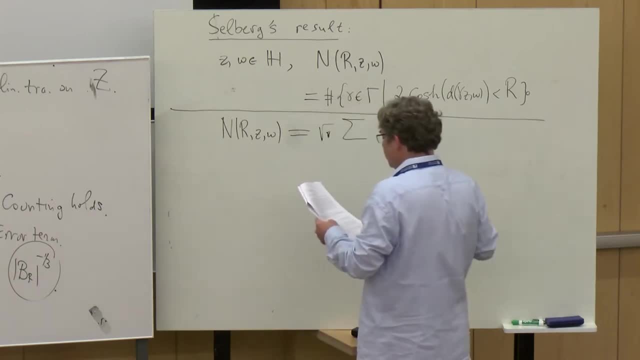 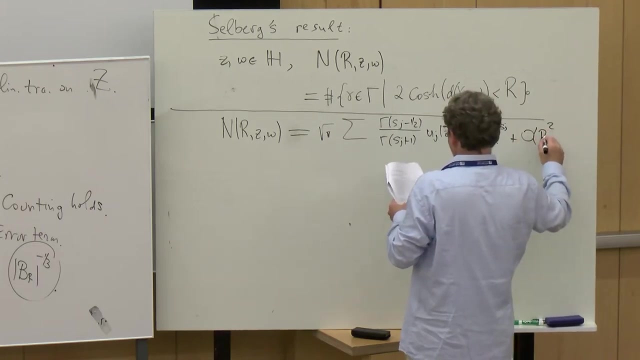 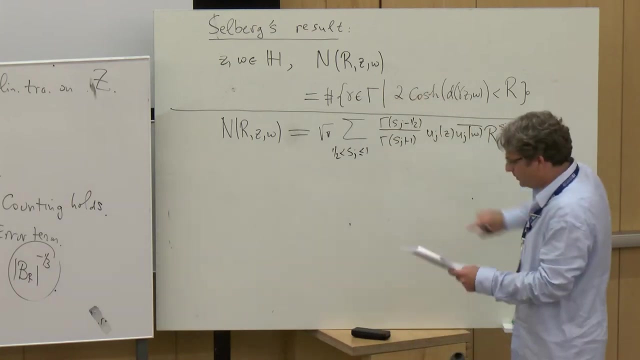 it's square root of pi and then a sum of some values of gamma functions- I don't know if it is visible- and the sum goes over some eigenvalues between one and half hidden. here is a main term, so it could be that I'm missing here. 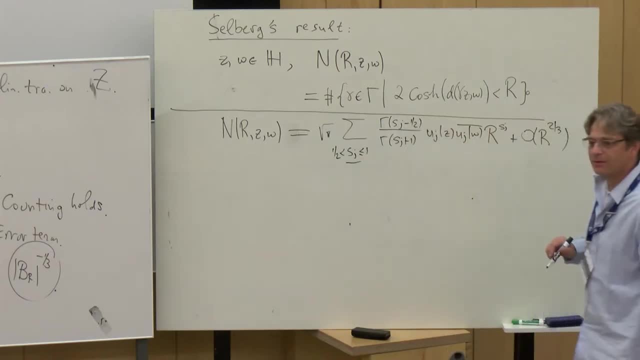 s equals to one. oh no, it's one. okay, the one is here, okay. So the main term of this sum belongs to the eigenvalue which corresponds to one. so in this normalization these are eigenfunctions. on L2 of SL2r. 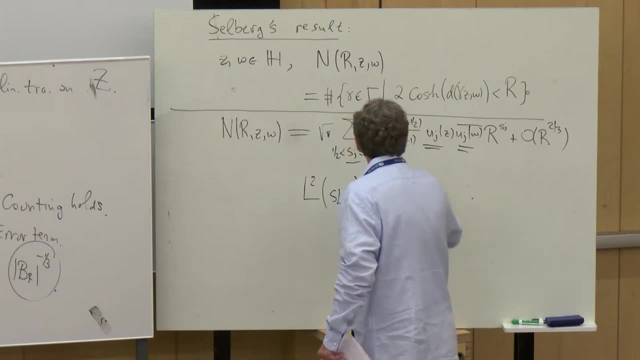 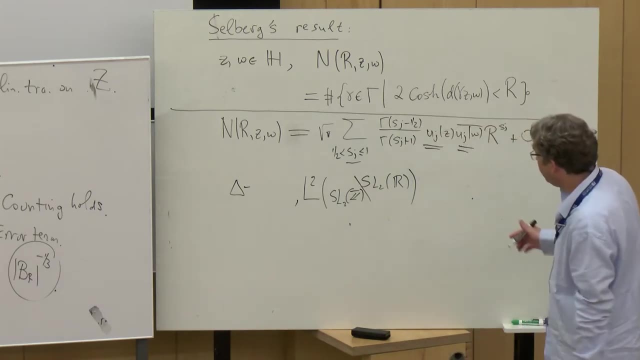 divided by SL2z of a certain operator which I'm not introducing. Okay, So there is certain L2 theory which Selberg produces, and today we call this the theory of automorphic forms, So the vast generalization of what he produced. 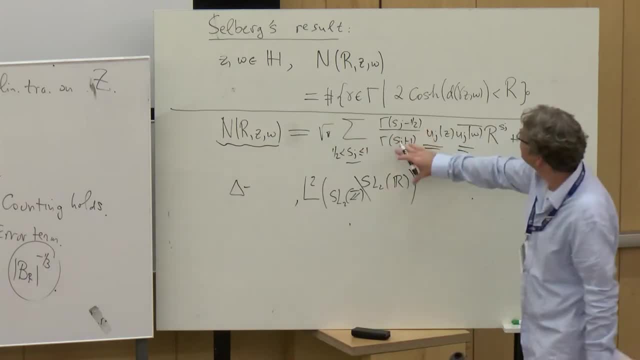 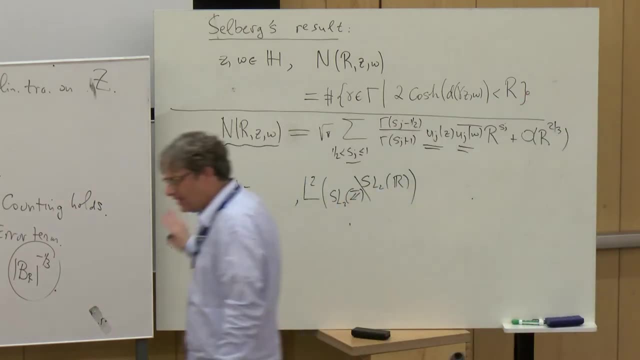 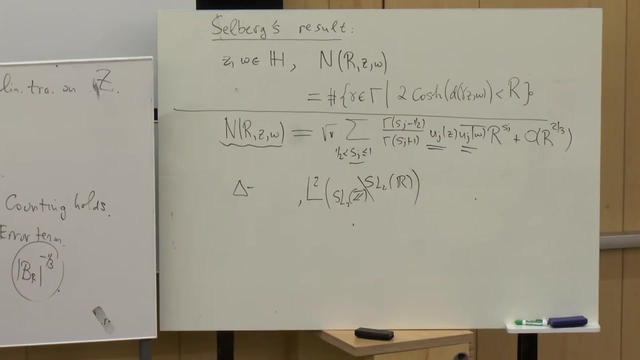 and these numbers occur in a natural way in relation to exceptional eigenvalues and other things in this formula. So I just wrote this on the blackboard to say that this counting problem it really relates to geometry. but if you want to really go further, 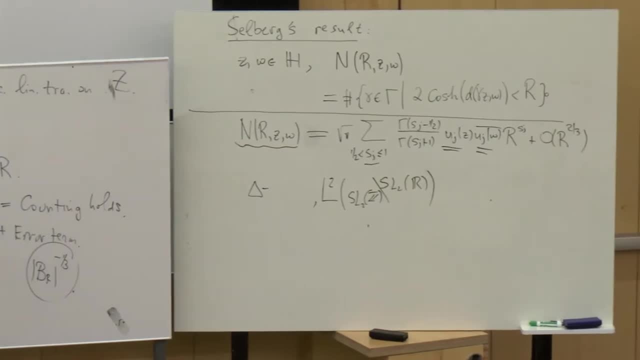 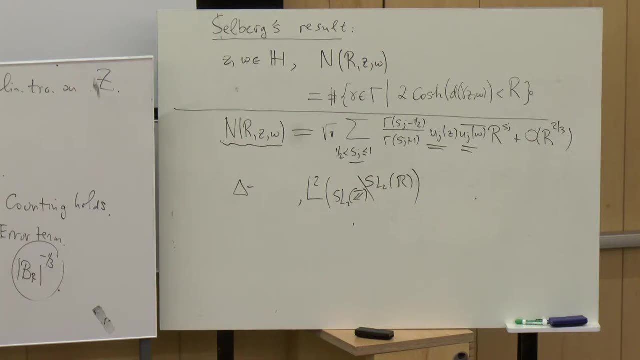 you touch number theory And in some sense our study, which is not that deep, is trying to see how far we can go with analysis without getting into number theory. Okay, So in some sense, the shape of the balls, if they are allowed to be arbitrary. 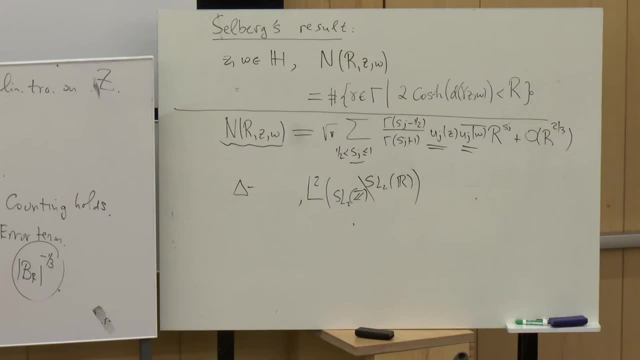 then in some sense there is no number theory. Okay, So if you can obtain general results in terms of the shape of the balls, then maybe your result is from geometric analysis. Okay, So I just wanted to give some feeling. I hope I didn't waste too much time on that. 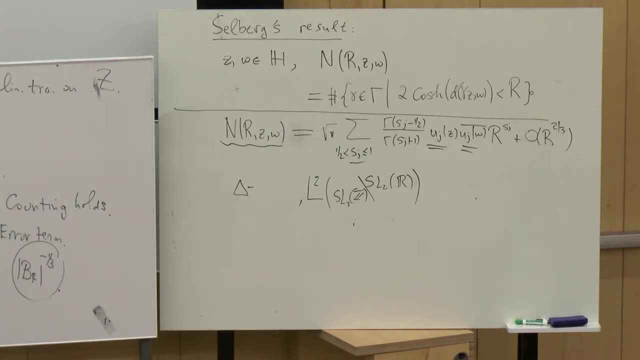 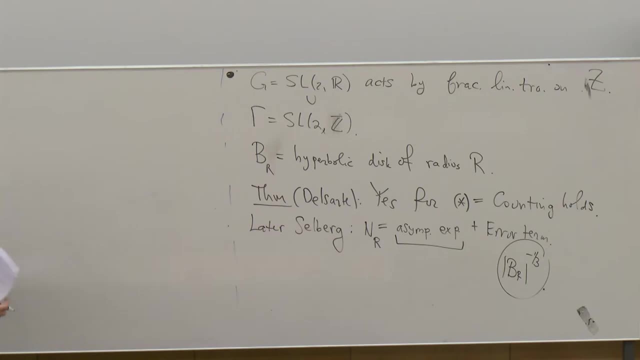 So just to finesse the setup, let me maybe formulate the result. Okay, so let me repeat Gauss from the Math Olympiad. then Delsarte and Selberg do this thing, which is much more, I mean can get much more advanced. 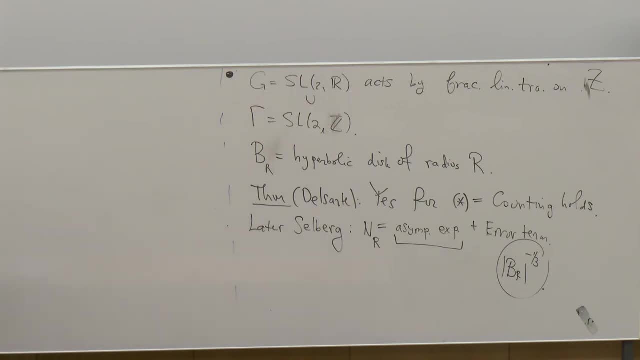 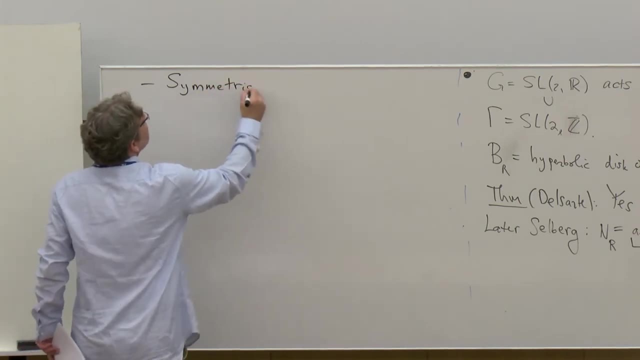 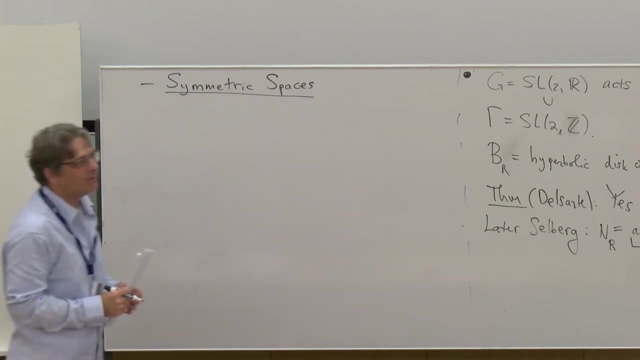 And the next in this non-really historical setting, sorry, is the case of symmetric spaces. So for symmetric spaces, which is one way of generalizing the upper half plane. so okay, in this audience maybe I don't have to say too much. 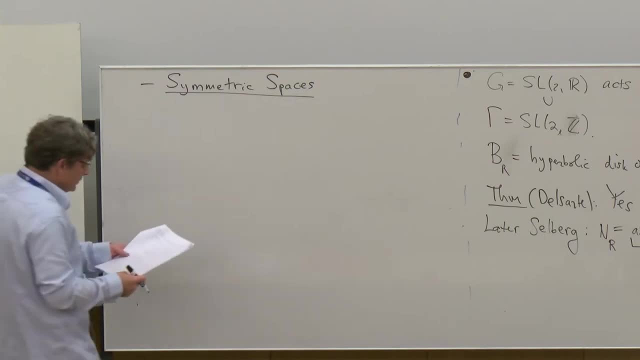 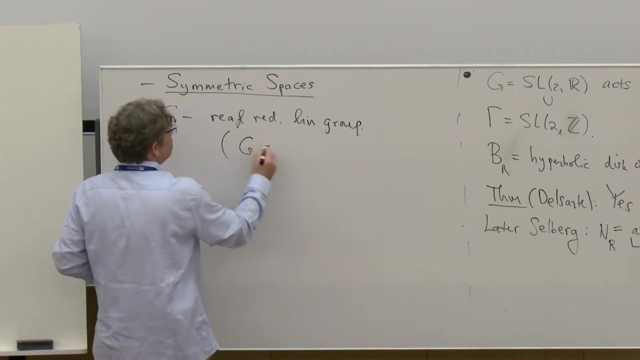 about what I mean by symmetric spaces, but nevertheless. so I will take G to be a really reductive linear group and I will assume that. so this: for me G is a subgroup. it's a closed subgroup of GLNR or maybe GLNC. 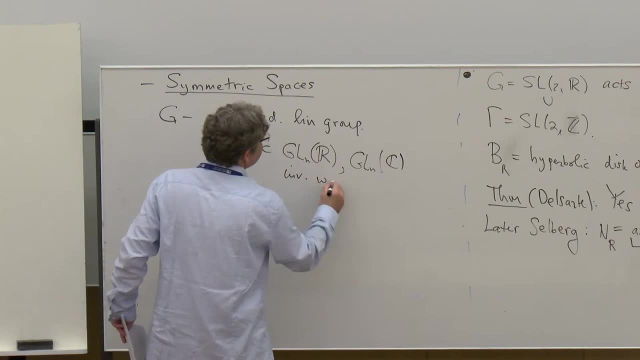 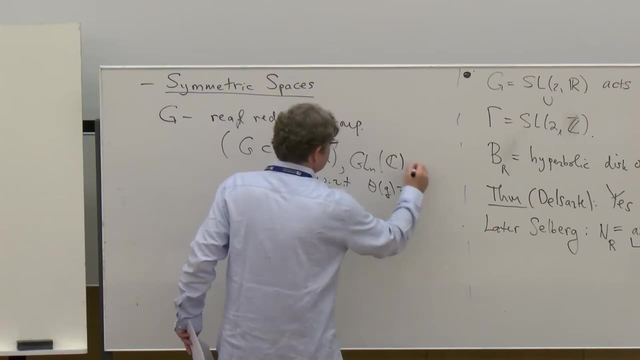 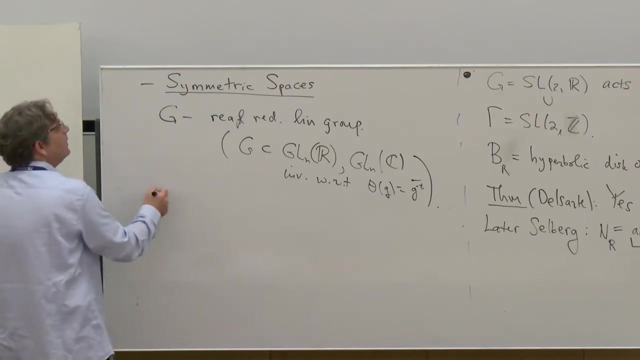 and I want it to be invariant. invariant with respect to our beloved involution, theta, the transpose, inverse, and maybe a bar, if needed. Okay, so some classical object of what we are working on. So, in this setup, so it is known. 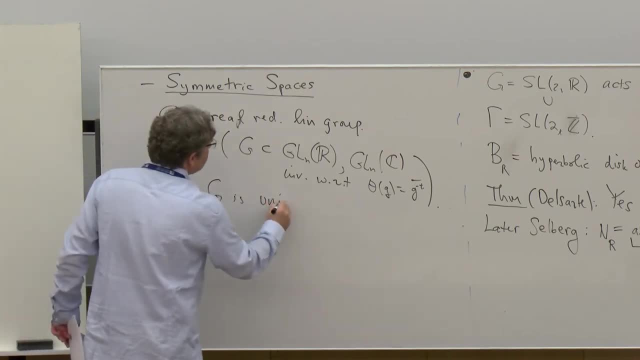 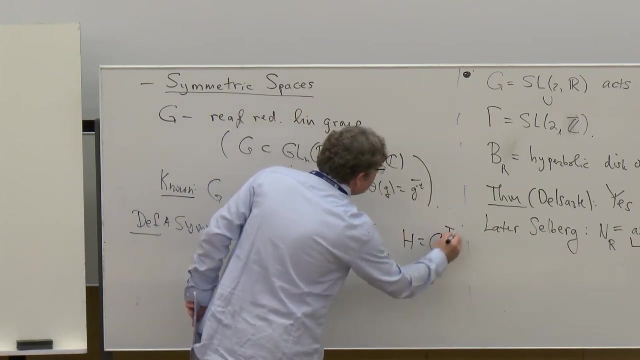 that then G is unimodular, so there is a natural way to take a measure, and so the definition for symmetric space that I'm going to take: symmetric space. asymmetric space is a gadget of the form G mod H, where H is the fixator. 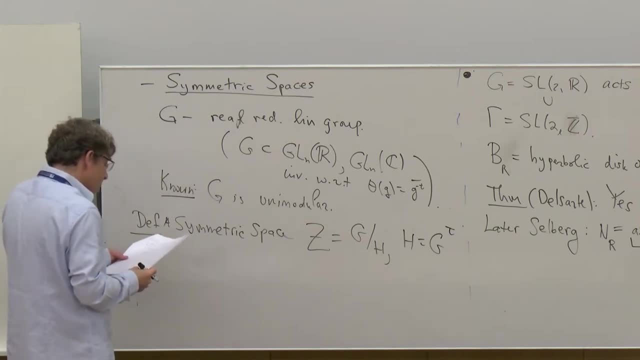 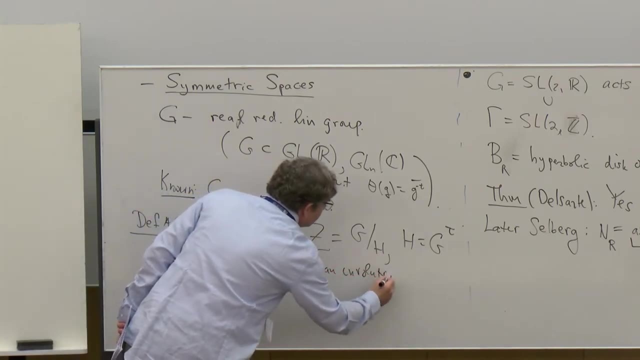 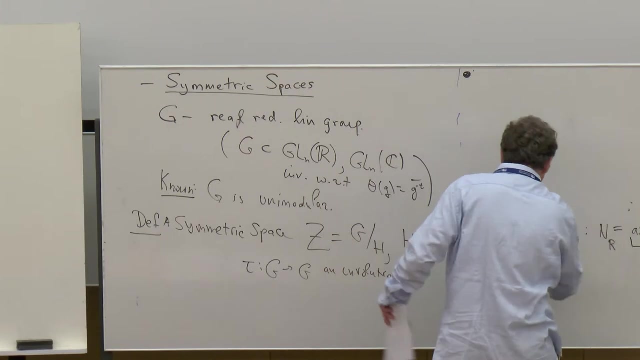 of an involution on G. So tau, from G to G is an involution. Okay, One can go with more general things. you don't have to take the entire fixator. you can take connected components, you can take something in between them. 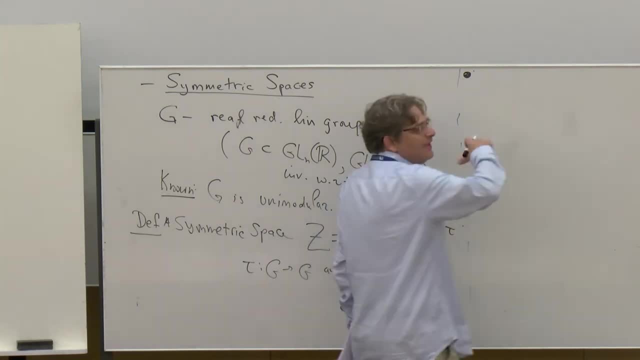 these are small things which are not relevant here, and they are kind of vaguely broken into two classes. we have the Riemannian ones- Riemannian- I think I'm missing an N- yeah- Riemannian symmetric spaces. 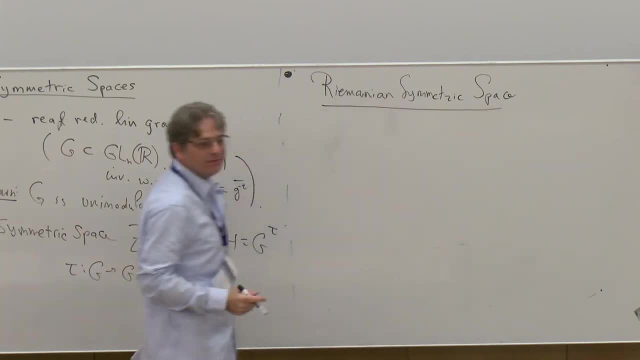 So grosso modo this corresponds to the case that H is compact. So if we define tau to be theta, restricted to G, so theta was- maybe it was not clear- theta is an involution defined on this big group, I can restrict it to G. 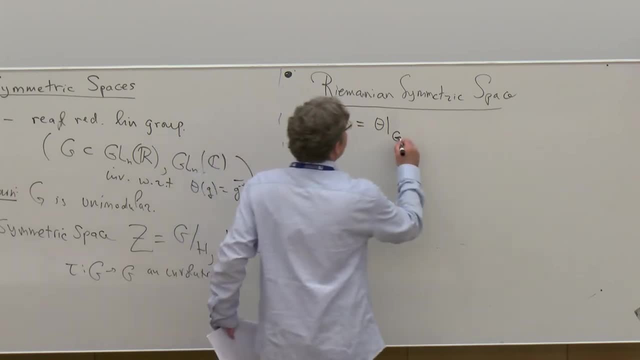 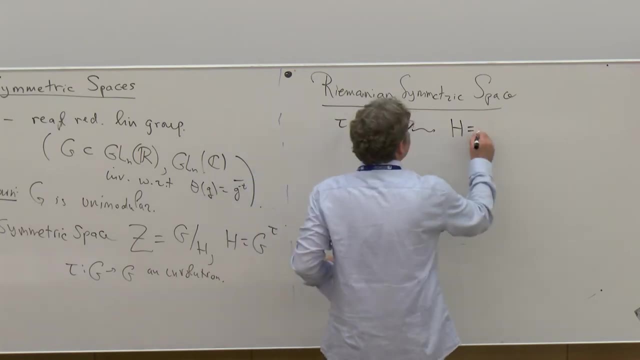 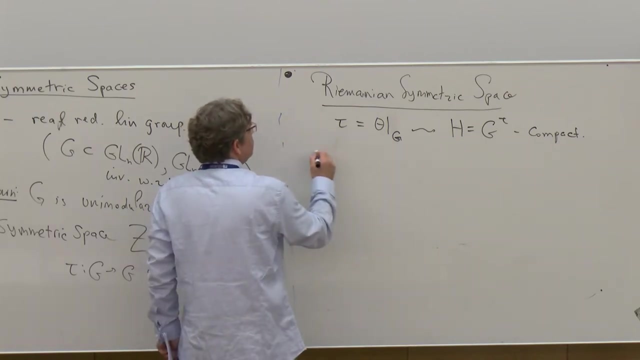 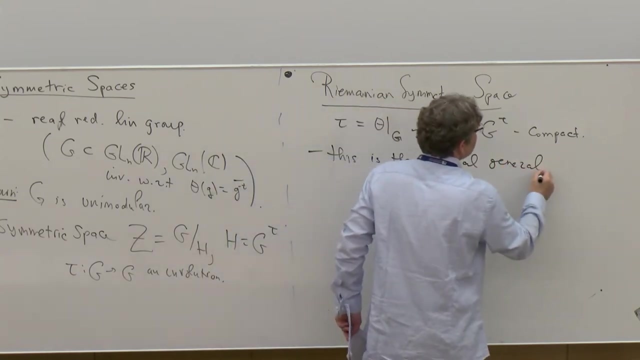 and define an involution. now on my G, and this leads to H, which is going to be well. tau is compact and it admits the Riemannian structure. so this is, this is the natural, this is the natural generalization. 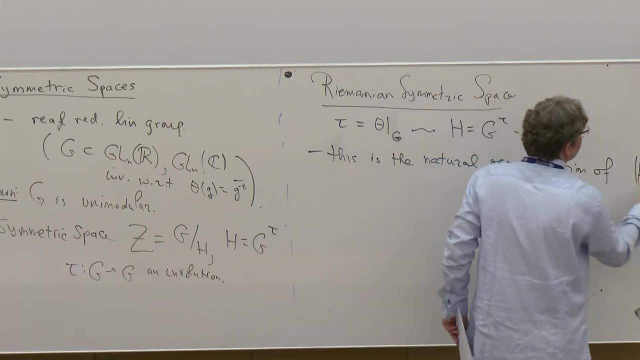 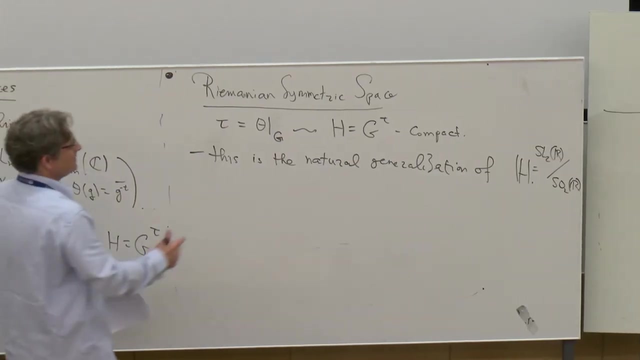 of the upper half plane. Yes, so if we take SL2R and divide, or maybe PSL and divide by SL2, then we get our. What is the generalization? G mod K. Okay, So so we call it K now. 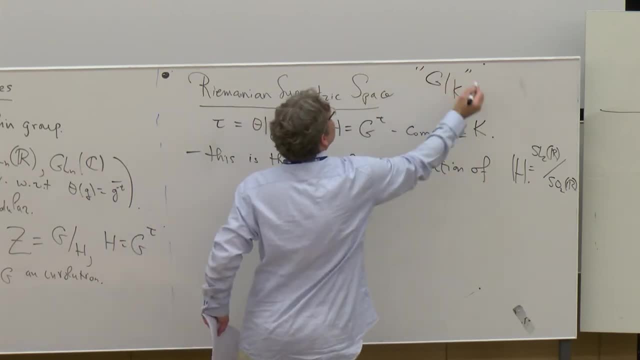 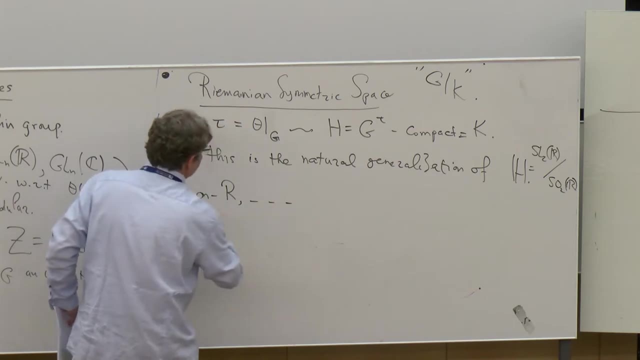 Okay, so these are the G mod Ks. Okay, And then there is the non-Riemannian. non-Riemannian- Okay, So here the H is not compact, the involution is not conjugate to to this restriction. 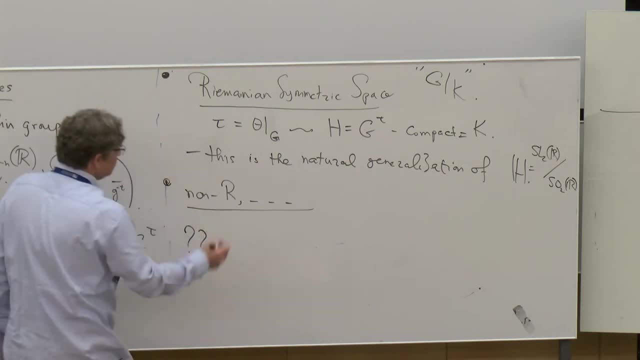 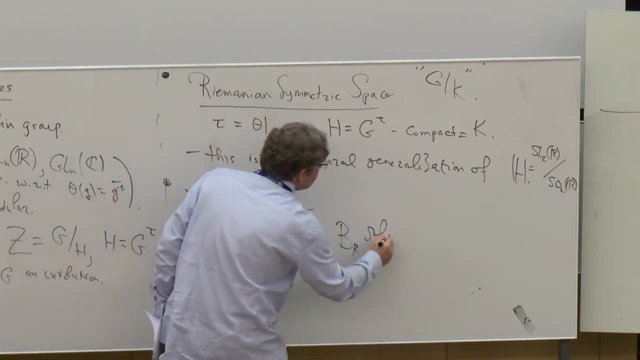 But in both cases, the question that I want to address is what both the R should we take Okay. should is is a hard problem. I want to take Okay, So when I write here it's visible, or? 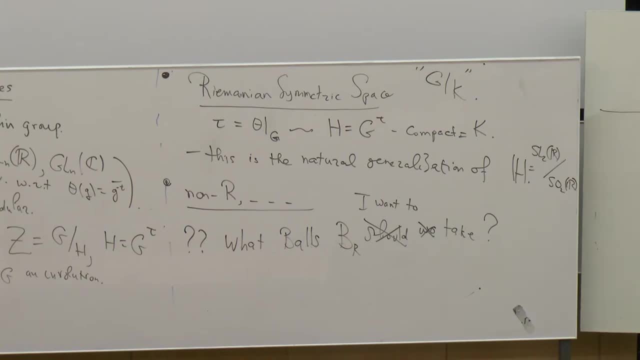 Is there something like for some natural within some natural families? I don't know how to answer that. Okay, Yeah, but certainly I suspect that there is some natural class of balls and I want to introduce them. Okay. 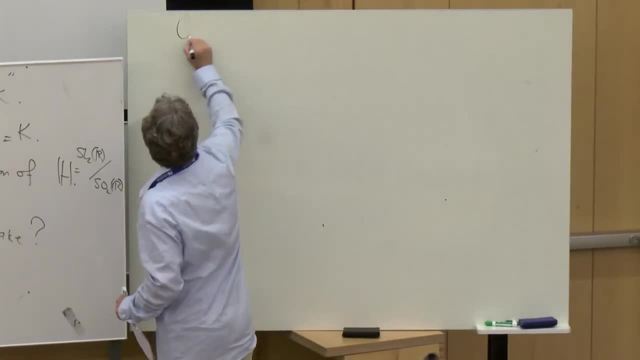 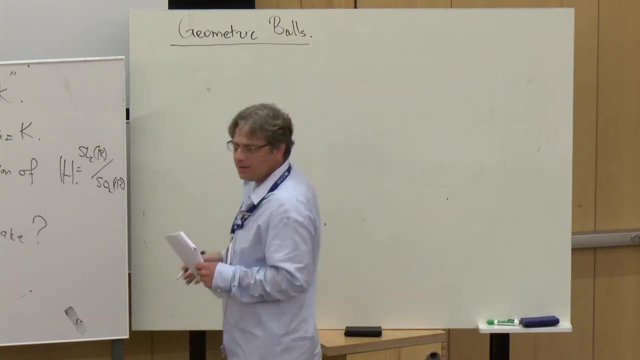 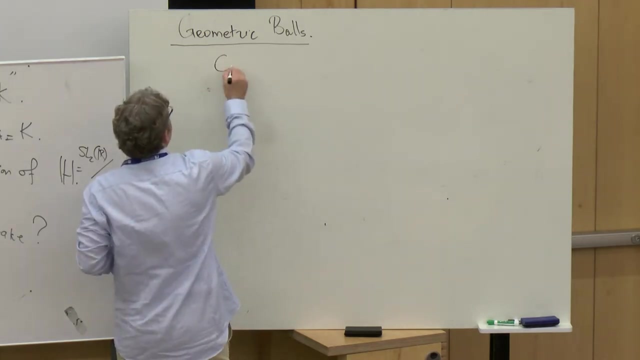 So I will call these maybe geometric balls. Okay, So the geometric balls are obtained by. I will assume that, as before, Actually, this can be done in any in a more general setup. So can be defined. 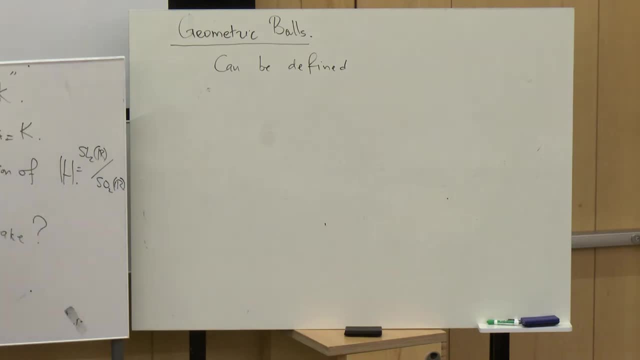 I forgot to say that the spaces that we obtain here is called G mod. H is symmetric spaces are always affine. These are affine spaces. H is reductive, but these spaces are affine. Okay, I will slowly go into. 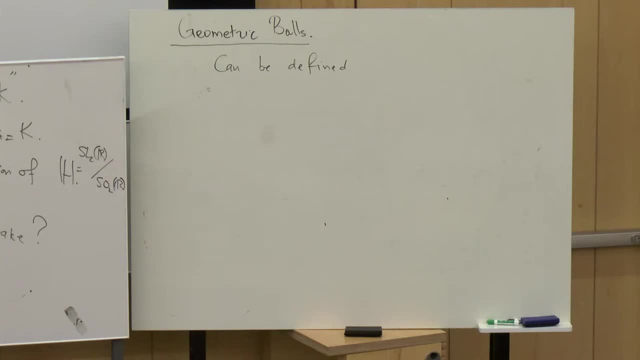 more, more general spaces. Now, regarding the, the question whether the hope is validated, et cetera. Yes, there was a foundational work on this by Duke Rudnick and Sarnak and by Askin. 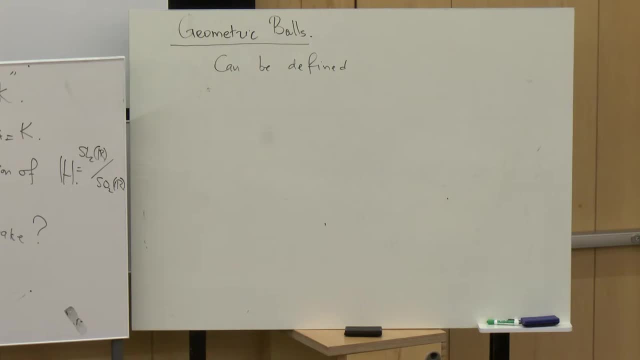 and McMullen, And they established the counting property for all symmetric spaces. Okay, I will say more on that in a second. but they did not discuss- at least not in their paper- the error term estimates. 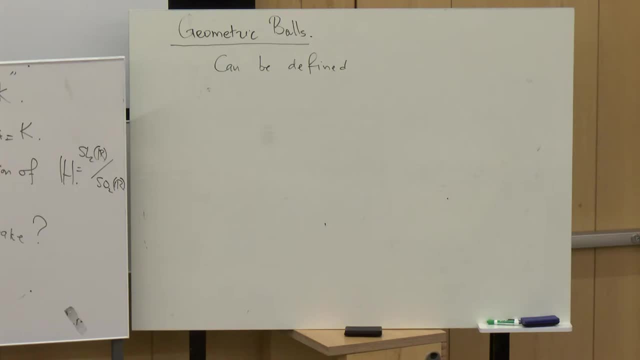 And What The word affine To me. to me, yes Over R, Yes, Okay, So I, I. I will go to a more slightly more general setup. So can can be, this can be defined. 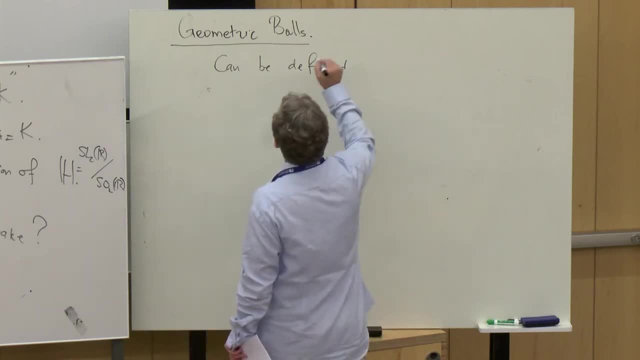 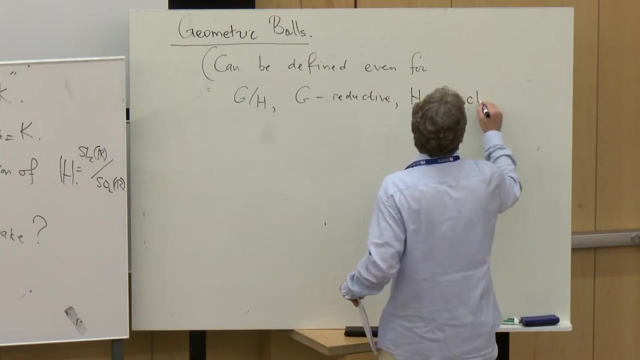 even for G mod H, where G is is, is is where G is reductive And H is is a closed subset. Closed subset. Closed subgroup. Closed subset. Okay So. 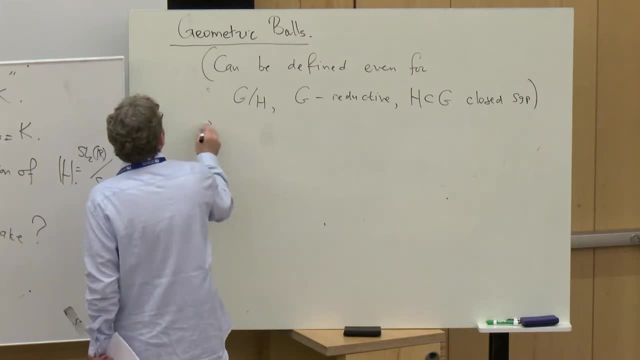 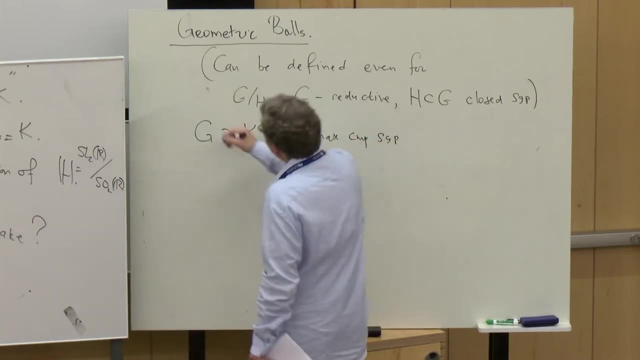 I just wanted to to to illustrate the idea. So G has in it a maximal compact subgroup. Well, it has main, but And so, G being a re-reductive group, it carries with it this Riemannian symmetric space. 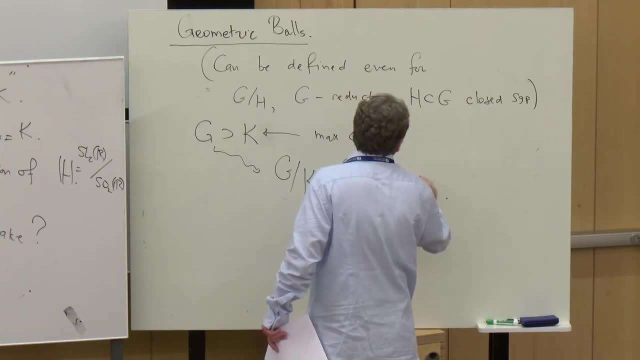 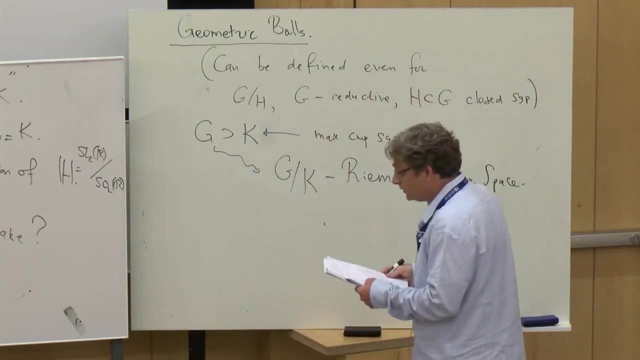 This is a Riemannian symmetric space which it comes for dinner even if it's not invited, So it has. so this guy has an invariant metric and we can just lift it to G, So and then push to H, So that gives us a way to to G mod H. 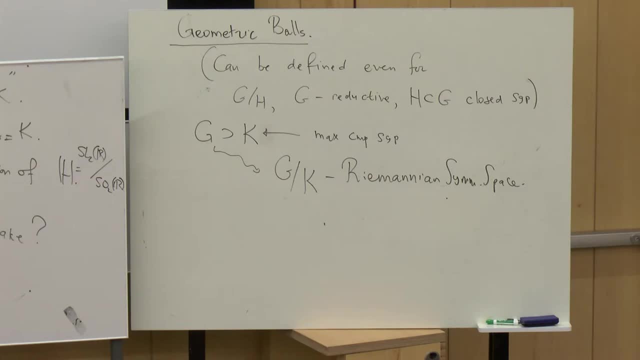 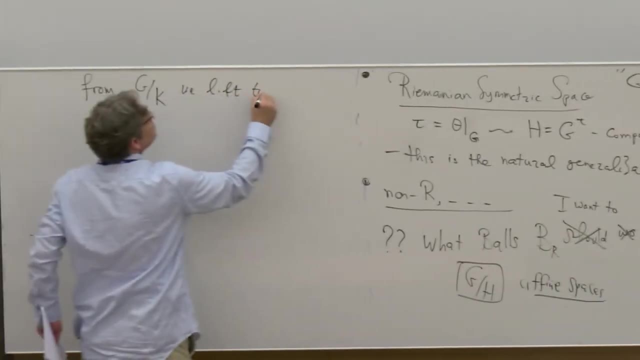 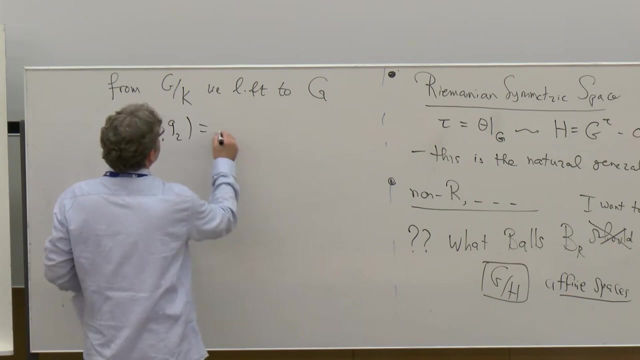 And that gives a way to construct balls. so let me just set this. So from G mod K we lift to G. The distance between G1 and G2 is just this d, G mod K of the cosets, And this allows us to define well- I want to use the word ball- 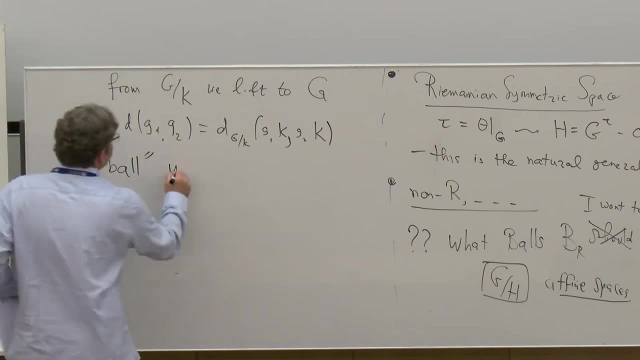 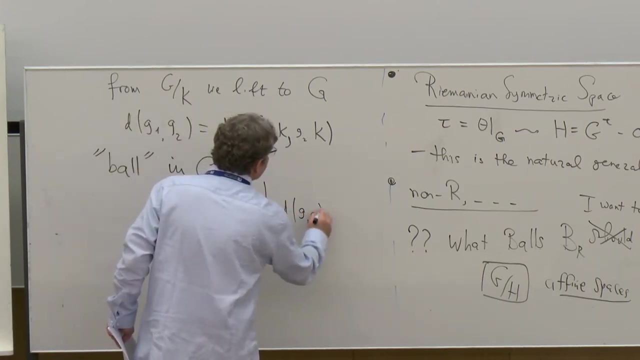 so we have this kind of a ball in G. This would be defined as follows: B R with G upstairs is the collections of G in G which satisfy that their distance from the unit is less than R. Okay So, and now I want to use projections. 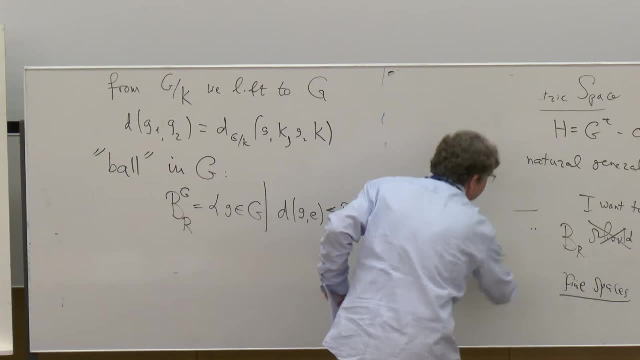 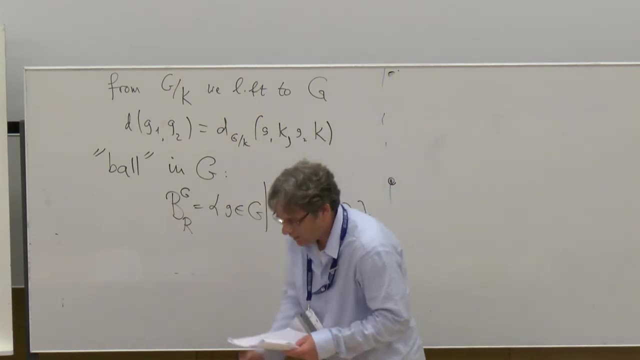 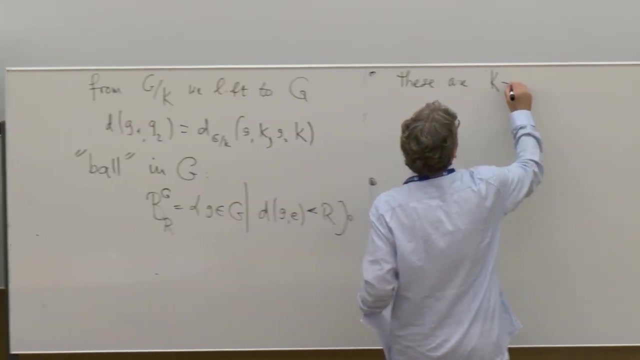 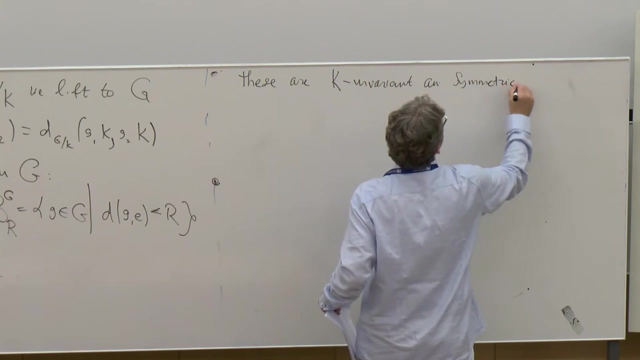 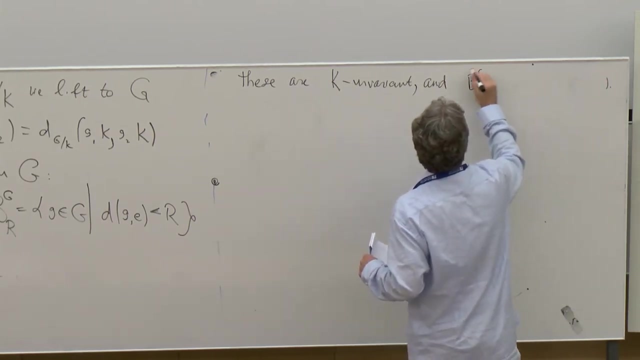 In order to to get to the space Z. So these are K invariant and symmetric. Symmetric in the sense that for inversion, respect to inversion- Okay, Maybe I will- K invariant and B R G inverse is equal to B R G. 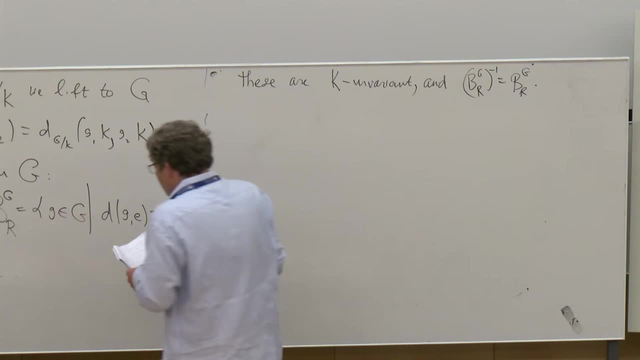 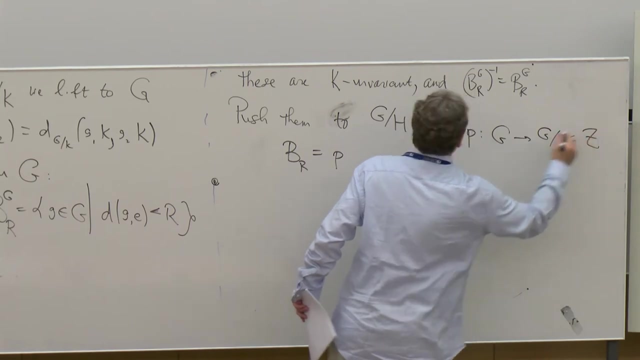 This is what I meant. Okay, And now we want to push them. put them. so I'm answering the question: what subsets in G mod H I want to study? Push them to G mod H And the result is the following: I get a subset. 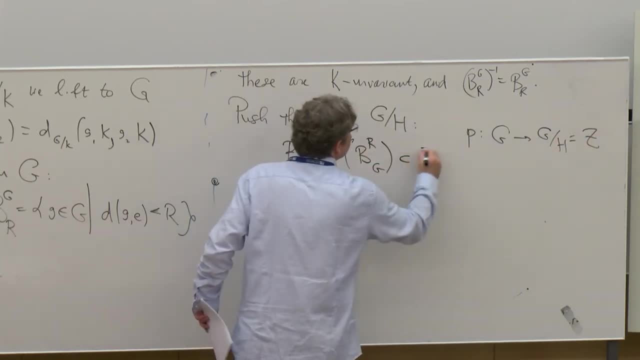 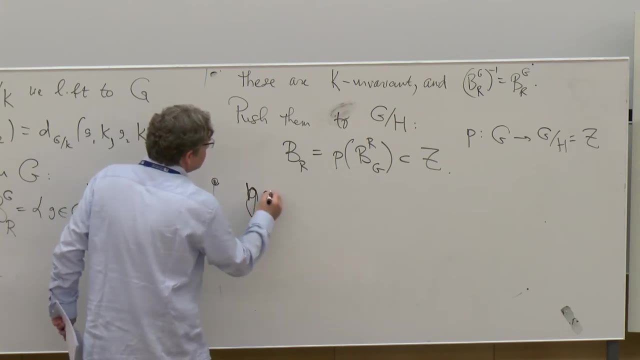 Which is the image under P of this ball, And this is what I call natural or geometric balls. Geometric balls in Z. Okay, How much time did I use to kind of organize 35 minutes? I have 35 minutes, Okay. 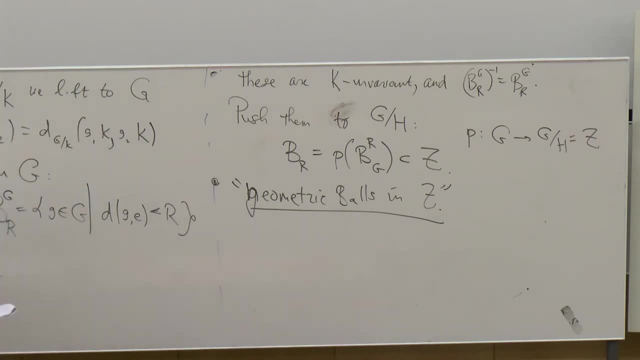 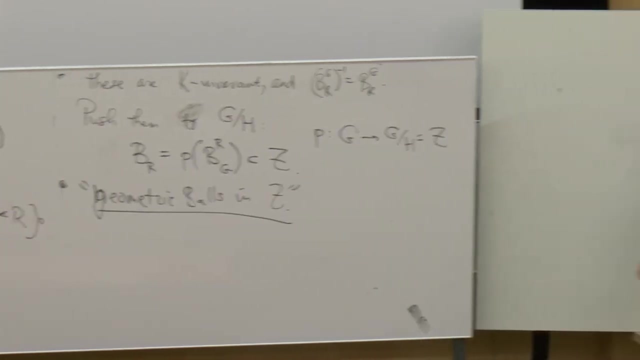 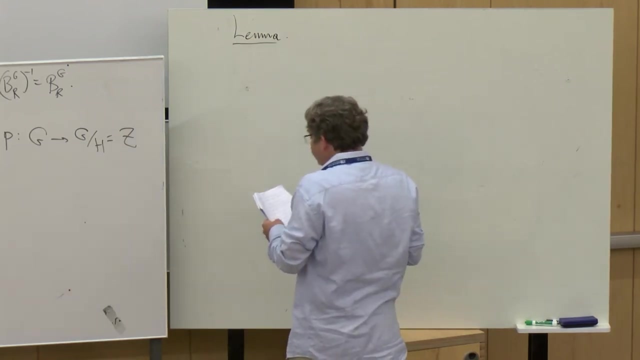 20. I have 25 minutes. Yes, Okay, Thank you, Okay. So one property which is kind of nice and maybe convince you that that these are interesting balls, is the following lemma, which is not difficult, but just I formulate it now: 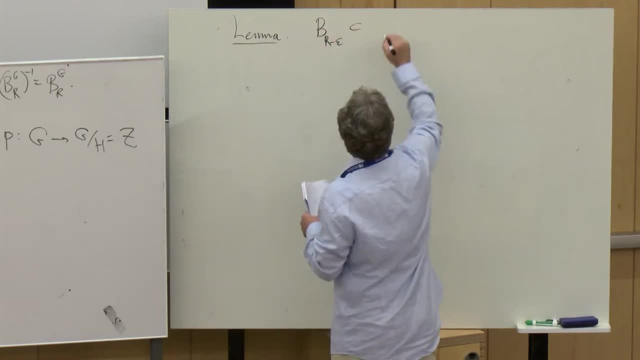 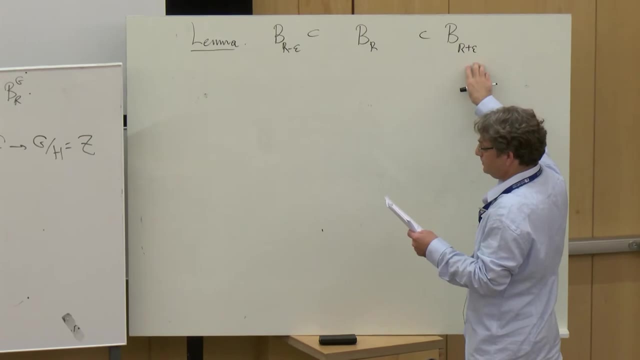 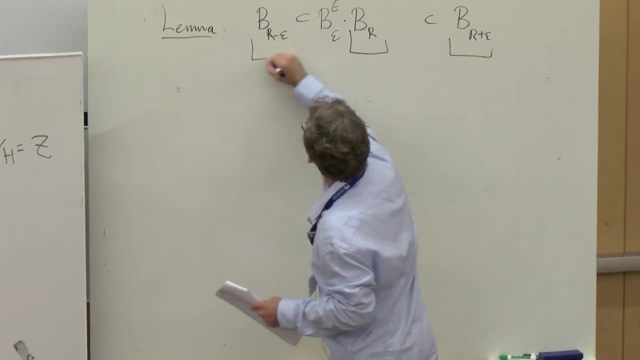 What happens when I perturb? when I perturb a ball, Mainly I look at a ball of slightly bigger radius. Then the statement is that if I act, so these guys belongs to Z. All these are Z objects. Subset of Z. 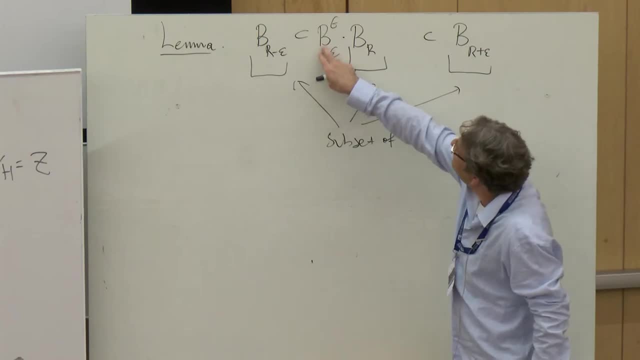 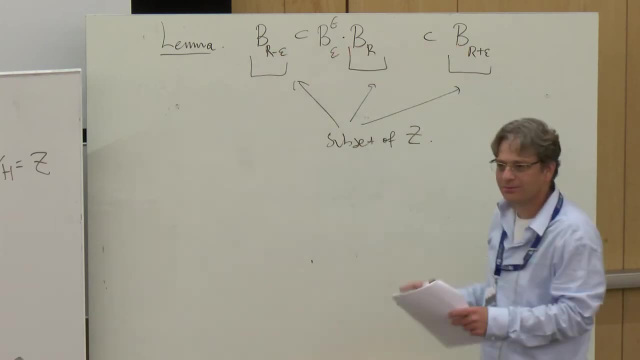 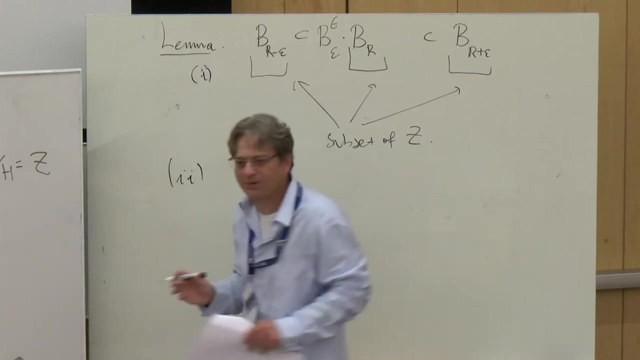 The statement is: if I act by some epsilon ball in G on the R ball in Z, then I don't go too far. Okay, This is one nice property And the second property- and I'm following these properties because these are essentially the only things- 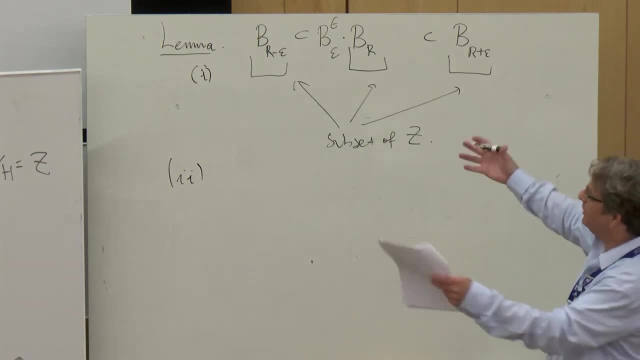 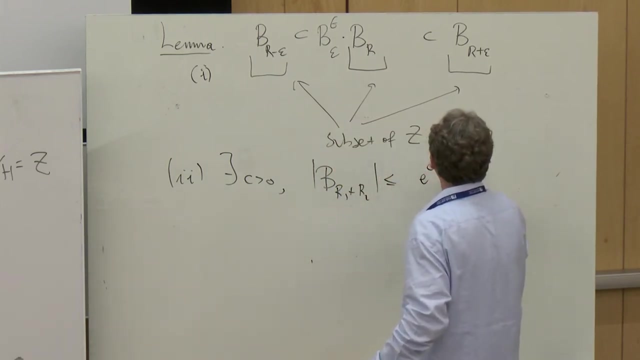 we are going to use in our arguments. So whenever you are in a setup with these properties, you should be happy There exists some positive C, So that V of R1- R2 is less than or equal than E to the power R1 times the volume of V of R2.. 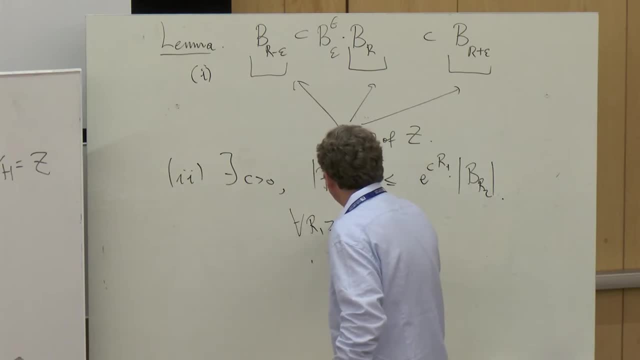 Okay, And this is valid, well, almost for every R1 and R2.. R1 is positive and R2 more equal than 1.. Okay, Okay, And naturally, if we, if you observe this construction, if you go back to G, mod K, 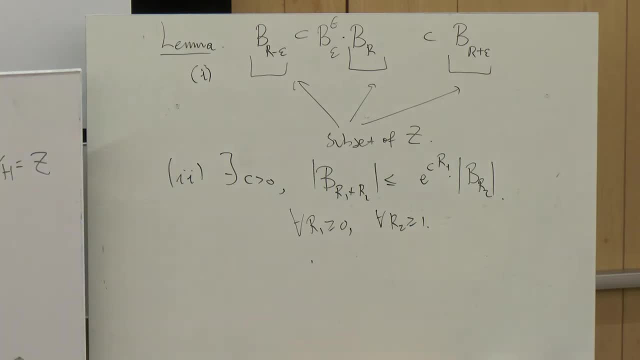 you will get the original balls that you had, So everything is consistent, Okay. So since my time is almost up, let me at least try to formulate some results. It will be difficult because I still have to introduce some notions, So I promised in my abstract: 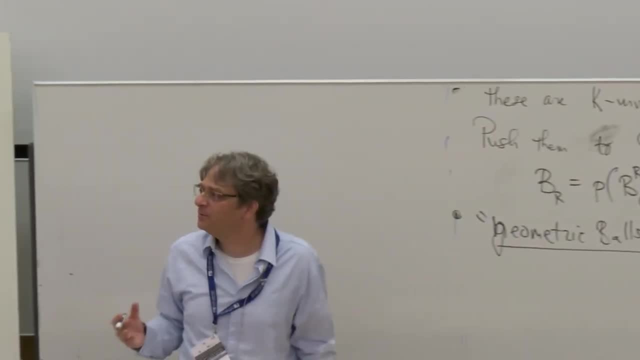 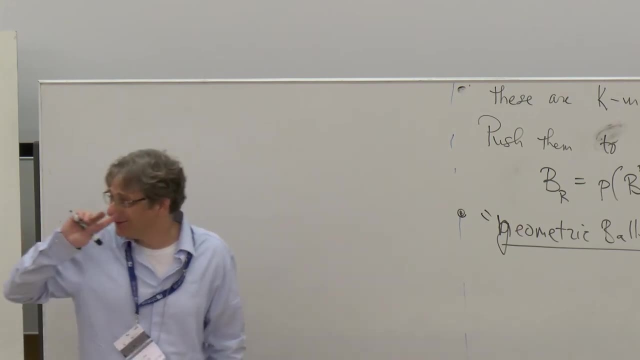 that I want to discuss counting on certain class of spherical spaces. So the person from which I learned this notion is sitting in the audience And the class is called Wavefront Spherical Varieties. So this is due to Secularidis and Venkatesh. 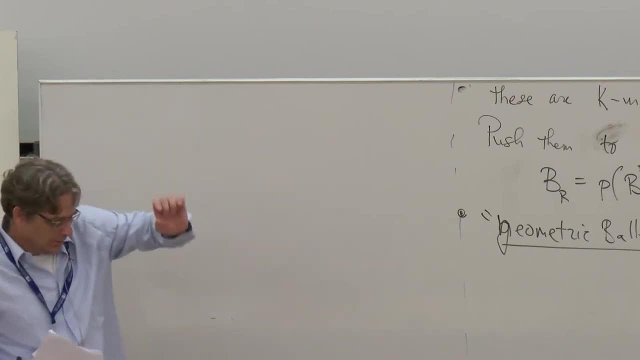 And earlier researchers introduced the notion of wave- wavefront as a geometric property. So it will be not so trivial for me to give you a definition in less than 20 minutes, But I will try at least to give you the gist of what. 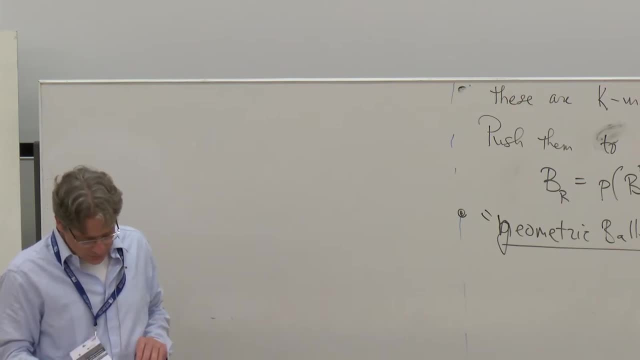 what is it all about and to formulate the theorem. So Maybe you can give a non-example. What? Maybe you can give a non-example I already gave? Ah, the non-example. Yeah, I will do that. So, first of all, 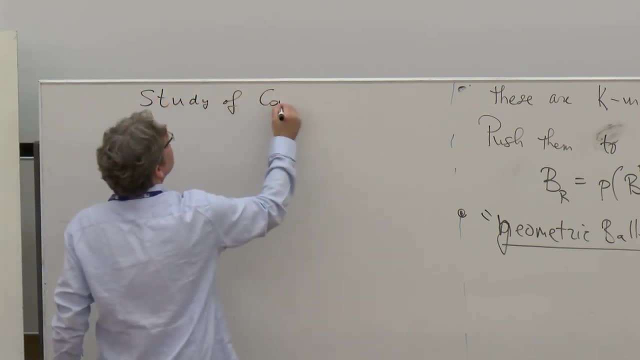 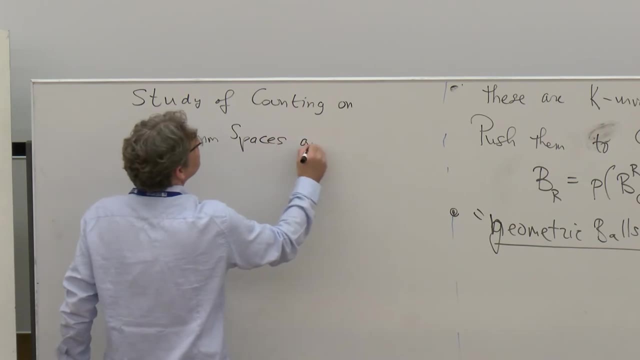 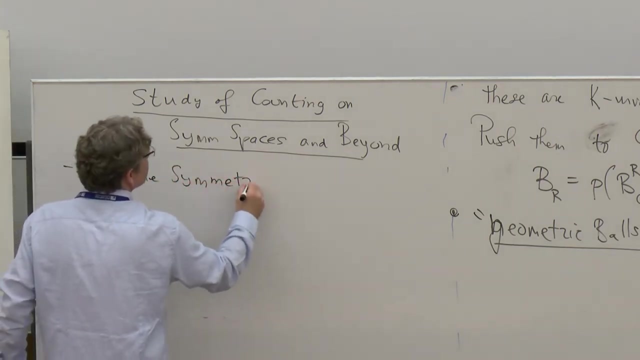 the study of counting on symmetric spaces and beyond Could be another title for the lecture. So, as I said, in the symmetric case- the symmetric case, I mean the following: yes, So g is a real reductive, as I said earlier. 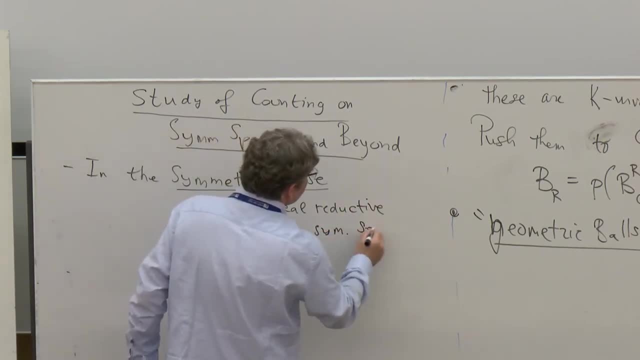 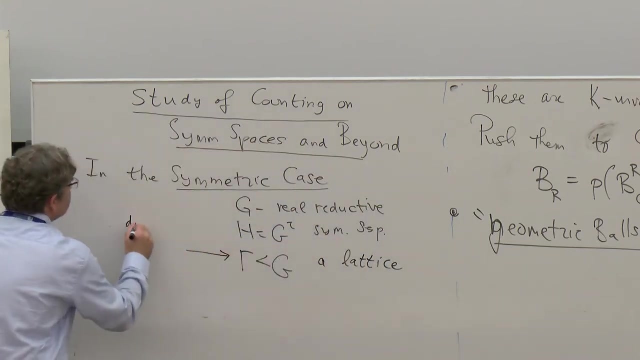 h is a symmetric subgroup And gamma in g is a lattice, which formally means that it's a discrete subgroup. discrete subgroup so that the volume of g mod gamma is less than infinity. Okay, Um, how? I will sequentially assume. 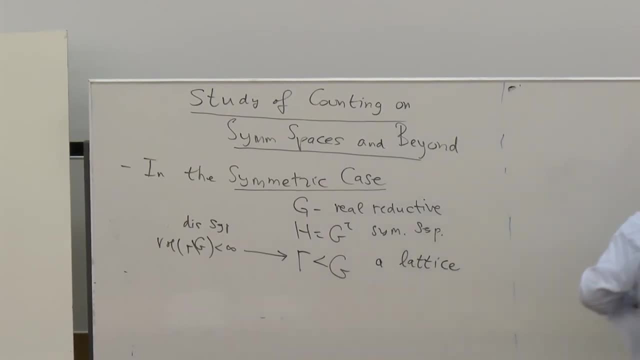 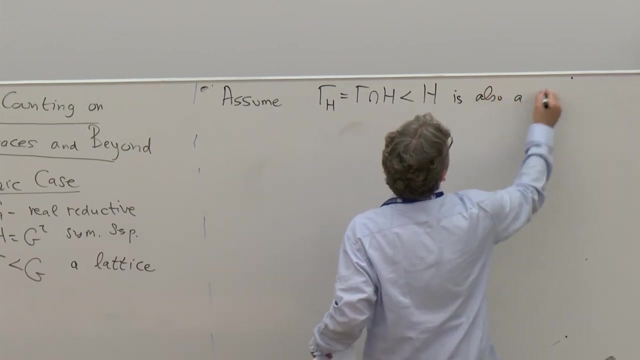 well, I will assume, and that assume, that h is kind of nice with respect to the situation. So this means that gamma h, which is gamma intersection h inside of h, is also a lattice. This is a natural assumption, Um. 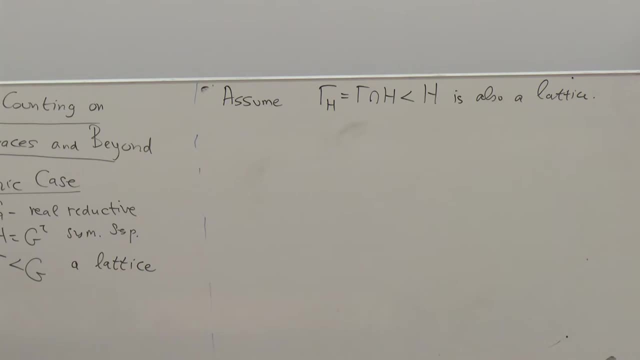 it turns out that this is the right setup to study things And in fact the volumes should be normalized. So volumes on g and h should be normalized so that, um, the volume of h mod gamma h is equal to. 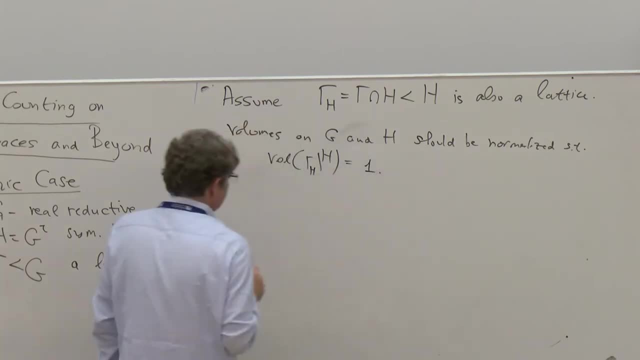 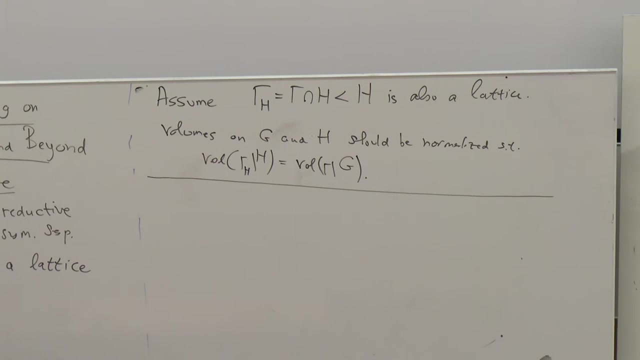 what? Probably to one. I'm not so happy. So maybe this, this is correct, Maybe this is better, Okay? Um so this, this gives natural measure on z which, as I said is, is unimodular anyway. 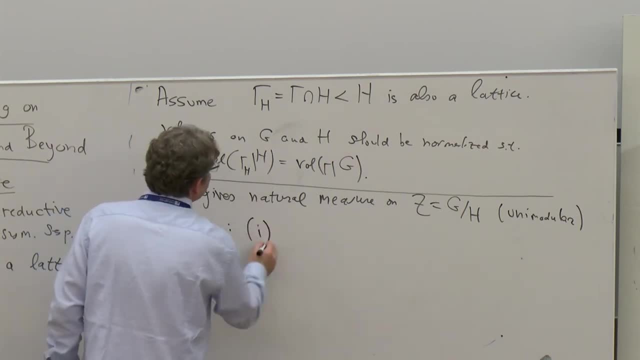 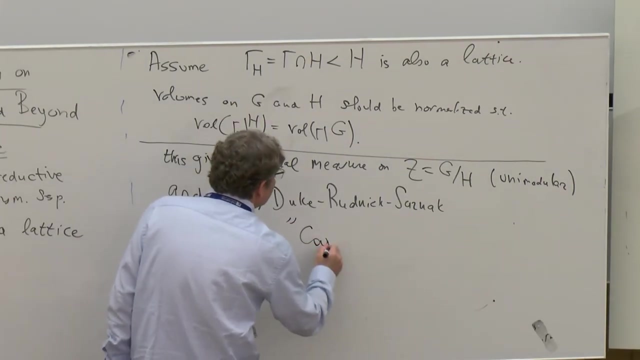 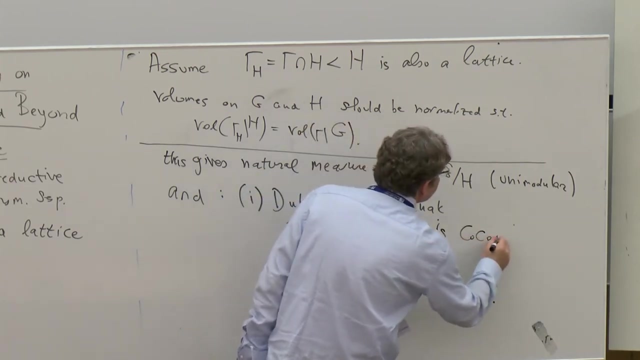 And there were two groups working on this subject. The first is uh Duke, Rudnick and Sarnak, And under some assumptions, under these assumptions um they proved counting if gamma is uh co-compact. 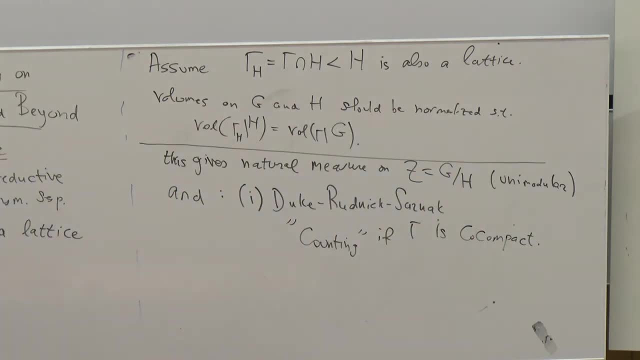 So if you further assume that not only the volume here is finite, but rather g mod gamma is compact, they have shown counting and they sketched it via how to do it in general. They never wrote it up because immediately. 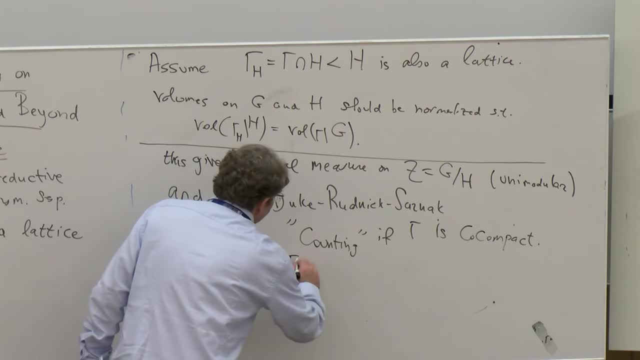 when the perprint was out and I'm kind of inventing the history- people here can tell me what really happened. Askin and McMullen gave a different proof in complete generality, using a different technique, So the technique of DRS. 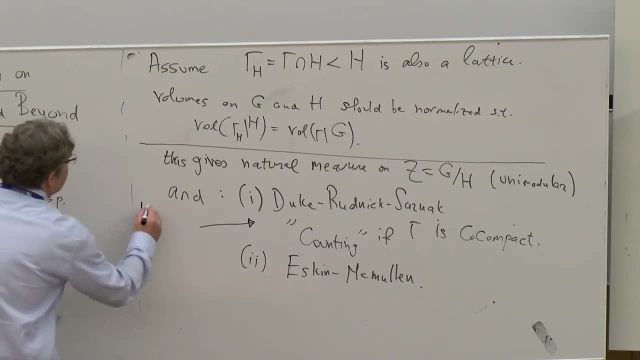 was, uh, based on harmonic analysis And in particular- okay, we'll say in particular- on what? and the technique of Askin and McMullen was based on something which is called the mixing lemma in Margulis' work, plus something that they felt. 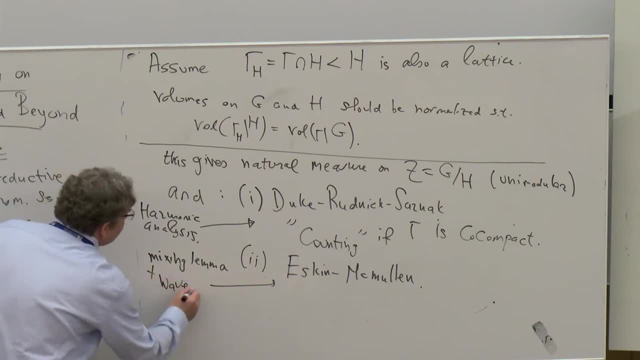 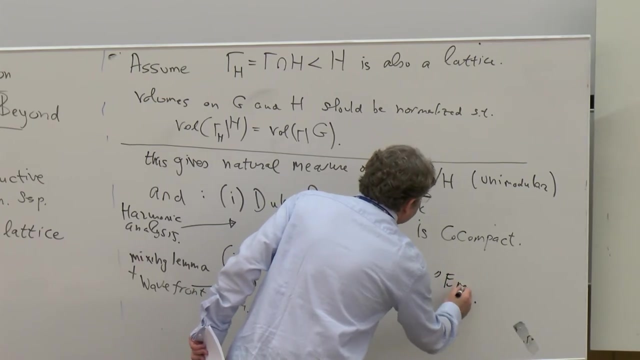 they found out and gave a name: It's the wavefront lemma. So they indeed formulated it. I will explain it in a second. and these two ingredients gave them a very general proof. So here we can also model. this is called. 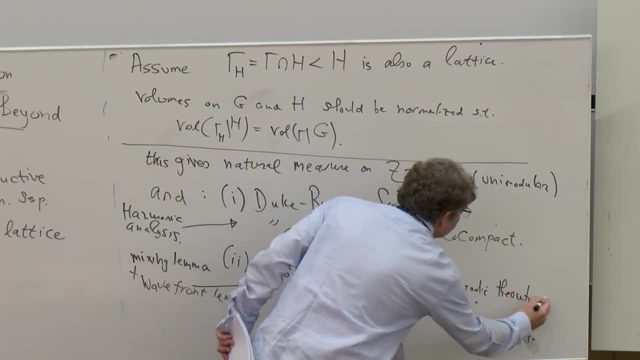 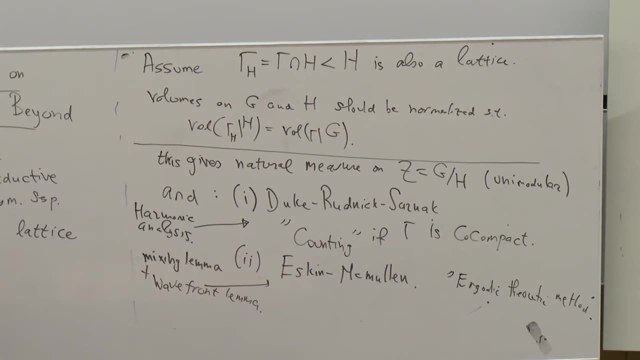 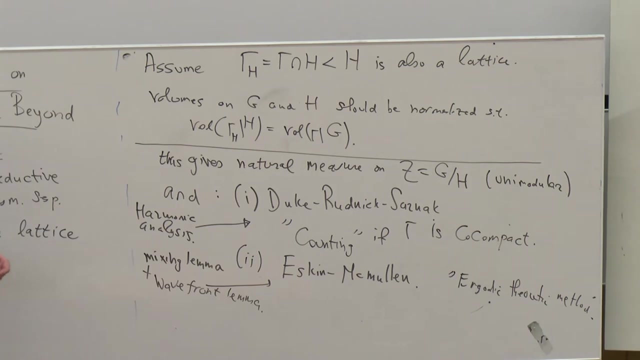 the Ergodic Theoretical Method. In these results there were no error terms. Later, Neveu and Gorodnik and a different group of Iho and Benoit were refining this technique and produced some error terms without explicit value of this S that I've written. 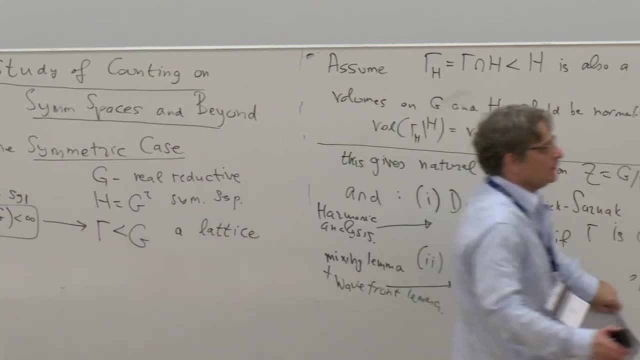 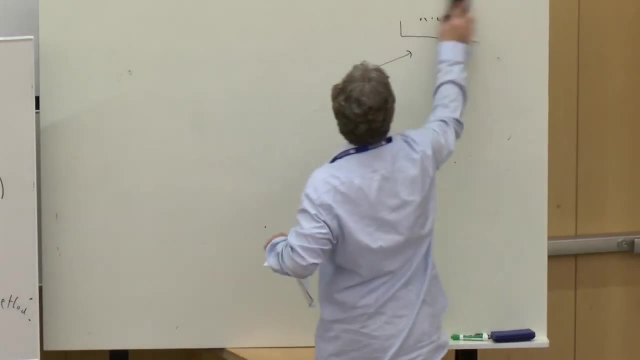 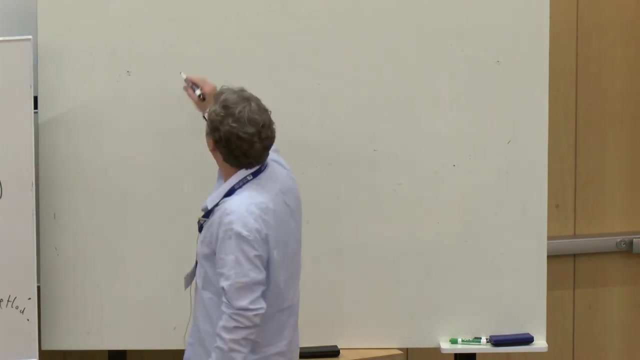 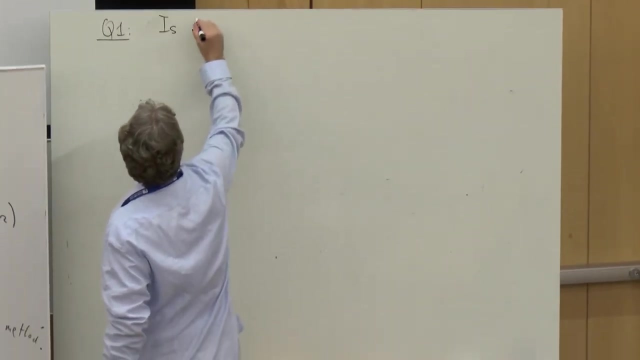 just ineffective error term. Okay. So the question remains. first of all, can one push the analytic method to get error terms and can one go beyond symmetric spaces? So question one: is it possible, is it possible, to use harmonic analysis? 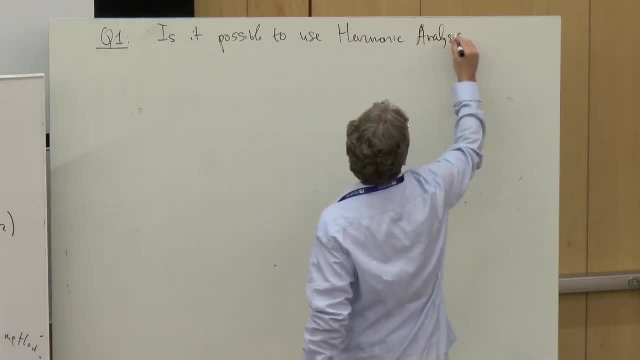 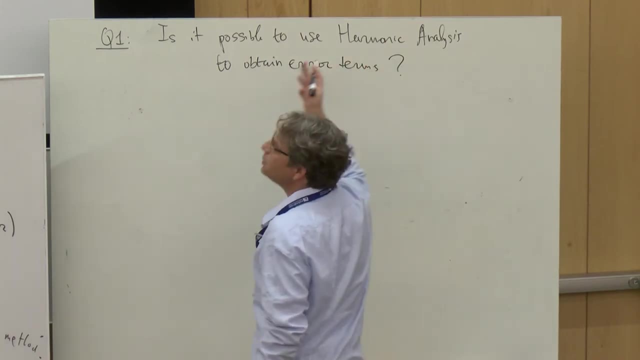 to obtain error terms. Of course, when I write it I feel it's a joke. What does it mean? Harmonic analysis was designed in order to produce error terms. When we're talking about Gauss circle problem, the first beating of the error term, 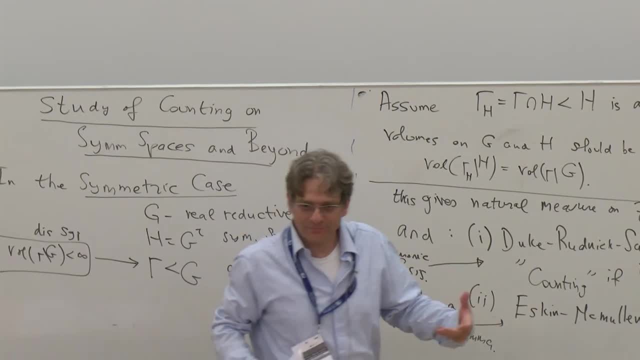 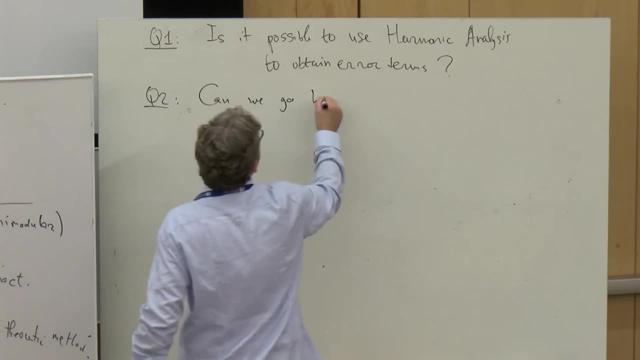 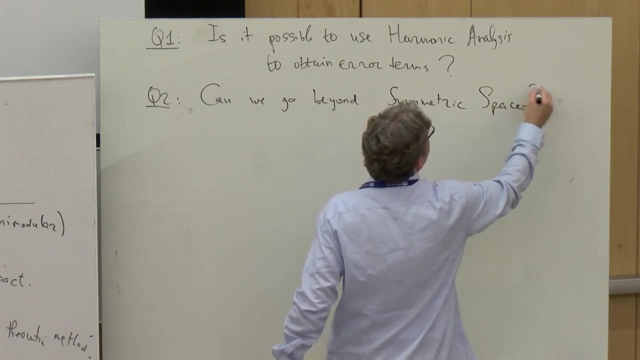 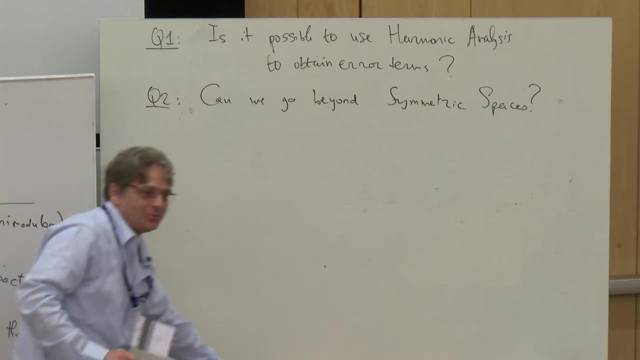 is based on Poisson summation formula. And the second question is: can we go beyond symmetric spaces? And the answers to these questions are sometimes So I would hope to say that always we can just produce a complete general, but we have partial results toward this. 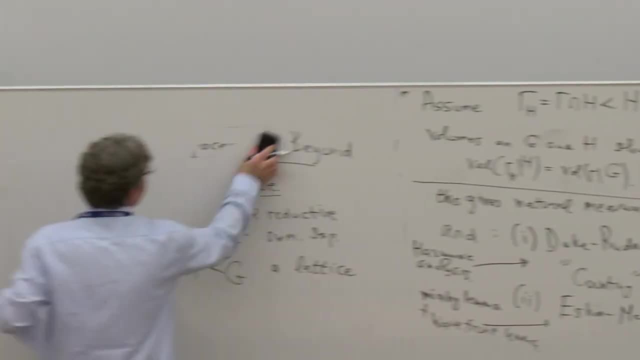 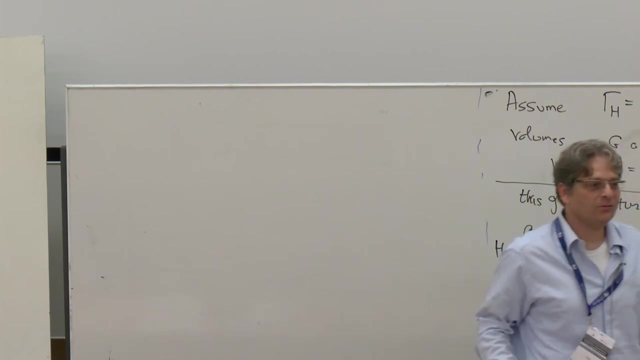 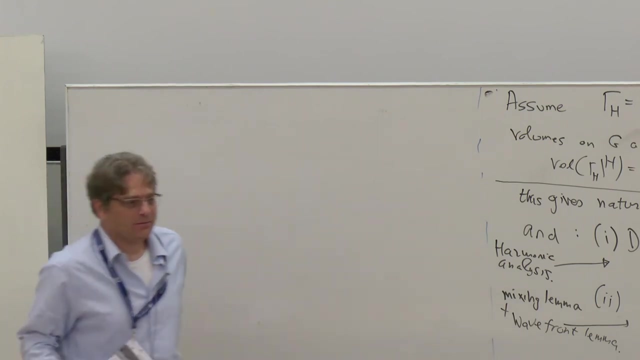 and I believe that actually this can be done in general. In a funny twist of events, our best result is obtained by adapting the Askin-McMullen method, Namely when we set up the approach to study the problem using harmonic analysis. 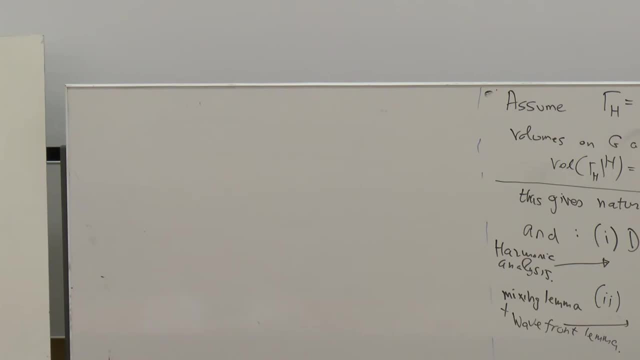 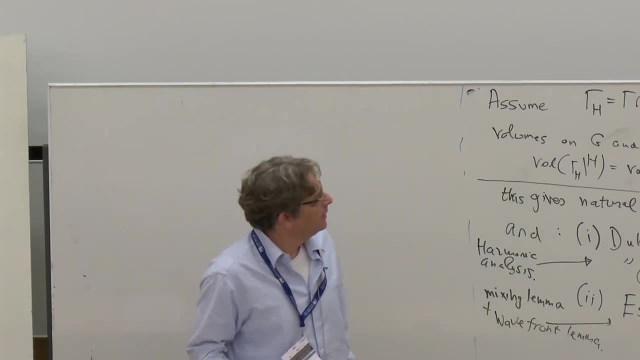 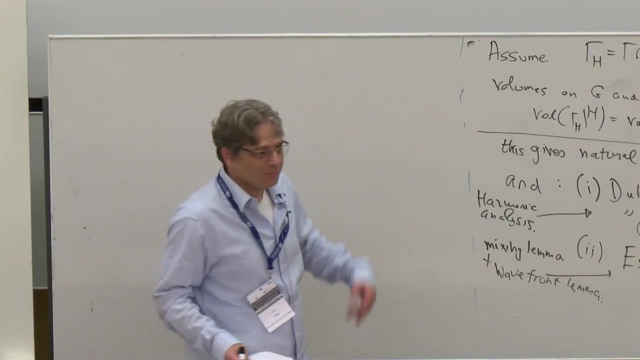 we wanted to invoke some tools from harmonic analysis, some spherically spherical varieties, in particular on wavefront spherical varieties, which is a subclass, And we realized that we can actually prove a version of the wavefront lemma in that case. So finally, maybe theorem one: 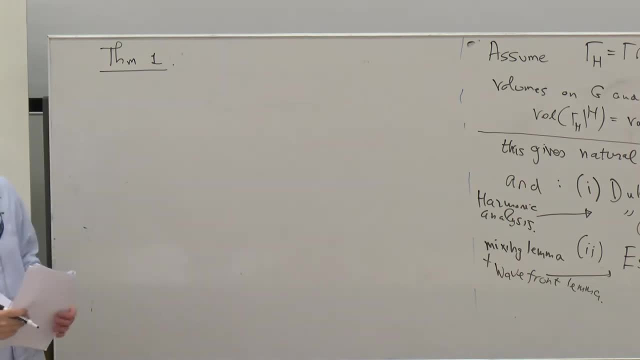 which is not the best result that we have, but it's at least easy to formulate for wavefront spherical varieties. So varieties we have counting Okay, so I will need to say something about this concept, So um. 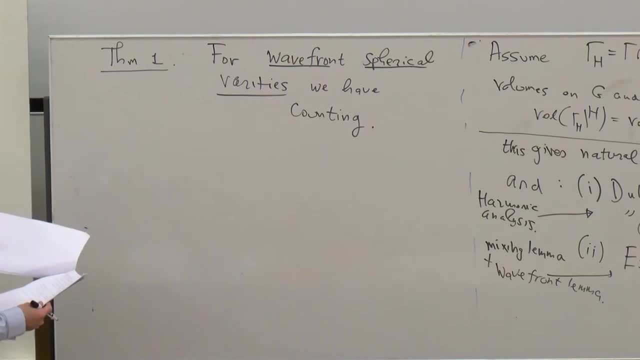 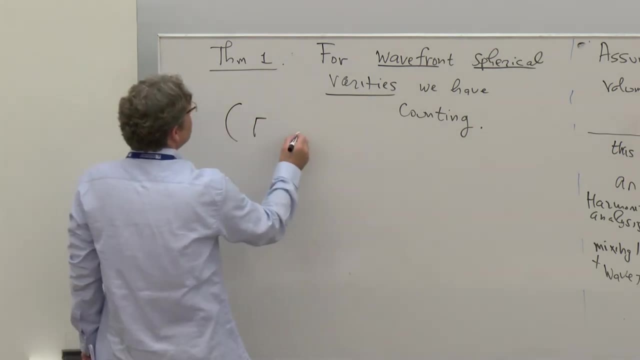 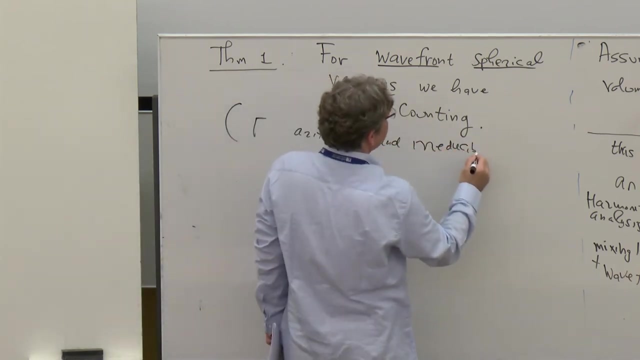 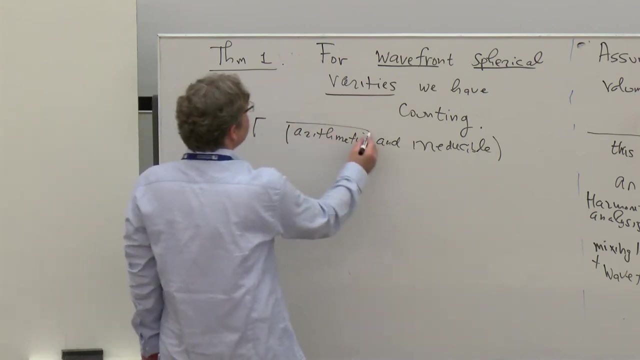 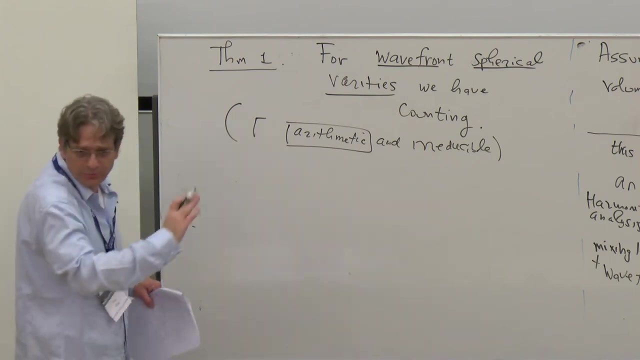 And okay, so no, I apologize, we don't need that. 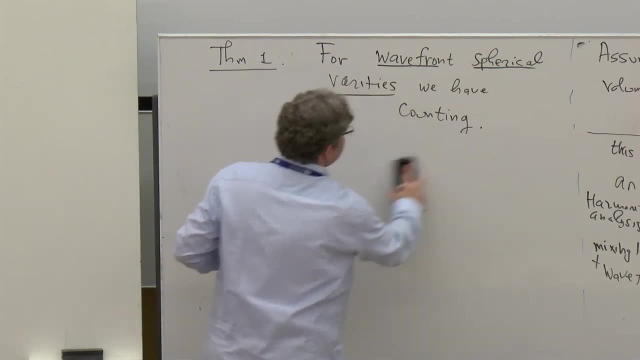 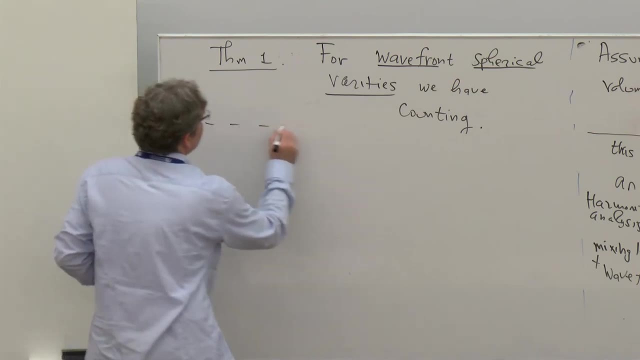 I'm sorry, I got confused. No, we don't need that. Sorry, I apologize For the counting itself. we don't need it. Okay, let me say something about spherical varieties and about spherical wavefront spherical varieties, and then I will formulate the second theorem. 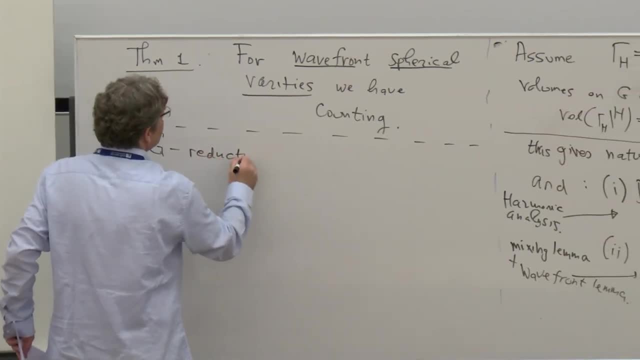 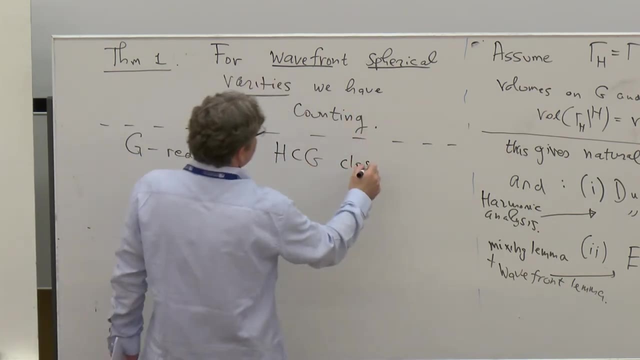 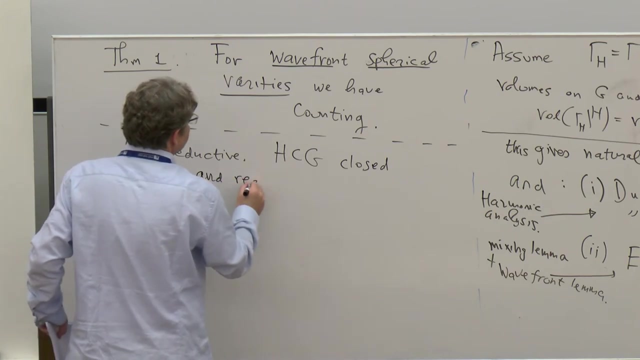 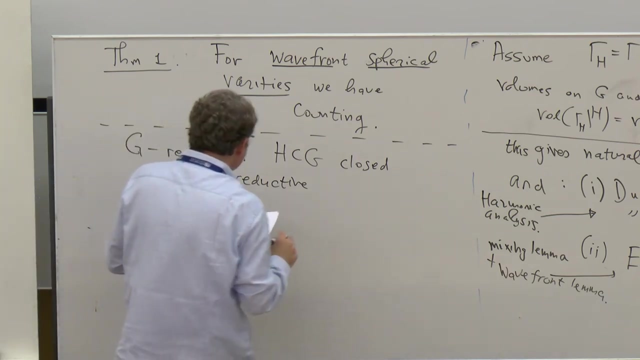 So suppose that G is reductive and H in G, I will assume, is closed. so closed and reductive and for safety. but people will not, okay, that's okay. So I give kind of definitions. 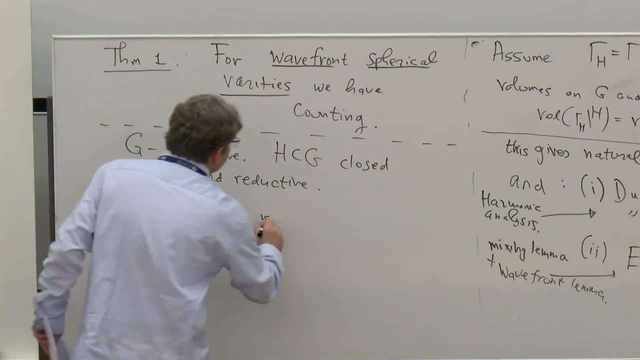 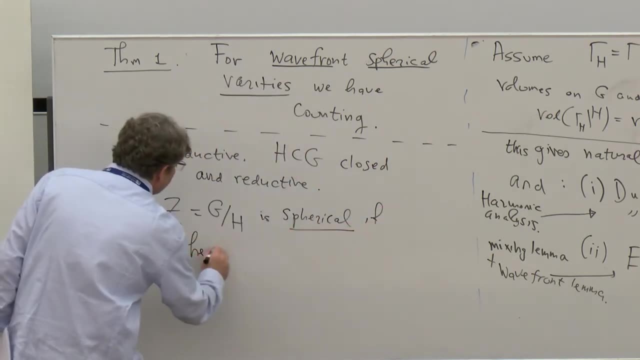 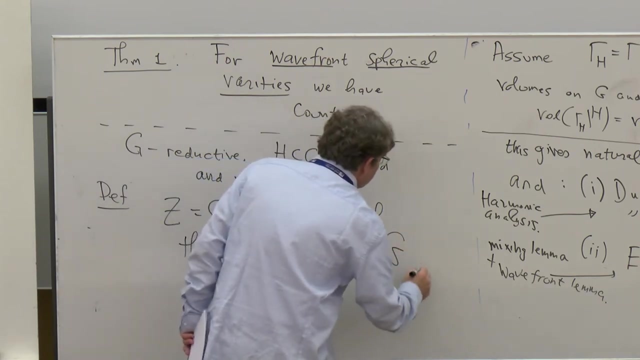 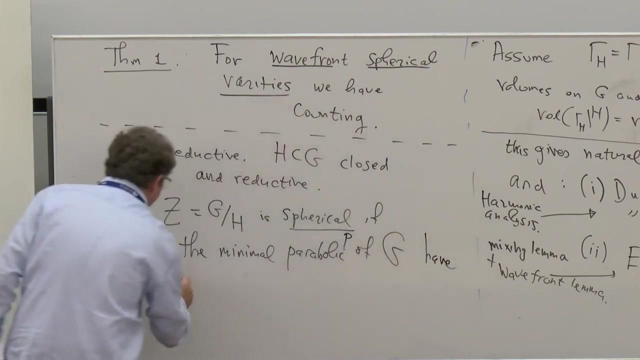 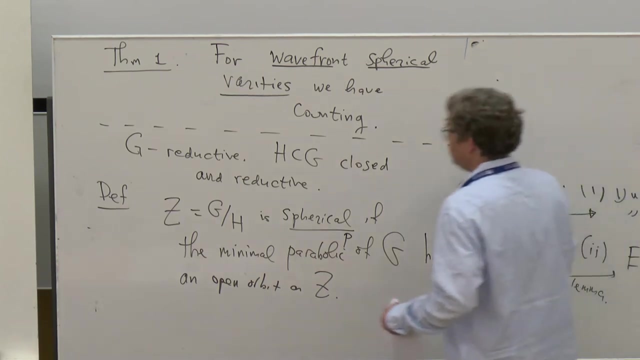 So I said the Z is spherical. if the minimal parabolic of G, minimal parabolic P of G have an open orbit on Z, This implies that it has finitely many orbits. and what Rereducted groups. There's a gamma, so it's called real state. 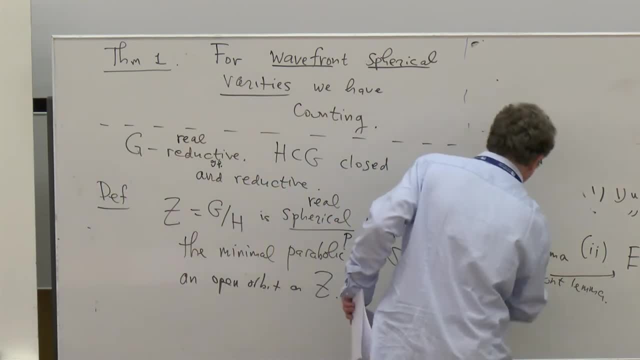 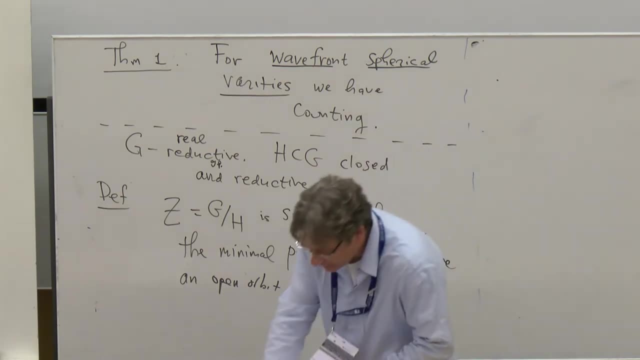 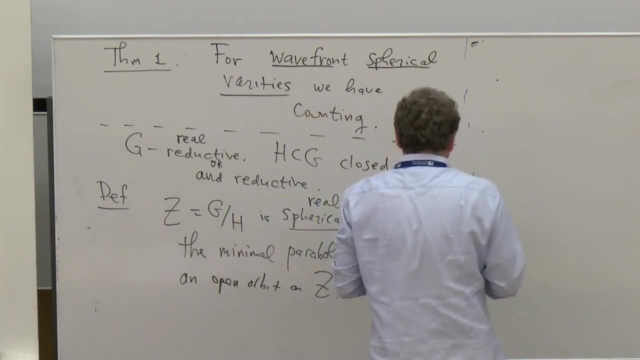 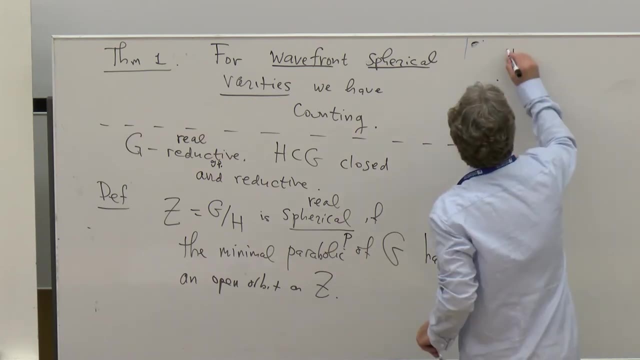 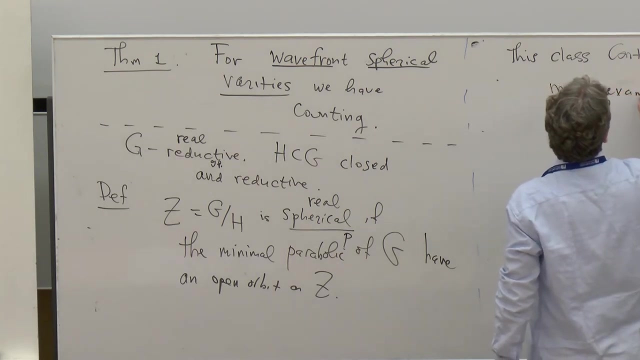 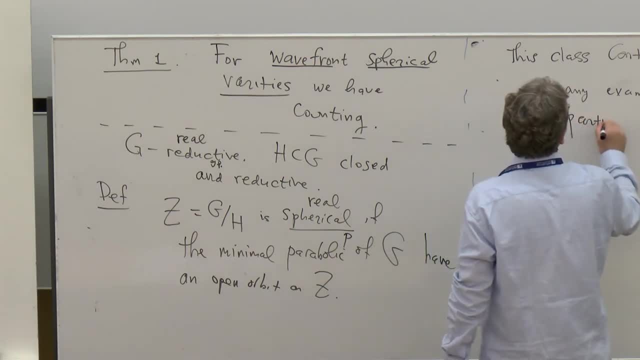 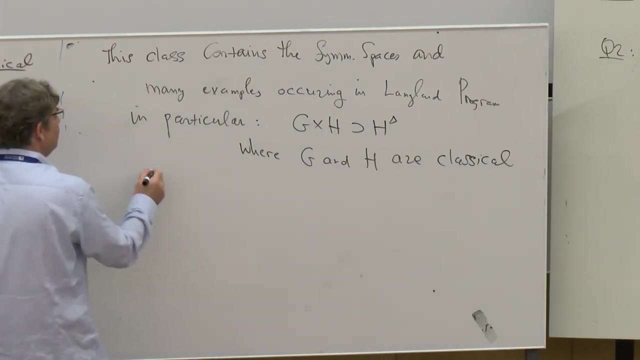 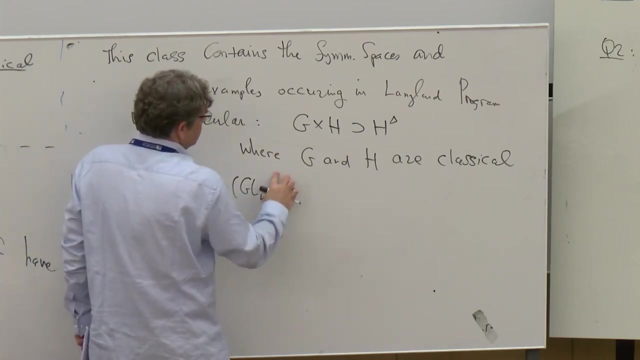 In particular the examples like g times h, where h is diagonally embedded, where g and h are classical. So I'm not saying any g and h will do, but for example, if you take gh to be gln plus 1 gln, then it will work. How many more? I'm focusing now on reductive. 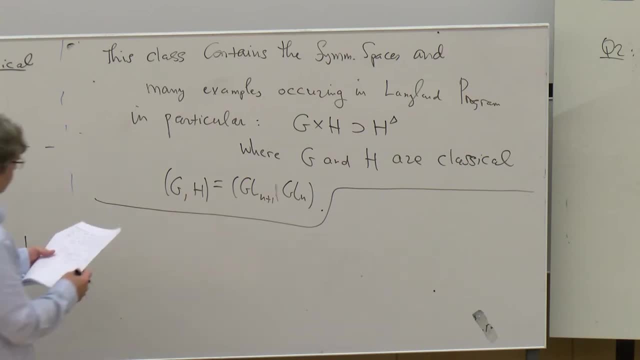 examples, Maybe some more. Okay, More example which are more in line with Savin's lecture. So S043 and a certain form of g2, which is denoted by g21.. Okay, This is as far as I, And then the example I said. 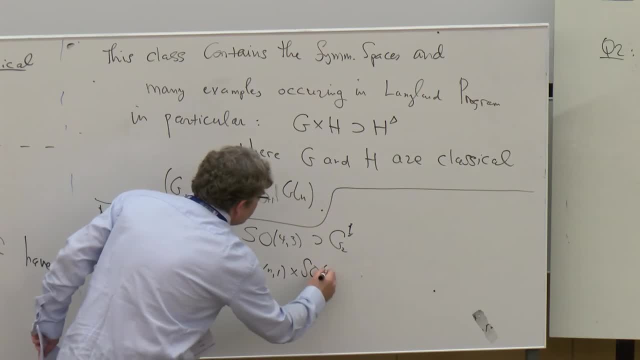 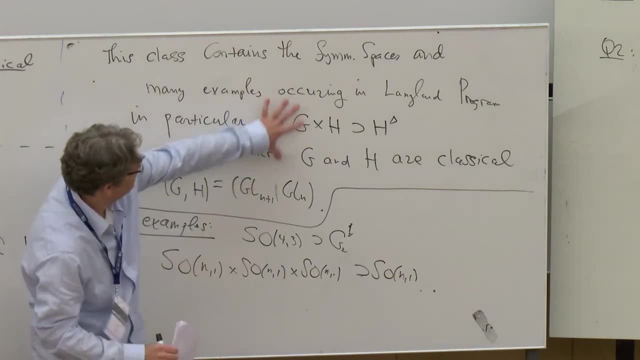 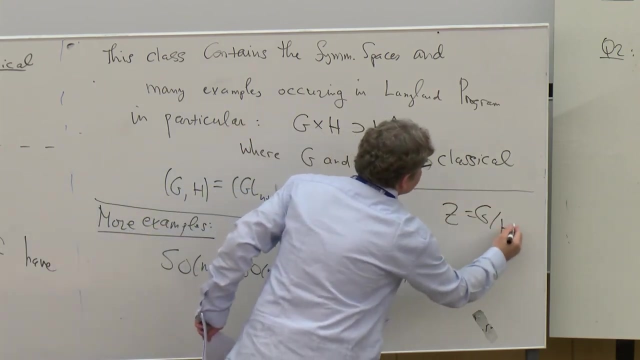 earlier SON1, triple product With SON1 embedded. Okay, So here I don't mean this part, This is just, This is g and this is h, and the space is g mod h. Okay, Okay. So I think I'm now almost ready to formulate. 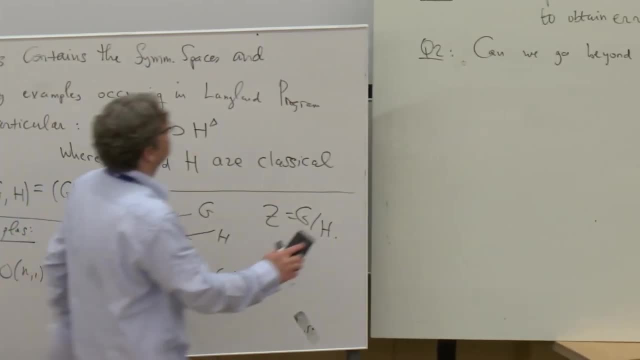 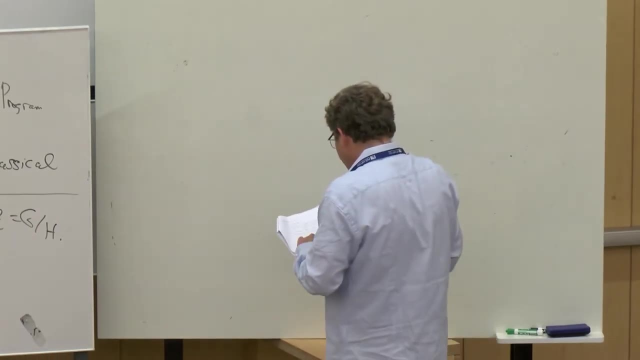 the main result: Okay, Okay, Okay, Okay, Okay, Okay, Let's see. now We say there's a test here. Okay, Again, the name of. Well, we can't say what a test this is, because we want to know the facts. 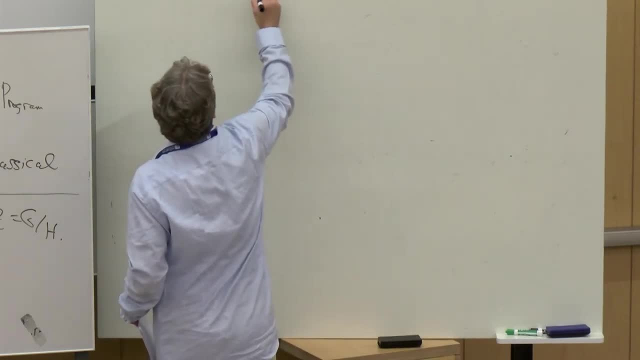 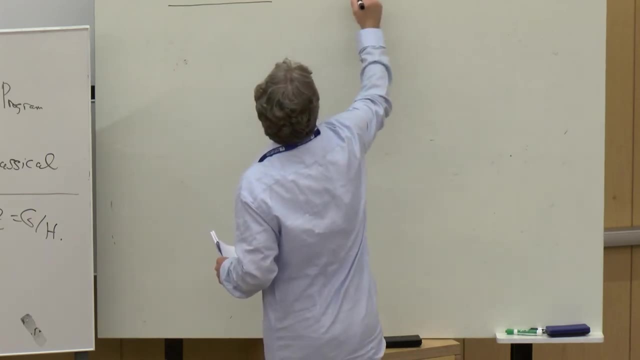 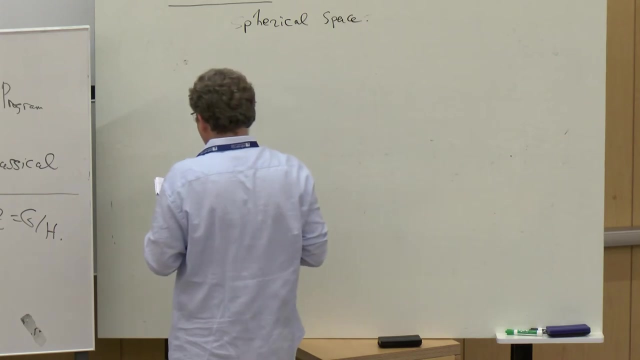 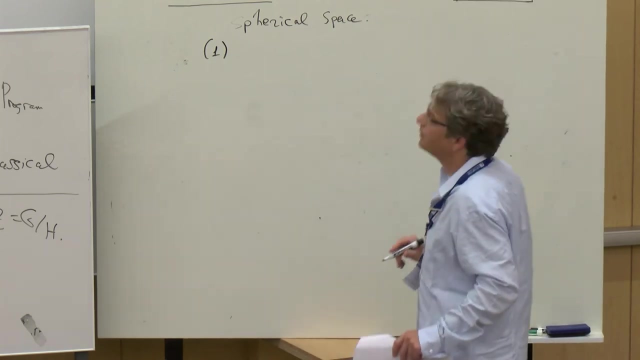 Okay, And the main result? Okay, And again, this name of wavefront will enter there. I will say something about it in a second. So let z be waveform spherical space. Okay, and I will make few assumptions. so okay, first, without any assumptions. 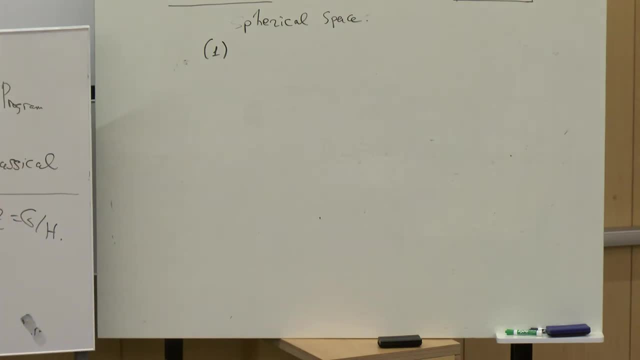 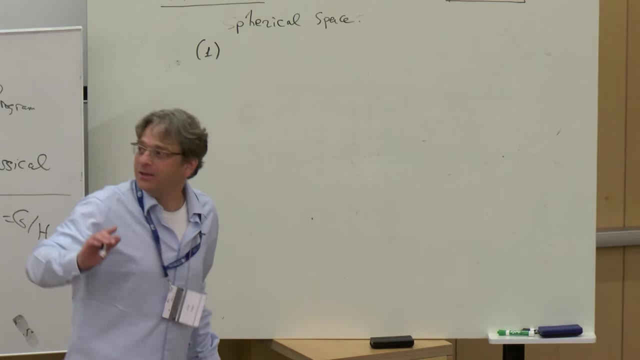 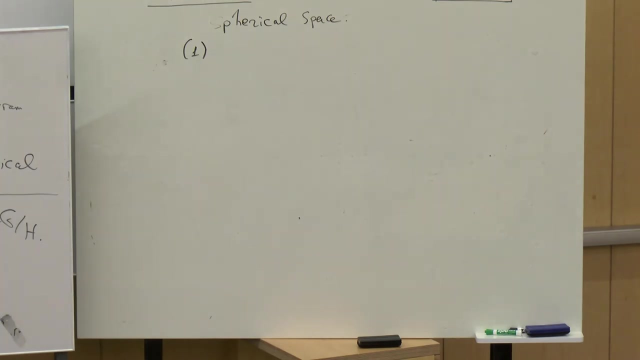 any symmetric is such, SON1 triple product is such. I can give you a list. you will be unhappy if I will give it to you, but I will describe it. okay, I will describe the main property which. so the main property geometrically is that you know. so for symmetric space, 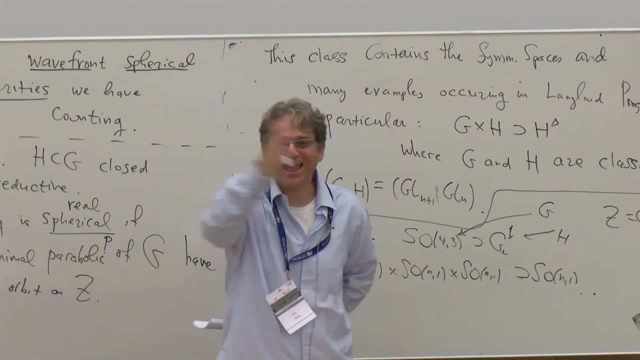 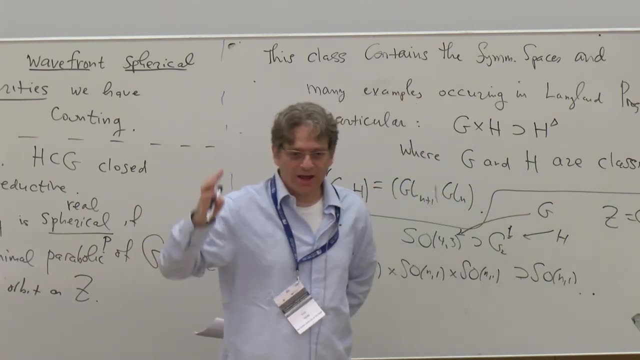 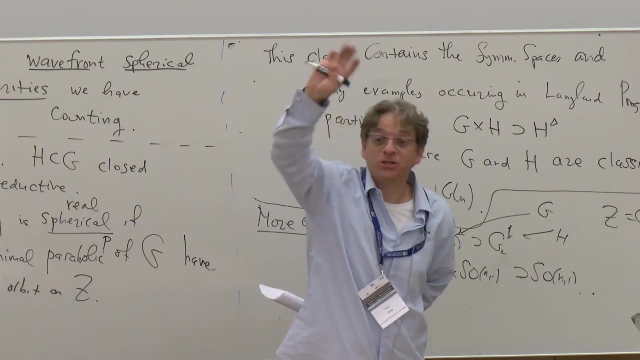 you have an analog of the polar decomposition k a h, k a k decomposition. for symmetric space a similar decomposition exists. you can write g as h, times a, times k, with a proper a. what you have to do is to take the two different decomposition of the Lie algebra. 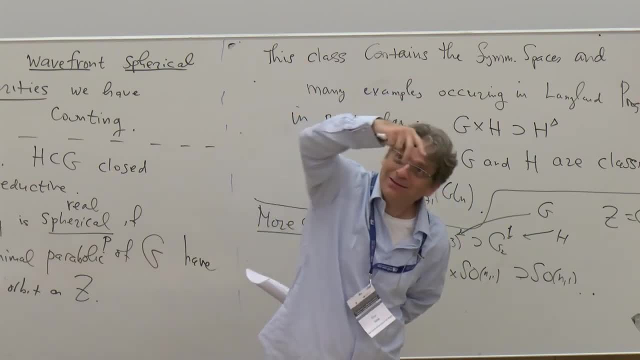 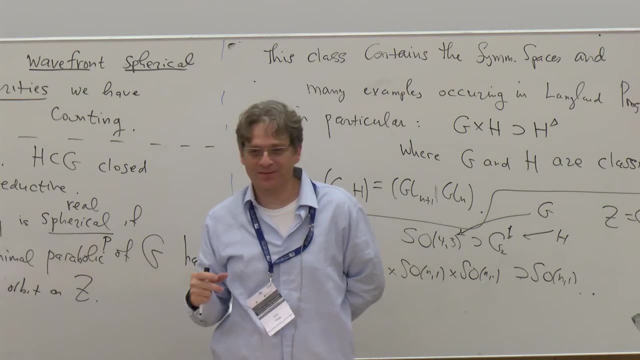 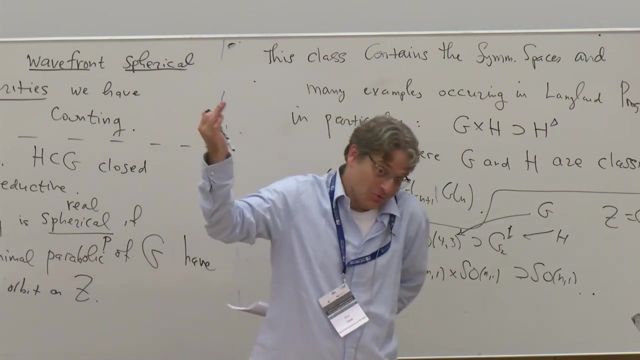 the k plus p decomposition and the h plus q, and then you intersect the p and the q and you take a maximal abelian subspace. this gives you an abelian subgroup, okay, and this gives you a decomposition which is an analog of k a k. just a second. 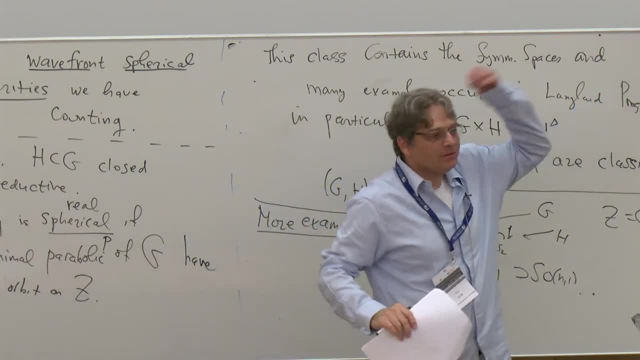 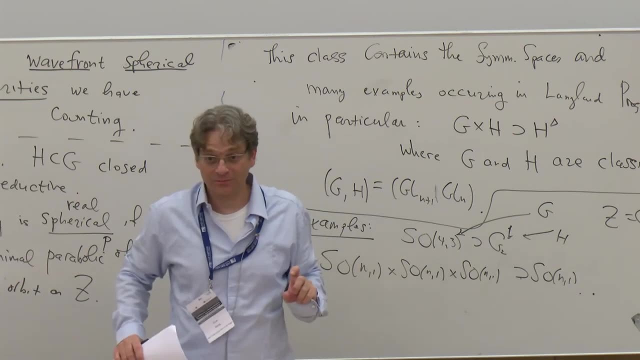 this. you followed a wayfron space. a spherical space is a space for which such a polar decomposition exists and this can be described in terms of its roots. so one can do this right away. you can write it to each other today and do it very easily. 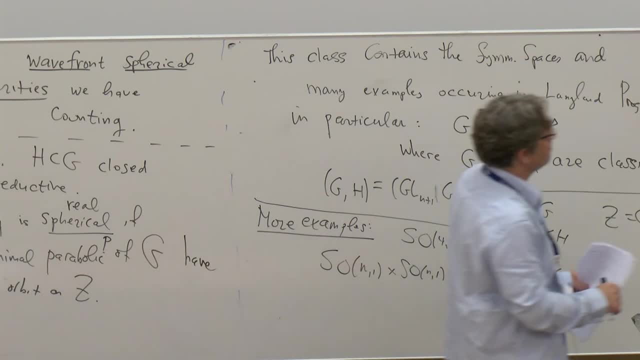 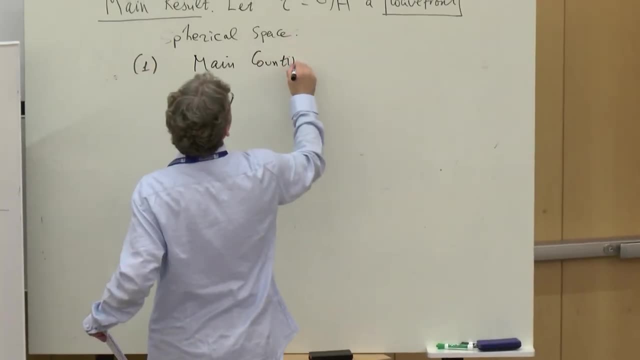 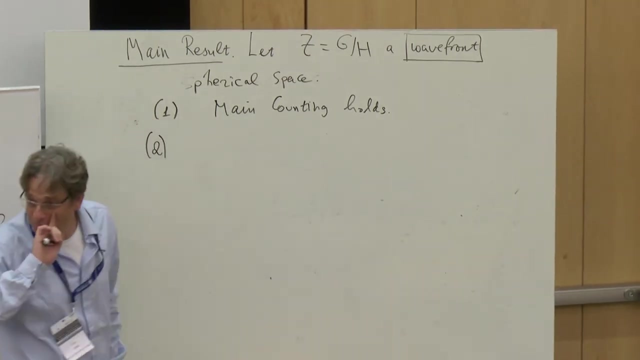 you can write it to each other and do it very easily, produce a list in a second. so the theorem main counting holds. so this you already seen. this was theorem one and second. assume further. this is what I made a mistake for the next three. so this is the main counting. this means that the 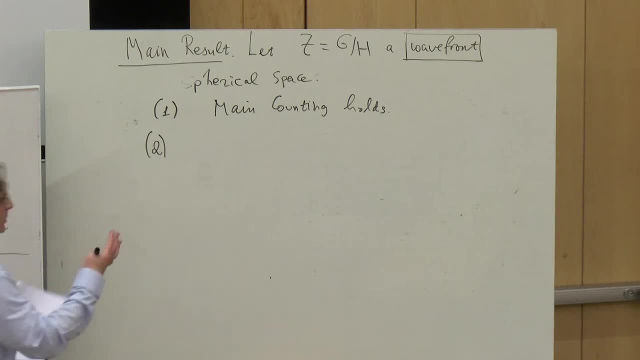 number of lattice points is correct. in order to get error term we need further assumptions. so we need to assume the g is semi-simple and no compact factors. all these are kind of small technical things. otherwise this, the result, is kind of not working. gamma should be arithmetic, and this I think we can. 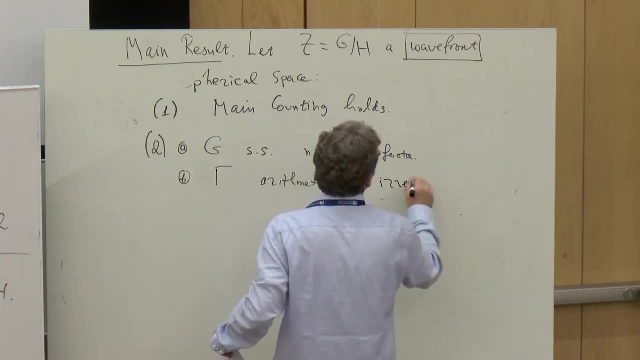 probably eliminate and irreducible. and finally, and this is our, at the moment, main burden, this has to be compact and this is probably also possible to eliminate. then there exists what I've written before. there exists a positive number which is completely explicit and ugly in terms of the parameter of the space, z. 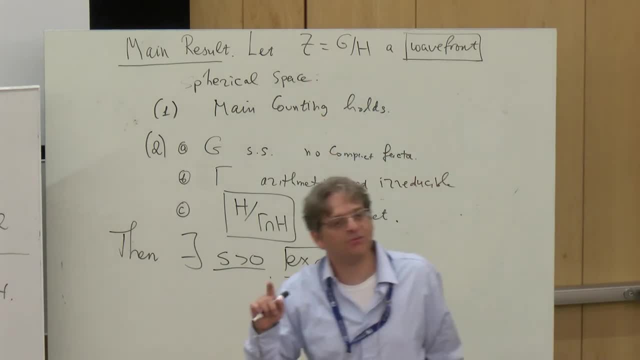 and in terms of the properties of gamma- and I will elaborate on that in a second- such that the error is less than or equal than a constant times the volume of the ball to the minus s. now what is that different than the ineffective result? from your perspective, it's the same. 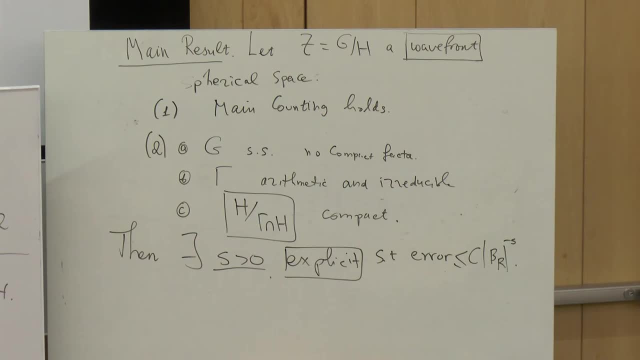 because I have not written a formula. it's ineffective, but this is a matter of trust- or going to the archive. we can write a formula for s, which involves what we call the rank of the spherical space, which involves the dimension of the spaces involved and, in particular, a parameter. 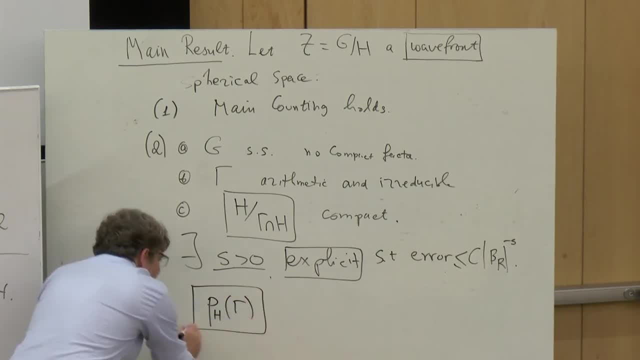 which we denote pH gamma and was studied by previous researchers, and this is actually the reason I'm mentioning, because it's a key to, or somehow the beginning of the argument in some sense. So the approach to this result is through analysis of matrix coefficients, So analysis of generalized matrix coefficients. 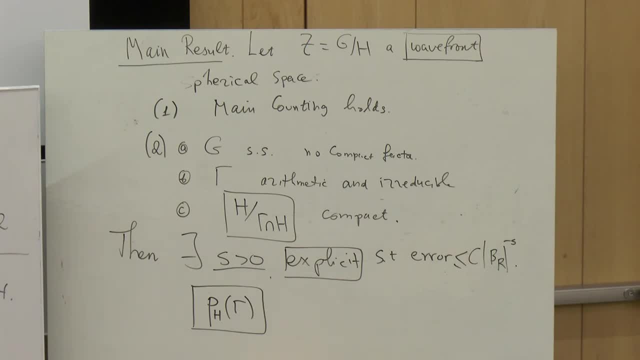 of unitary irreducible representations of G which are gamma-automorphic. So this exponent, pH gamma, looks at the spherical unitary dual of G and considers within matrix coefficients which are related to H-distinguished automorphic forms. And you look at the exponent, the LP exponent. 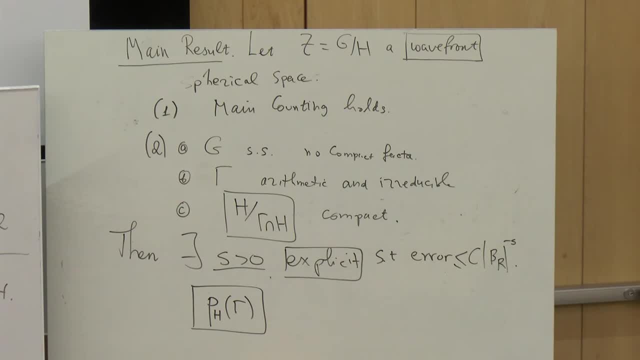 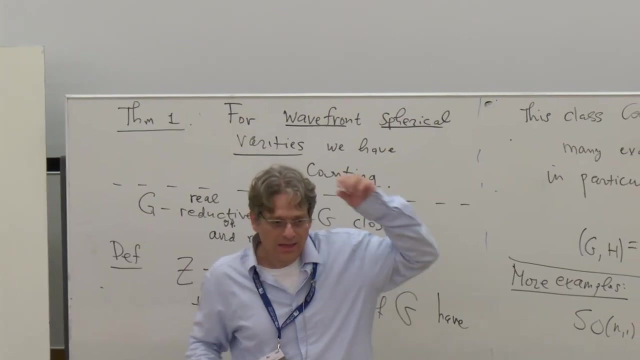 where these matrix coefficients belong to. Now, what am I talking? What am I talking about? So it all began with Roger. he's here. So the matrix coefficient of a unitary representation, if it's a non-trivial one, decay at infinity. 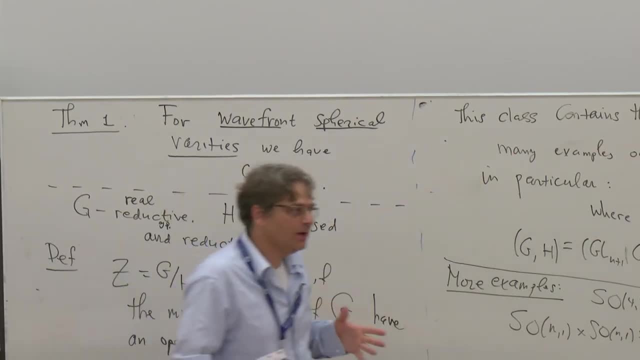 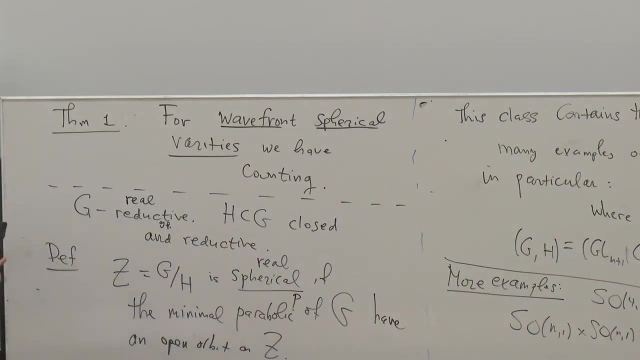 And in some sense the entire study began when we studied the following problem. So can I erase this? How much time do I have? Five minutes, Five minutes. So we'll just not give a proof of anything, but motivate our approach. 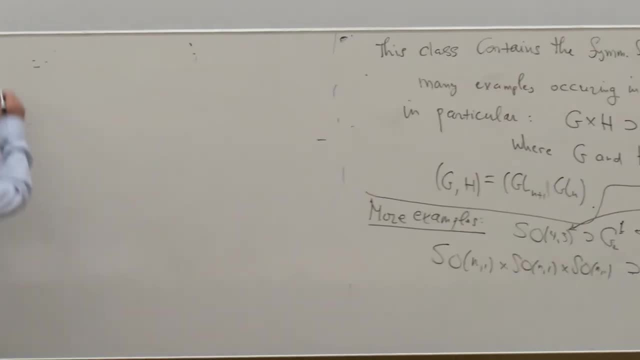 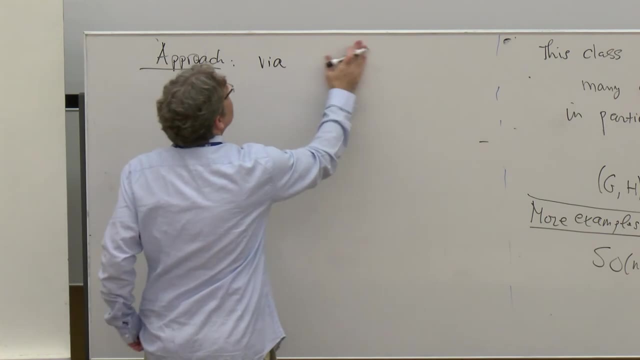 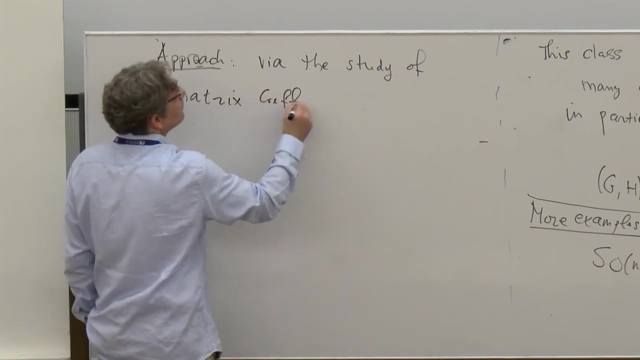 So approach via the study of matrix coefficients. So what we're going to do is we're going to look at the decay of unitary representations of G and, I should say, generalized matrix coefficients. So there are a few things in the soup. Maybe the most important thing is: 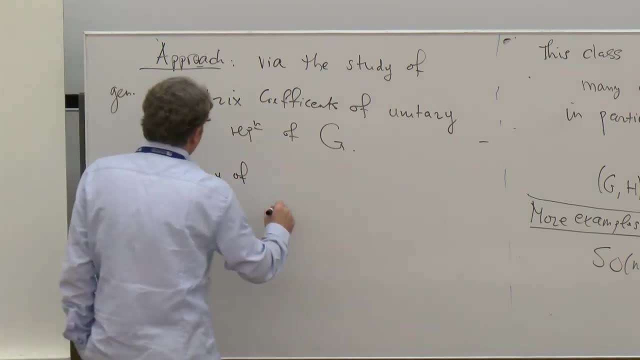 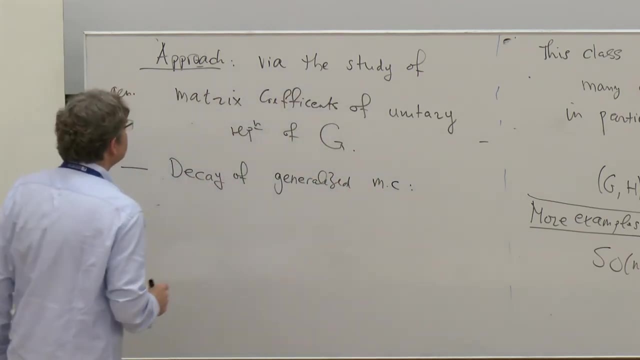 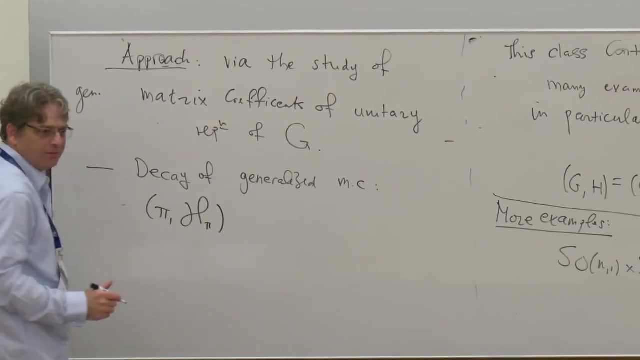 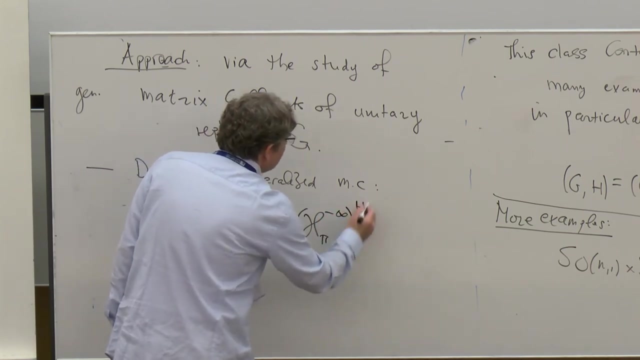 decay of generalized matrix coefficients. Let me explain what am I talking about. So suppose we have a unitary representation, pi, which is afforded on a unitary Hilbert space, h pi. And suppose we take a linear functional which is h invariant. 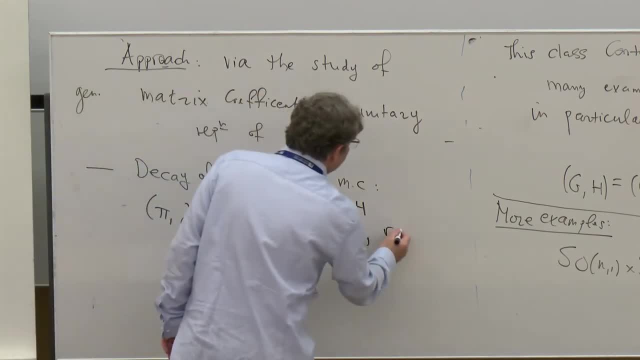 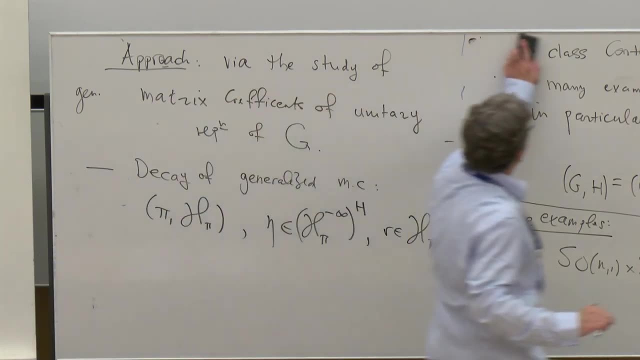 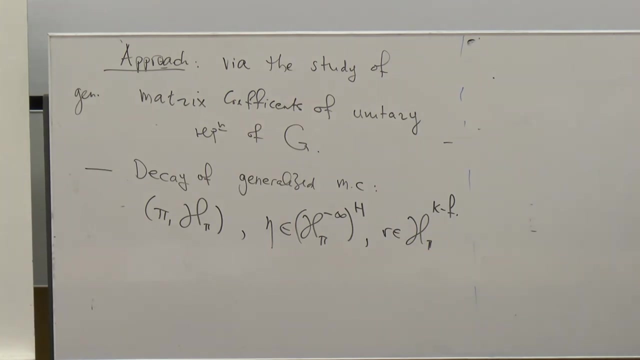 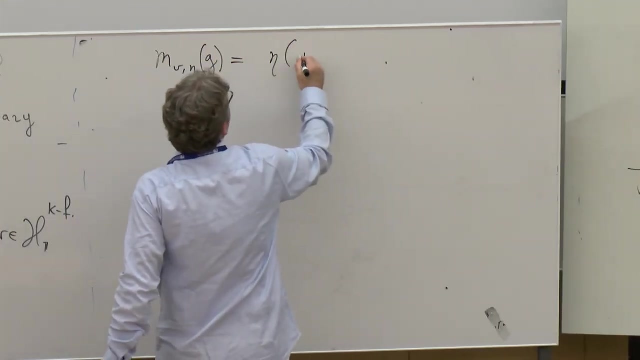 So I mean the setup of this G and h And V say a k-finite vector. Then one writes a function on G which descends to the space z. The function is the standard one. so m V, eta of G is equals to eta pi G. 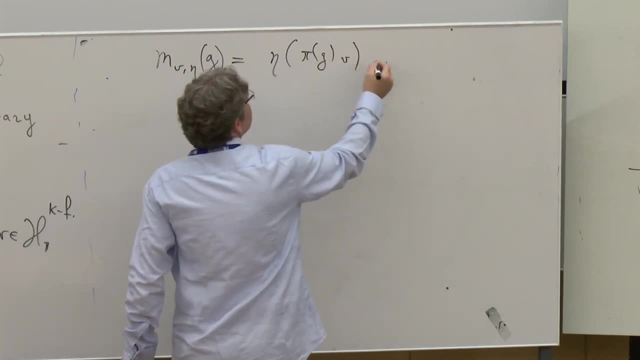 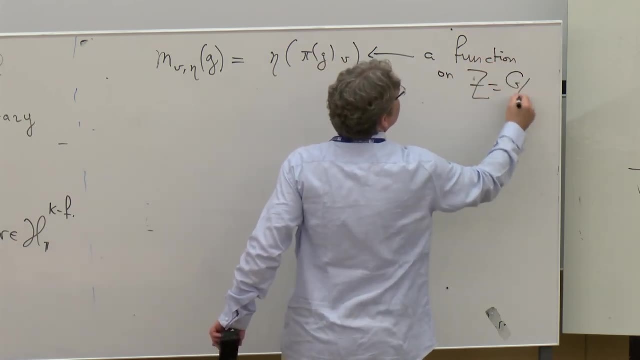 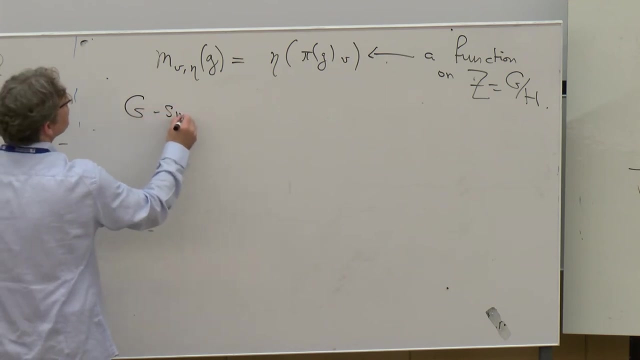 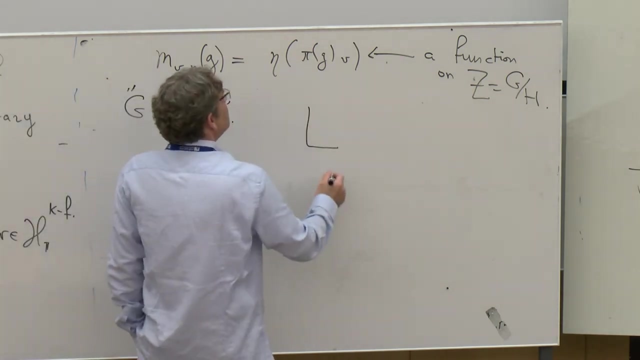 maybe G inverse of V. Okay, so this is a function on z And this function is really a smooth function. It is G smooth, So it means that it belongs to a space. let me, belongs to some function: space on z. 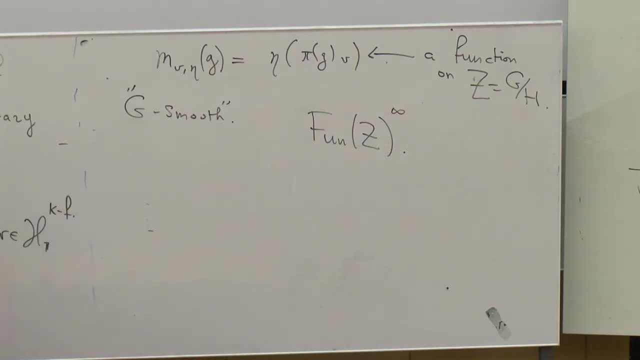 and it belongs to the smooth vectors. So starting point of the whole story, starting point was: we want to show that any function which belongs to L p of z and is smooth in fact decays at infinity. So if one analyzes the DRS argument, 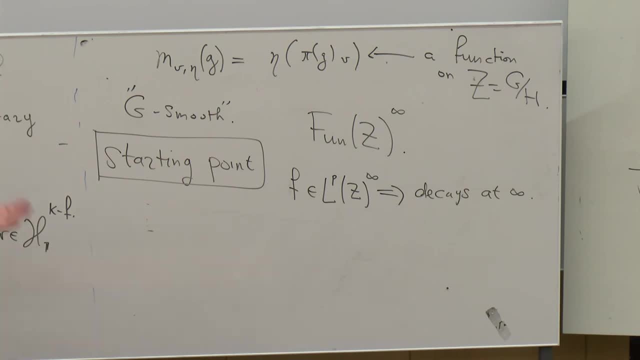 or in fact, any kind of harmonic analysis argument for the lattice counting problem. there is a beautiful double-fibration formula- which essentially is what people in automography call call unfolding- which allows you to calculate the number of lattice points in terms of H periods of automorphic forms. 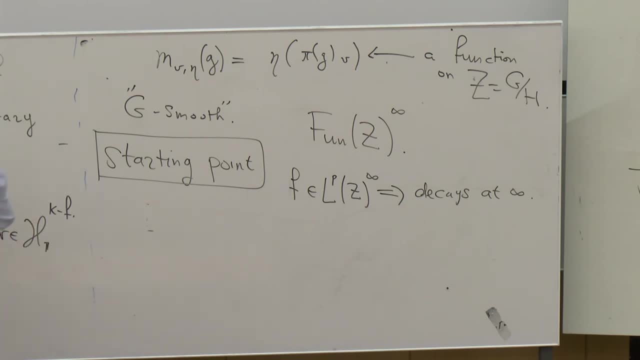 So, instead of studying H periods of automorphic forms, one decomposes this further using the automorphic plancherelle formula into matrix coefficients. So one needs to study the decay of matrix coefficients And then we prove the following theorem, which is completely abstract result: 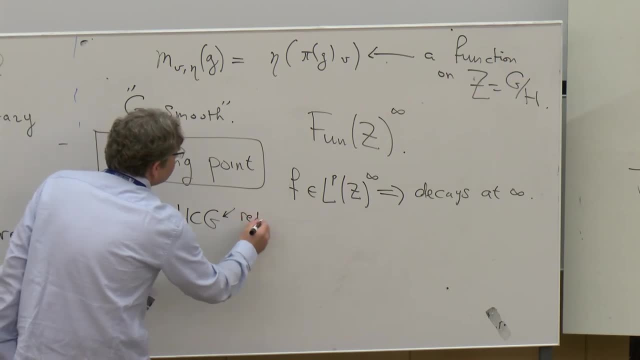 about H and G. this is say reductive let's, let's, for simplicity, say algebraic, and this is closed. And then we ask ourselves: when is it true that L, p, z, infinity, this means the infinity, means smooth vectors. 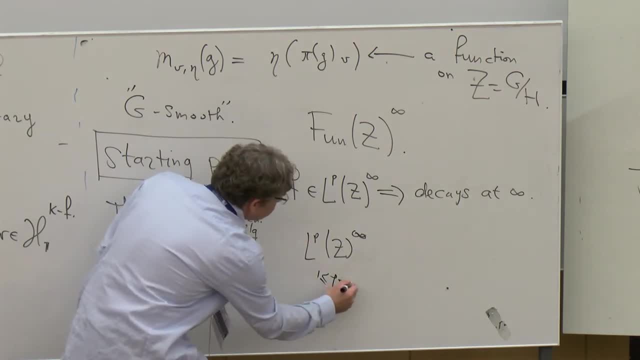 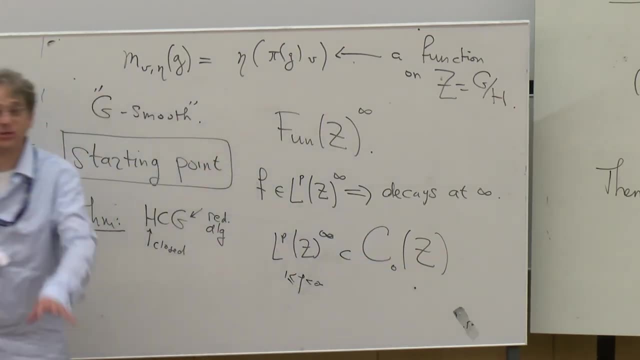 and p here is more than one and more than equal to one, less than infinity. when is this contained in functions on z which decay at infinity? This is just a notation for functions that outside a certain compact set become less than epsilon. 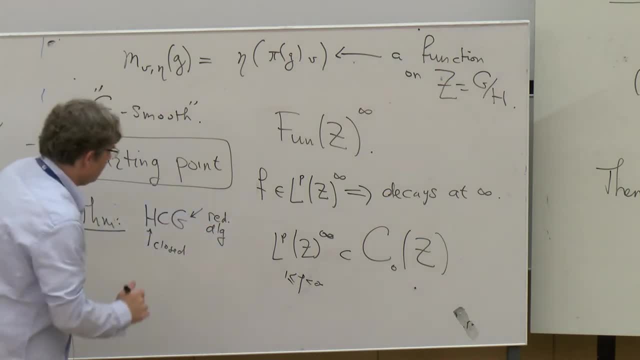 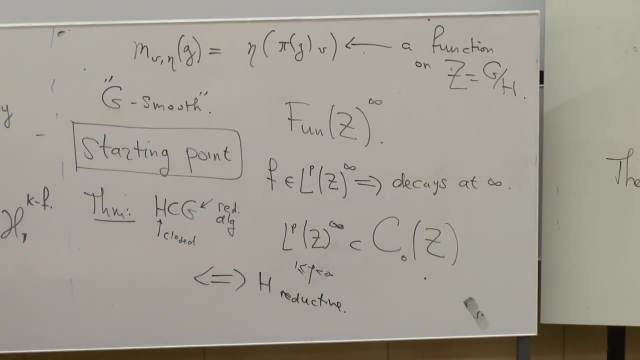 So you give the epsilon, I give the compact set. So we found out that this happens if, and only if, H is reductive. So the DRS argument can run in some way only if you study reductives of groups of G. 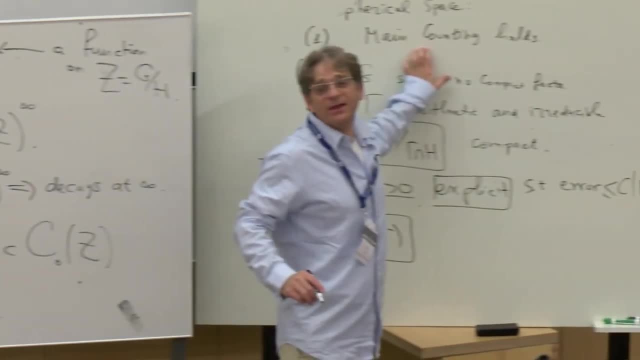 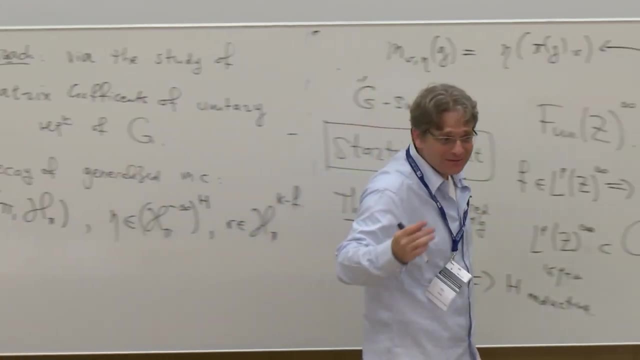 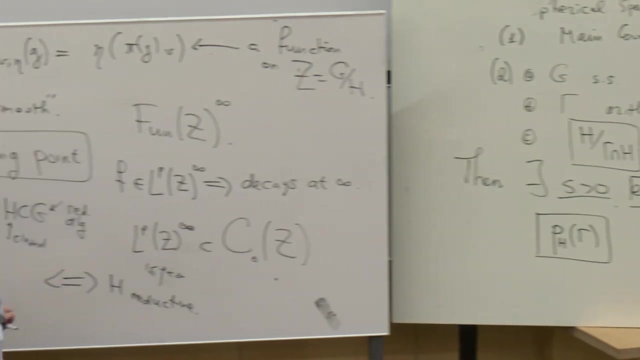 So this actually gave us main term counting using analysis. As I explained, today we have a completely different proof which avoids any analysis based on this geometric idea. But if one wants to run the error term analysis, one needs to have an explicit way. 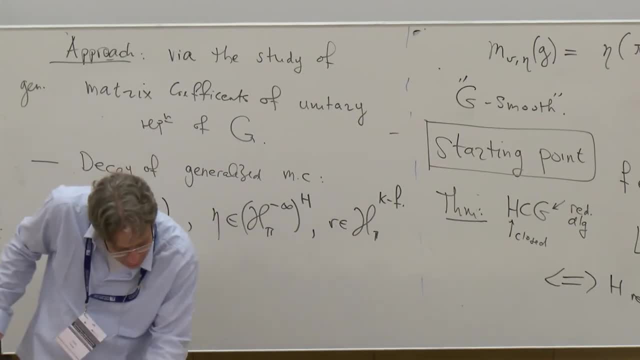 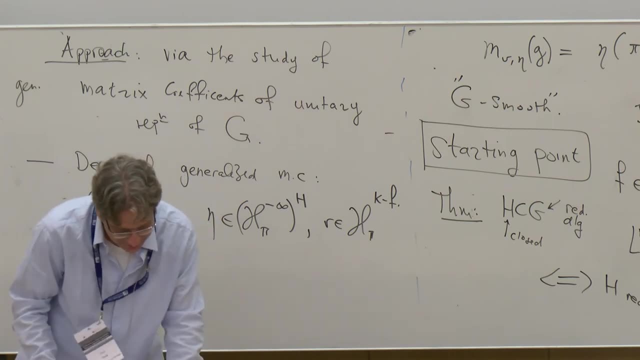 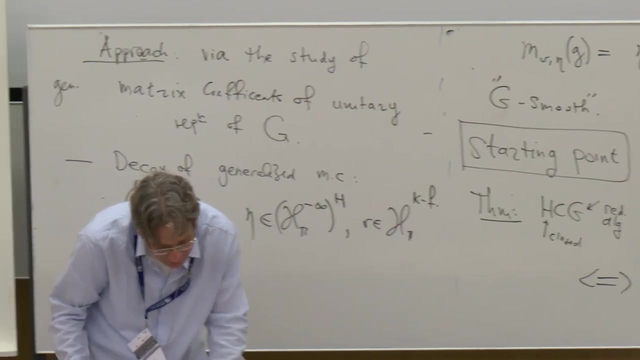 explicit control on the decay, And for that we so, since I have only five more minutes and I wanted to mention this, and so, thank you, Siddhartha. I think this is the right time. I mean, I see no other good time. 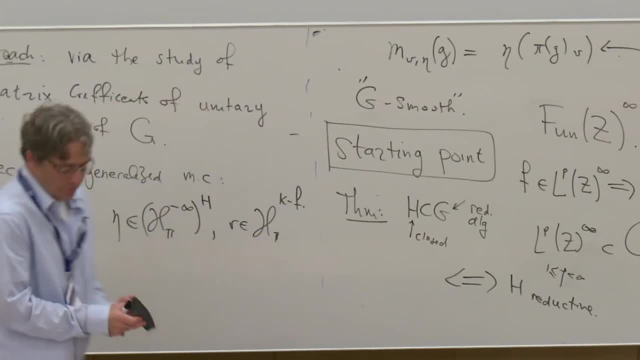 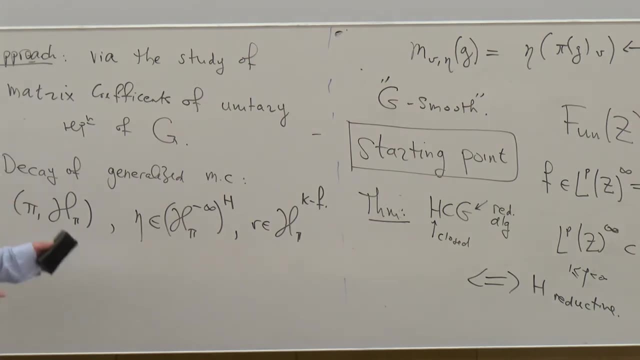 to mention that the key to the proof of this result was the paper by Joseph Bernstein, which Erez didn't mention, on the plancherelle formula. So I think, if you will give me one more minute, I will just mention this result. 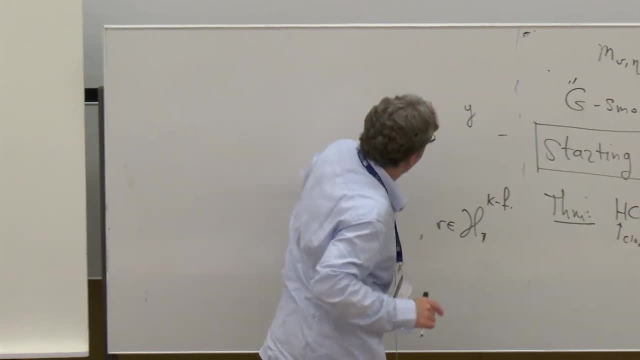 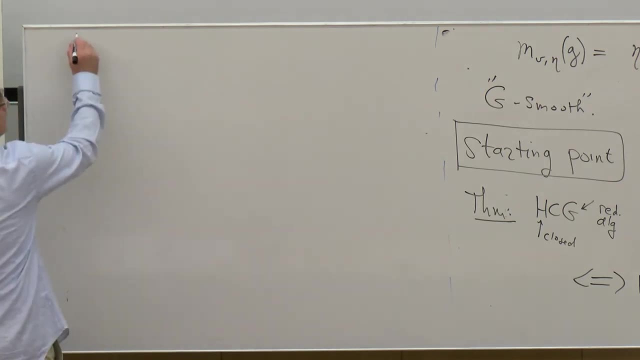 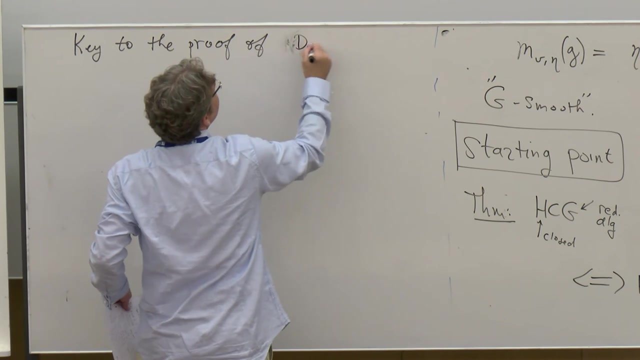 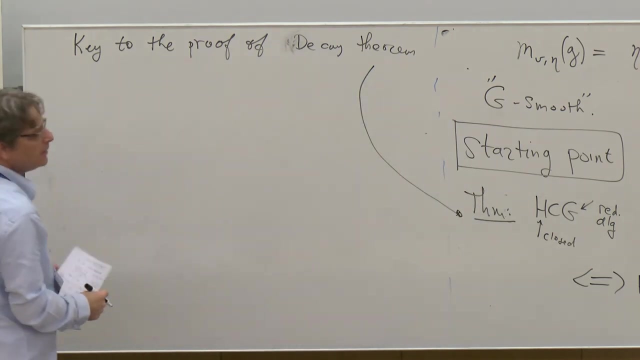 it's a beautiful result which I think deserves further audience. So P to the proof of of the decay theorem, this theorem, so it has two sides. it's relevant for one of them, so it's relevant for the side that we thought we proved. 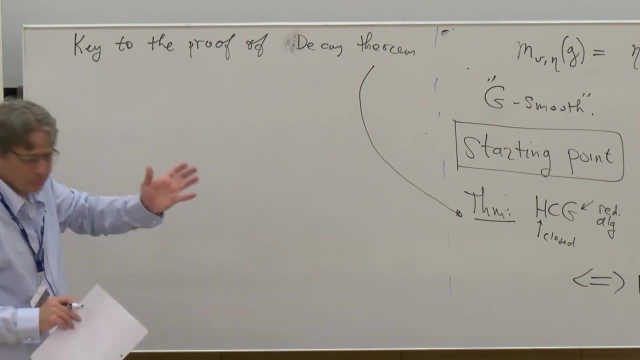 after we understand- and it took us a few years to understand that this was completely. it's not going to work until we understood better what's happening in Bernstein's paper. So this is the notion of what's called weight. 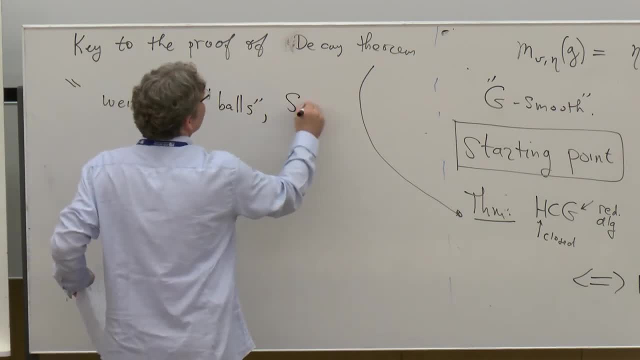 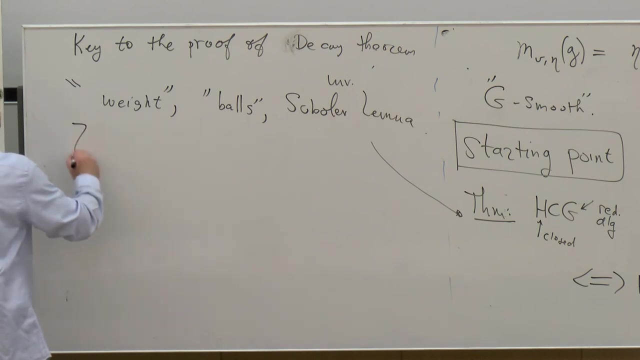 balls that you've already seen. and Sobolev Lemma- invariant Sobolev Lemma. So all this is very simple. it's far from being in the list of the ten best, but it's certainly a gem. So 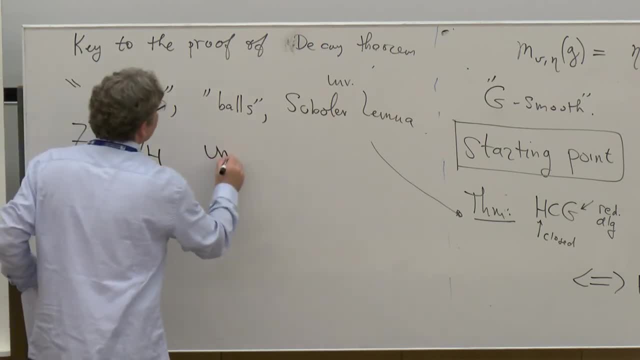 suppose that Z is a unimodular, homogeneous space. and suppose so, first of all we have a notion of a weight. so certain functions on Z which are a positive value are called weights. I will say the definition because I don't have enough time. 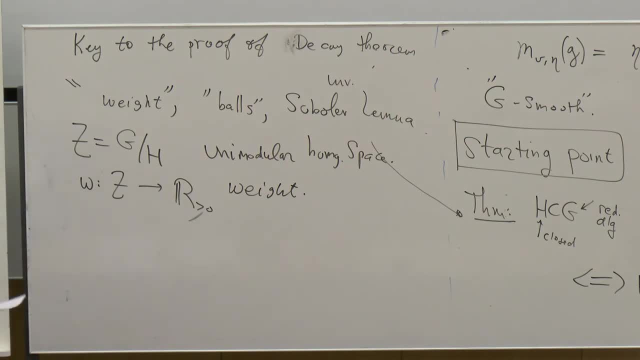 it has to be locally bounded and it has to behave nicely with respect to the action of the group, namely- I'll just say the second thing- with not the locally bounded, for every compact subset, if you compare omega of GZ. 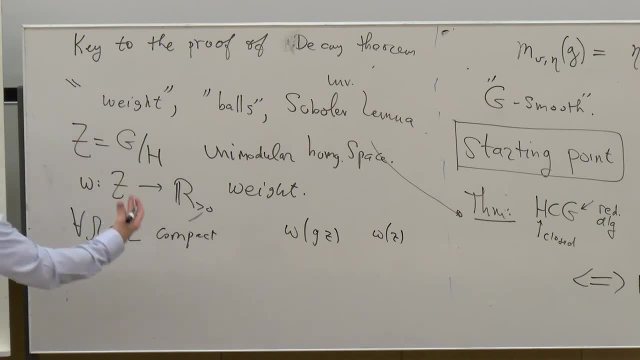 and omega Z. on that subset the comparison is in favor. so I mean, you don't ask for continuity here, so you need to to ask something. so you want some comparison of this form which holds at least in this compact. 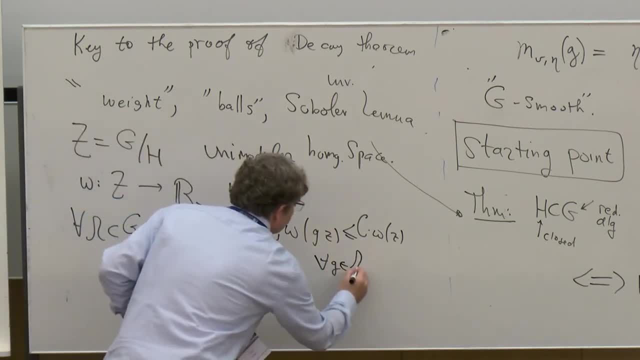 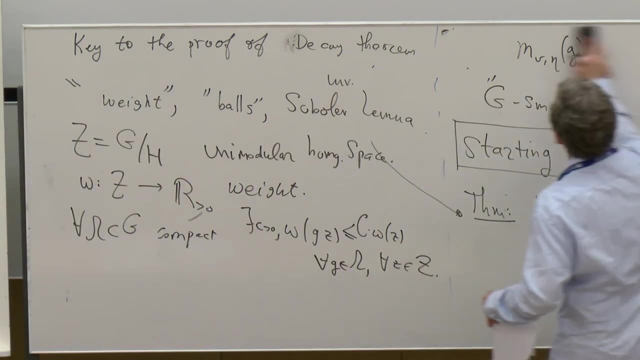 I made a mistake. it's compact Z in G, but for every Z in Z, so this is called a weight and there is a technology technology to produce weights, technology to take a ball in the group G and to act on a point. 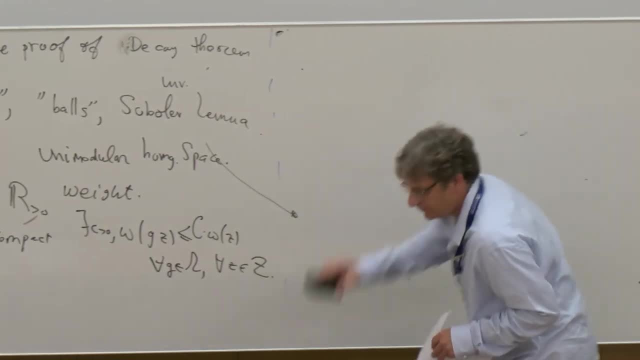 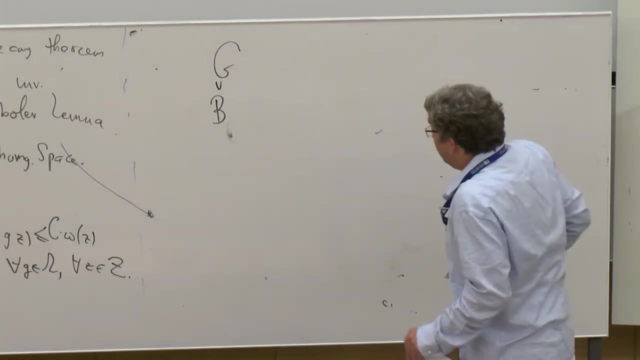 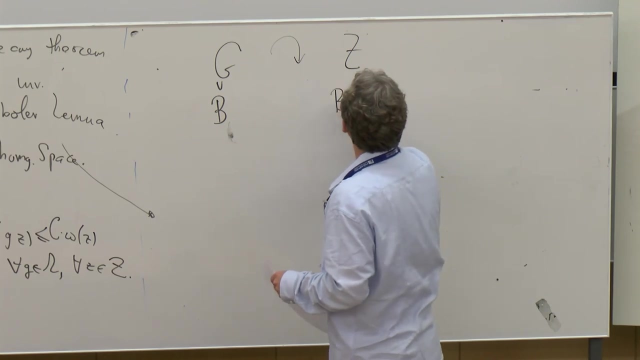 to look at the orbit of the ball on Z. so if this is G, you take a ball which is just symmetric, compact, subset around one, and you let it act on a point on Z. so in this way you create: 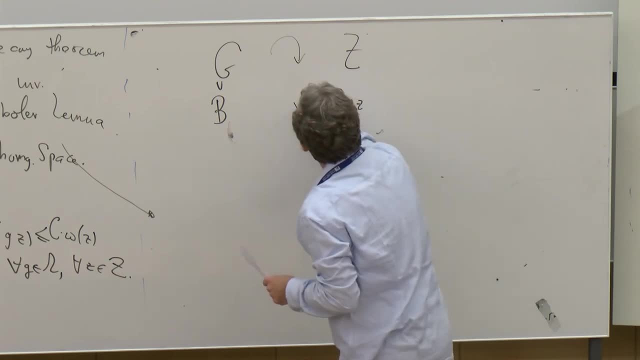 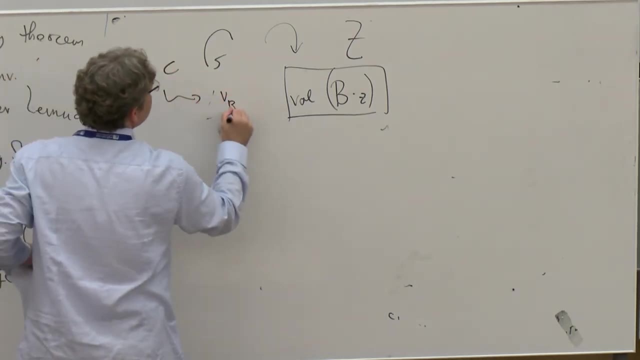 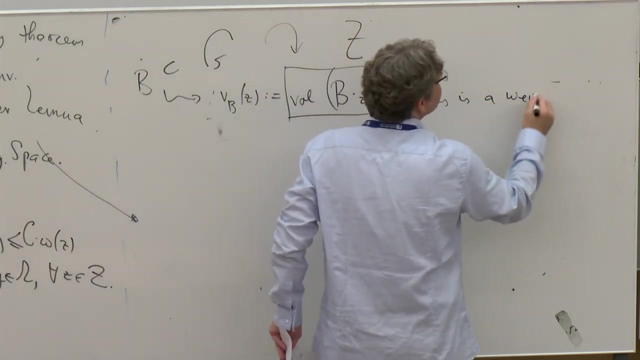 interesting subsets and if you take the volume, this gives you a function. so for every B you create VB of Z, which is this volume, and the exercise is that this is the weight and in fact it's easy to see that if you take two different balls. 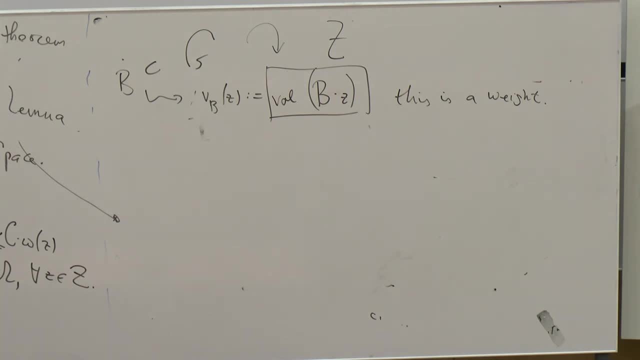 the two weights you get are comparable in an obvious sense. you make a definition and it works. and then the lemma which, with which I want to finish my my lecture, is the following, and it's absolutely crucial for us: suppose that you fix a P. 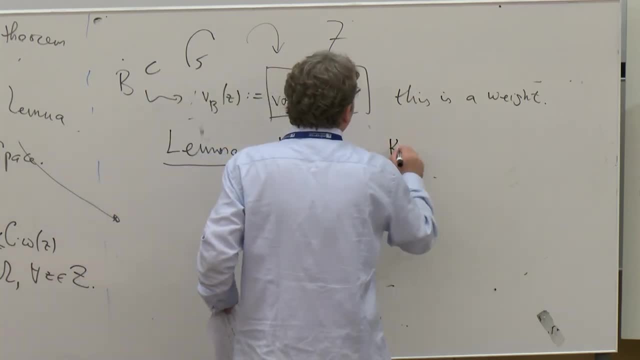 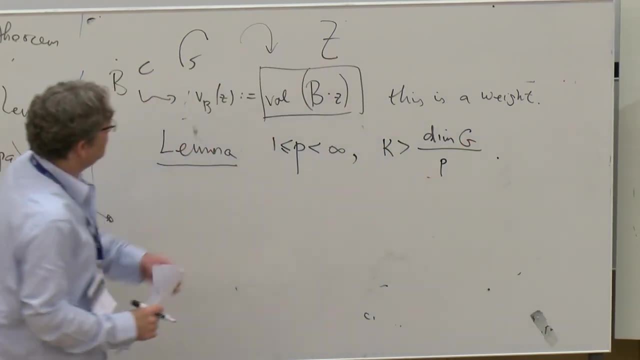 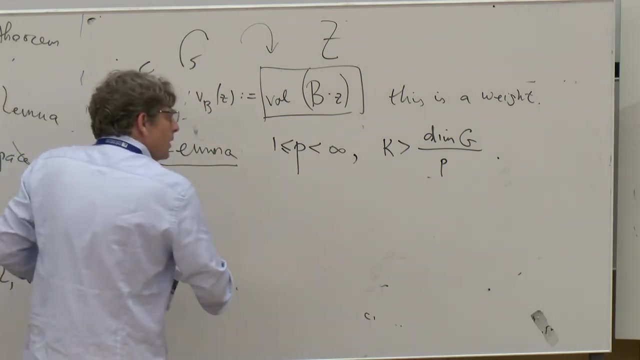 which is between one and infinity, and you take K, which is bigger than the dimension of the group divided by P. okay, so you fix a P because you are going to work with LP functions. Joseph worked with L2,, but this is okay. 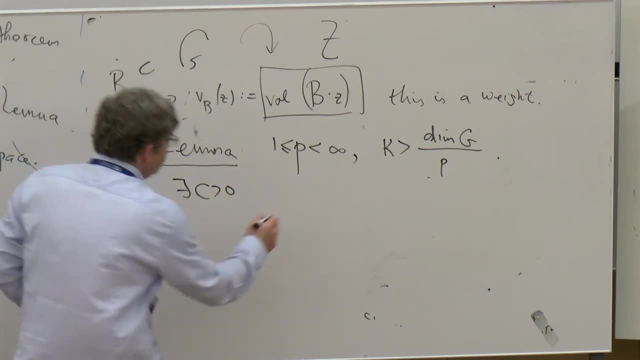 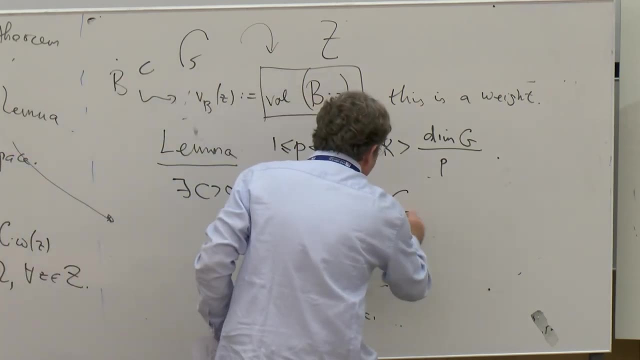 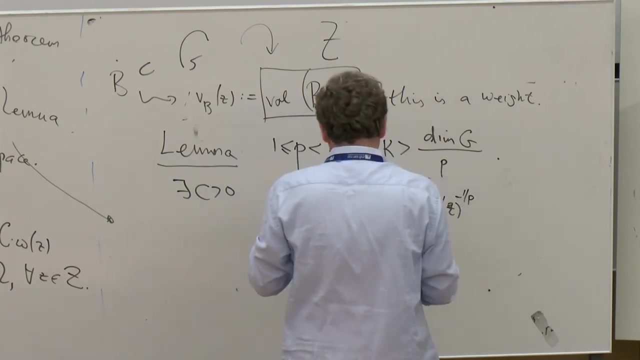 then there exists a constant C, with the property that the point of evaluation, at every point, is dominated by some constant times. the volume of this ball to some power, which is minus one over P times the LP Sobolev norm. 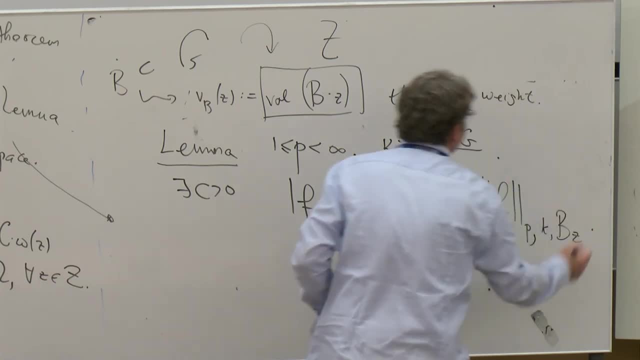 so you need to take K derivatives restricted to this compact set, BZ. Okay. so maybe it's difficult to appreciate this, but the idea is that in the regime of a group action, you can make the local Sobolev inequality. 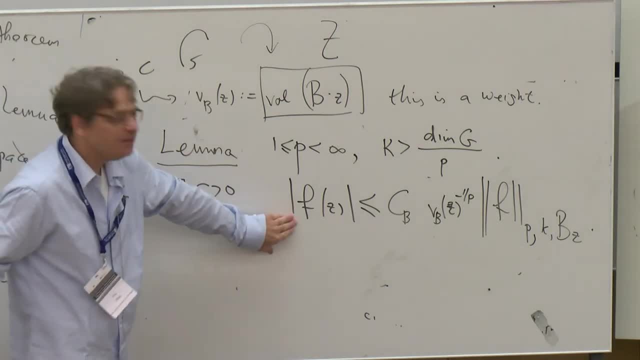 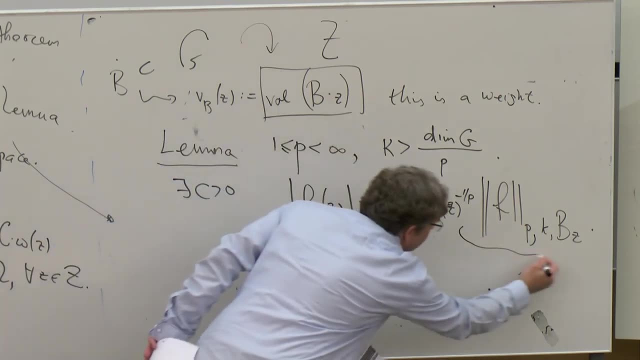 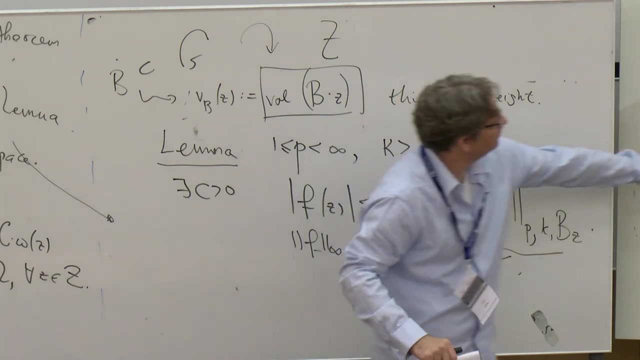 sort of global, because, effectively, here you have an L infinity bound on a function, you have an L infinity bound of the function on Z in terms of its LP norm. and to finish, it turns out that to get this result, 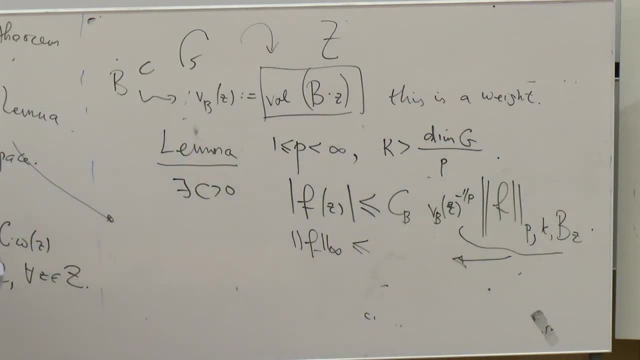 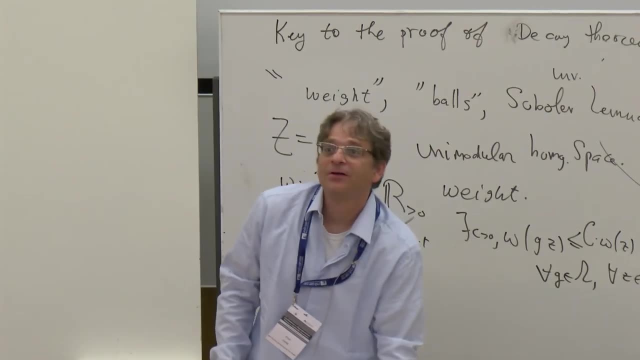 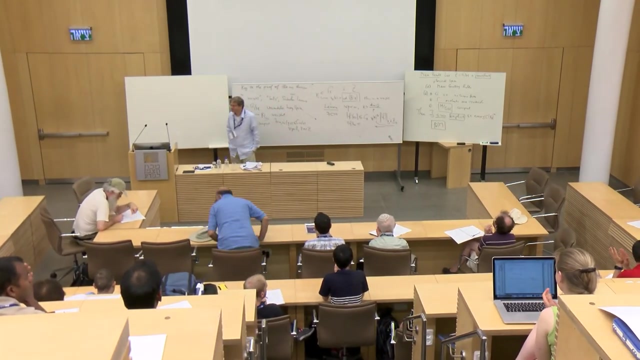 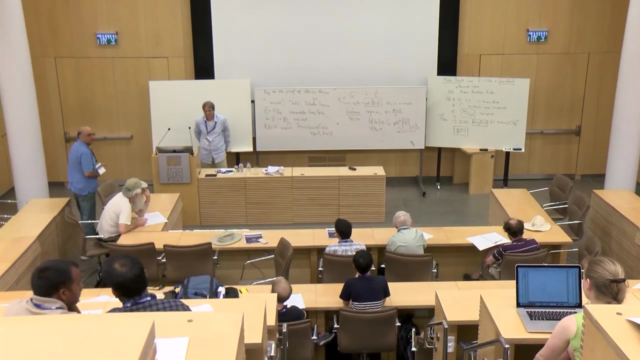 we need to have a converse to this inequality and this is based on a recent work of Patrick Delorme and company on constant terms of input functions on spherical varieties. Okay, thank you very much for your attention. Questions: 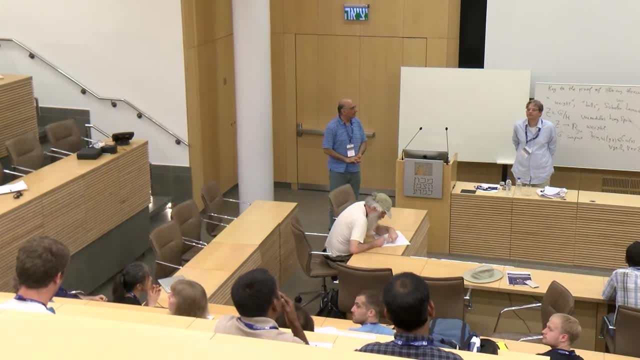 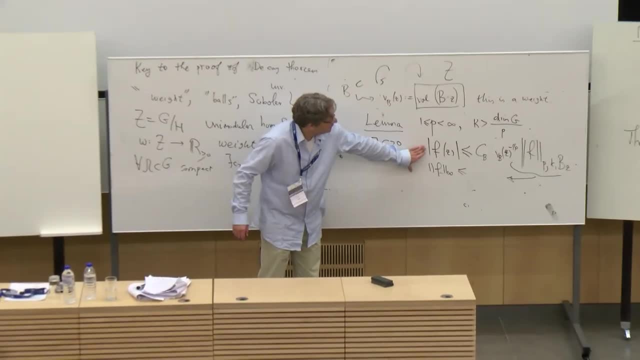 For that test do you need an explicit degree rate of the matrix coefficient, the effective degree of the matrix coefficient? Yes, so in fact, such an inequality, such an inequality gives you such a decay because of the volume, So what? 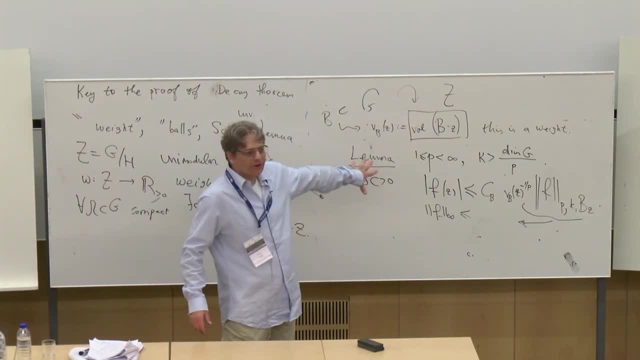 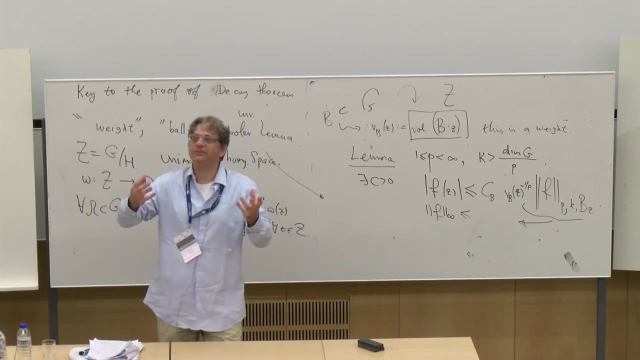 this is a general fact. you can prove this for any reductive homogeneous space. but on these spherical spaces, because they have a kind of data, you can study them using linear algebra. in some sense you can calculate. 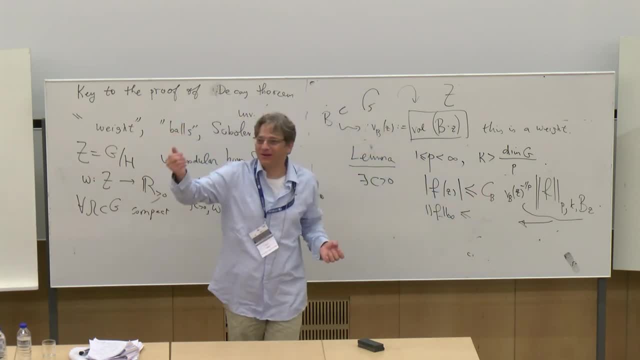 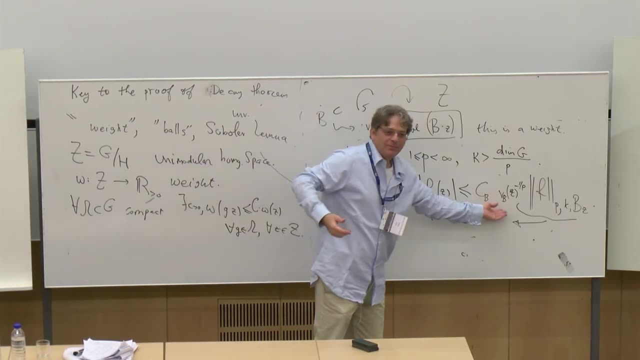 the volume of these balls. In terms of the combinatorial information, you get some kind of a to the minus two rho, a corresponding rho. So this gives you a possibility to prove two things: First of all, that they are in some LP. 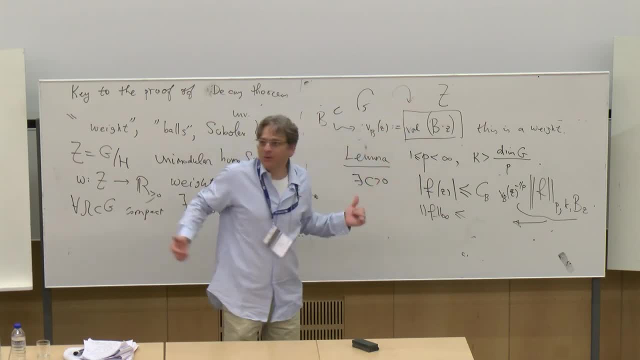 which is not obvious at all. After they are in LP we know by our general result that they have to decay. This already gives counting. But if you want to actually control how much they decay you need to know that all of them are in the same LP. 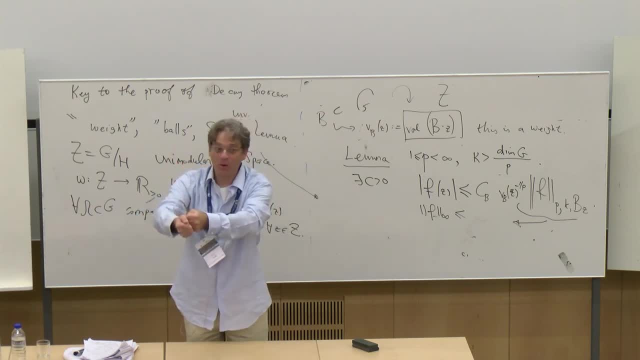 in some sense You need to have a P to put them all, And this is somehow the role of this guy. This is not an assumption, because people have been able to prove that such an exponent exists for particular gammas. 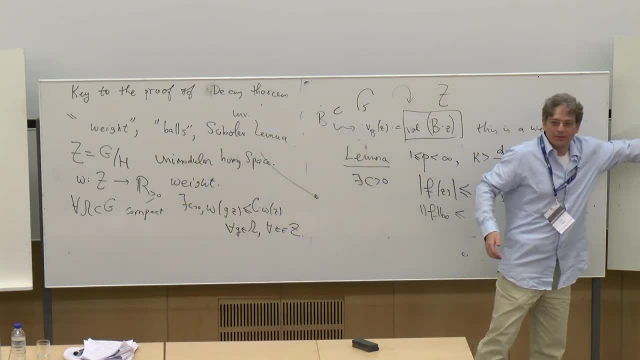 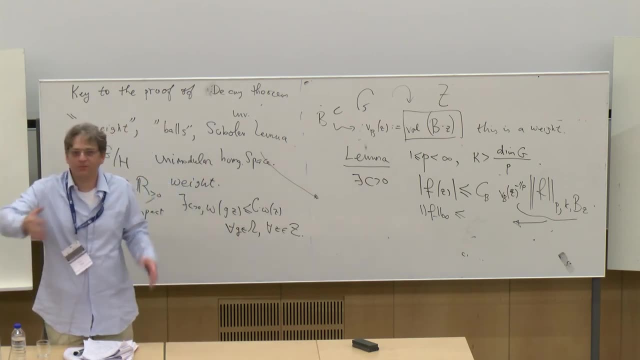 For some classes of gammas, in particular the ones I mentioned here. I'm hiding some other information that we are using some bounds and multiplicities in the space of automorphic forms, etc. So all these things are really deep. 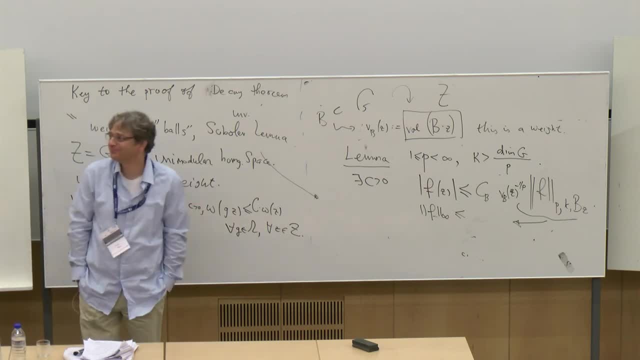 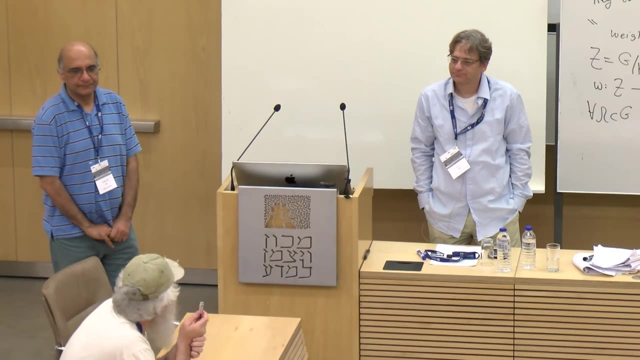 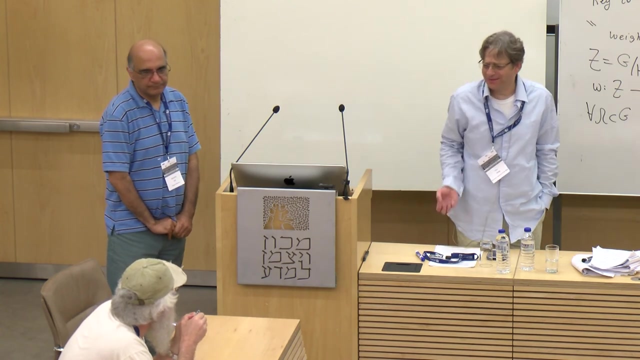 but they are already known. So the question is for the error term, are they related to a retic continuation or some kind of detail or something? No, I think it's much less. I mean it's not as deep as that. 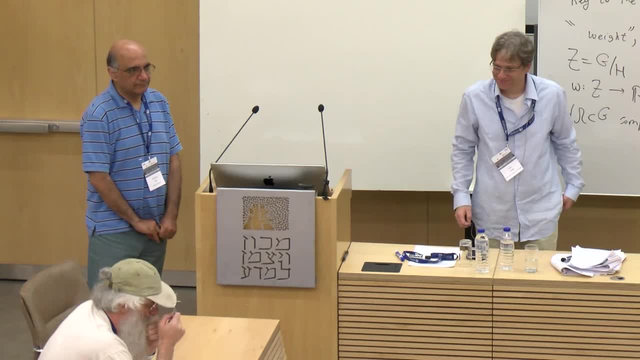 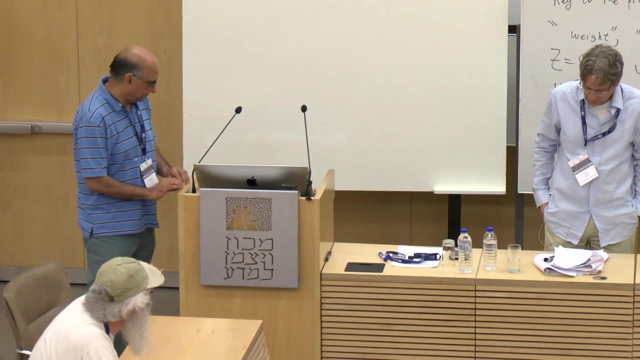 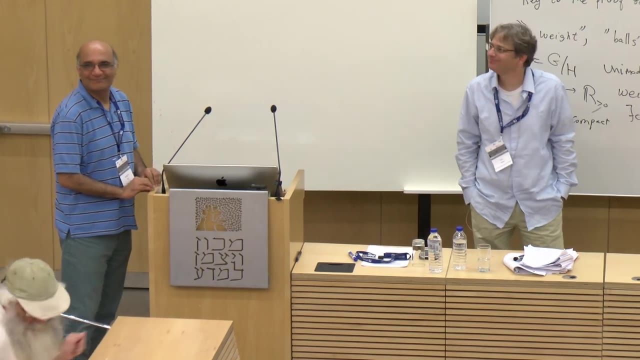 It's not. we don't touch this nerve, But is it expected that some kind of a, you know, morphic continuation is going to work eventually? I don't know, It's beyond my competence. Can you give us an example?